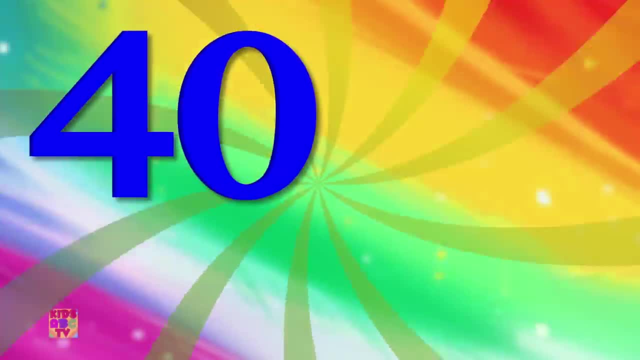 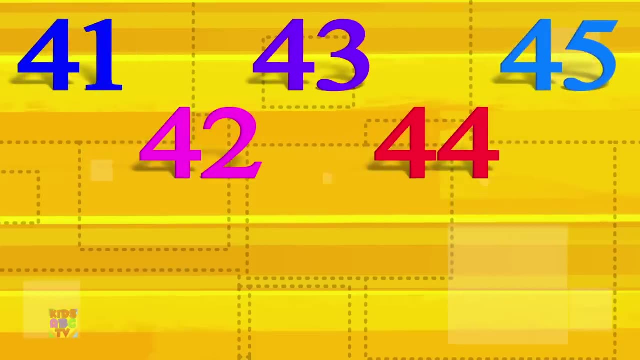 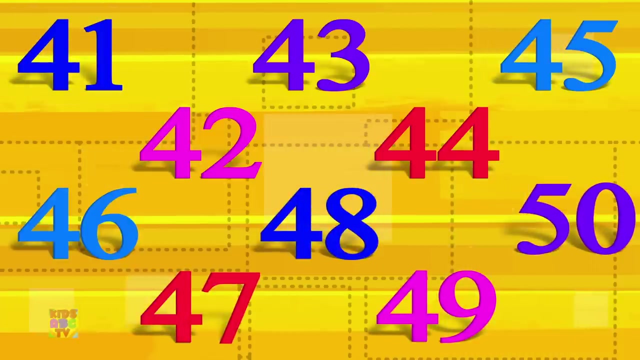 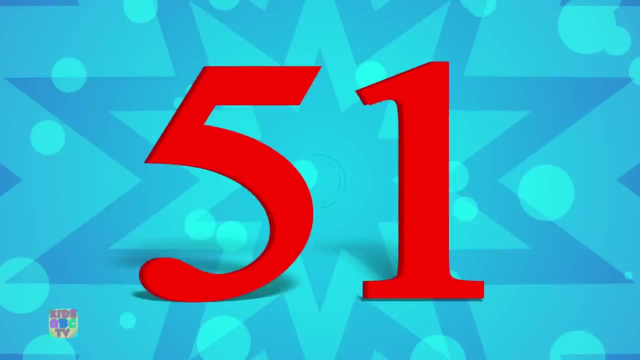 40,, 40,, 40,, 40, 41,, 42,, 43,, 44,, 45, 46,, 47,, 48,, 49,, 50, 50,, 50,, 50, 50, 51,, 52,, 53,, 54, 55. 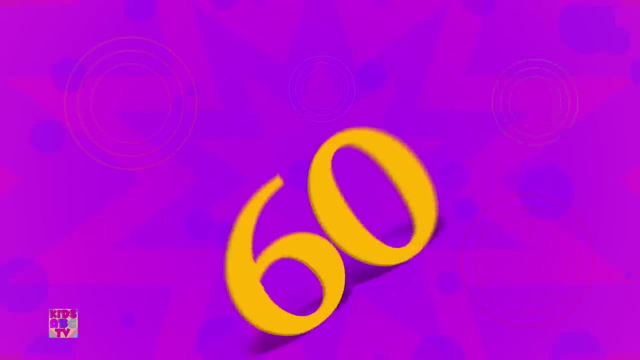 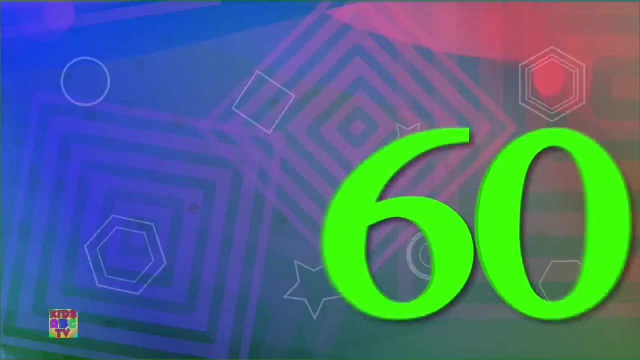 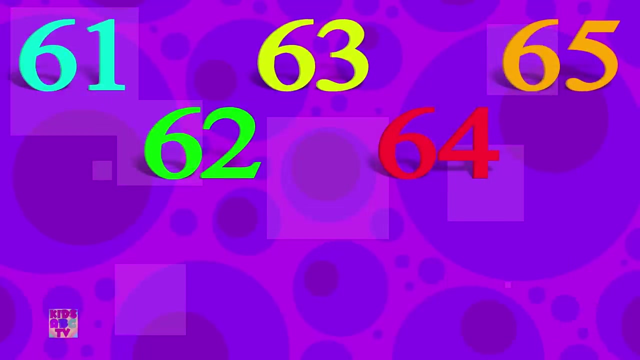 56,, 57,, 58,, 59,, 60, 60,, 60,, 60, 60, 61,, 62,, 63,, 64,, 65, 66,, 67,, 68,, 69, 70. 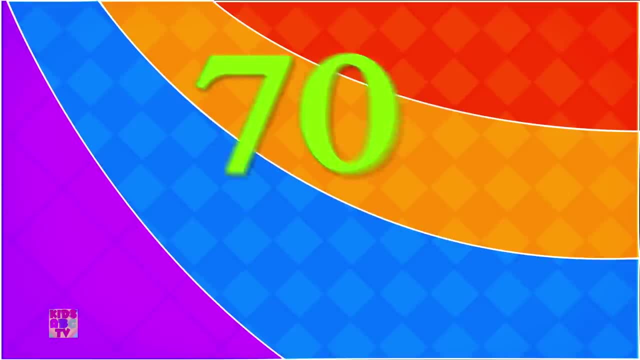 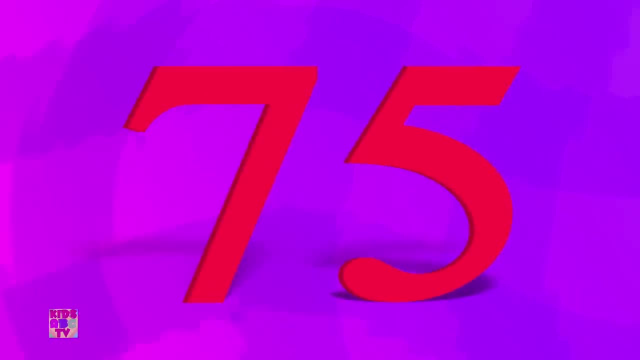 70,, 70,, 70,, 70, 71,, 72,, 73,, 74,, 75, 71,, 72,, 73,, 74,, 75, 76,, 77,, 78,, 79, 80. 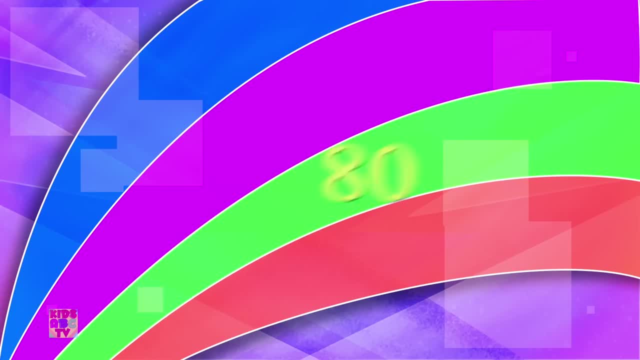 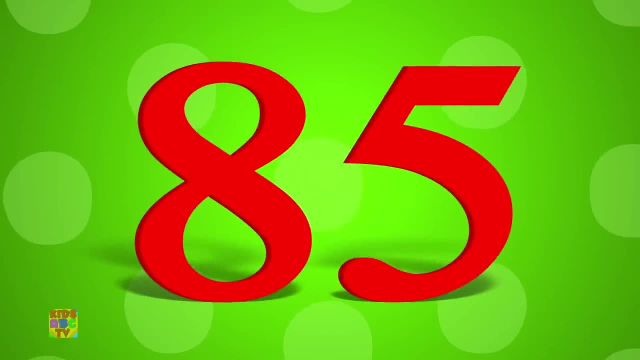 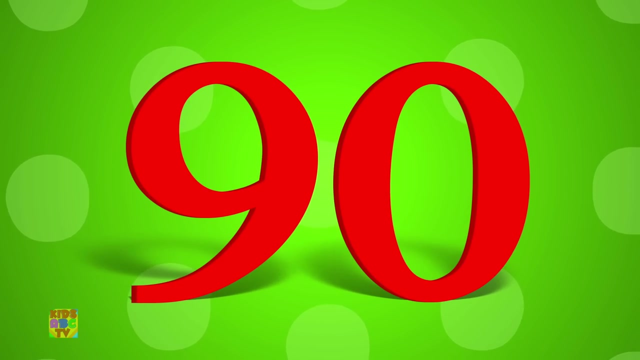 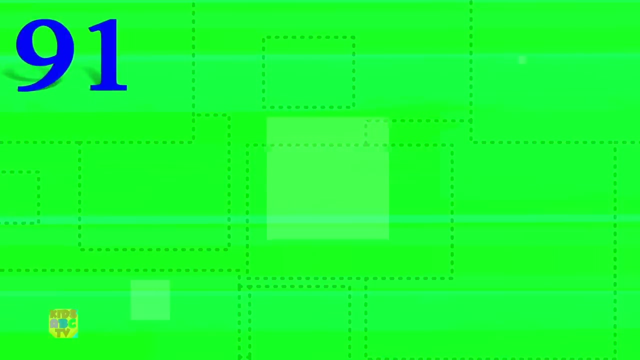 80,, 80,, 80, 80, 81,, 82,, 83,, 84, 85, 86,, 87,, 88,, 89, 90, 90,, 90,, 90, 90, 91,, 92,, 93,, 94, 95. 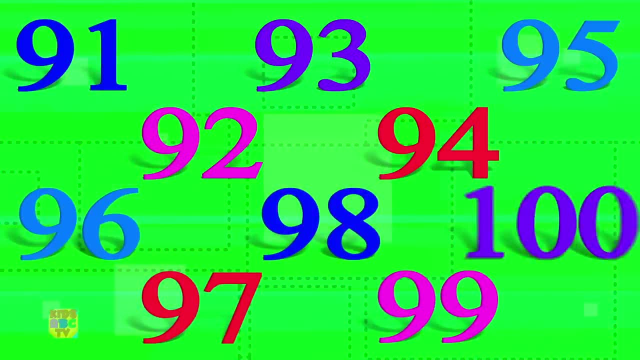 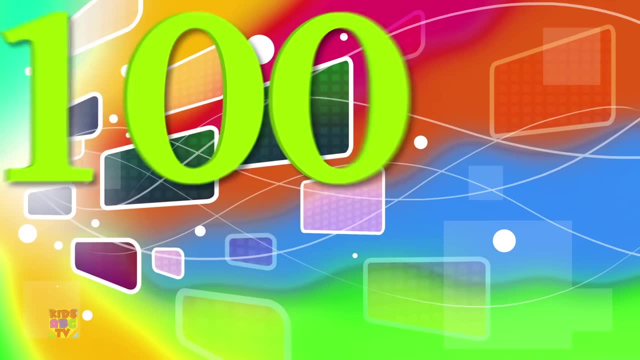 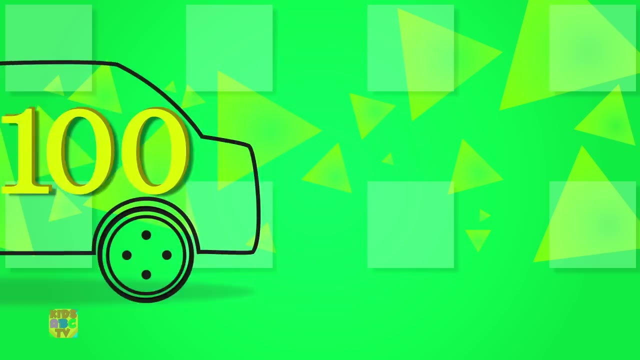 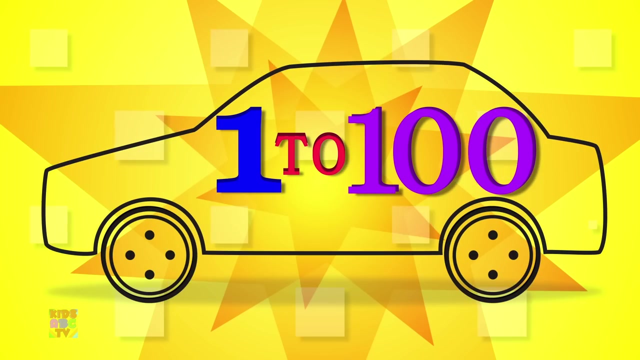 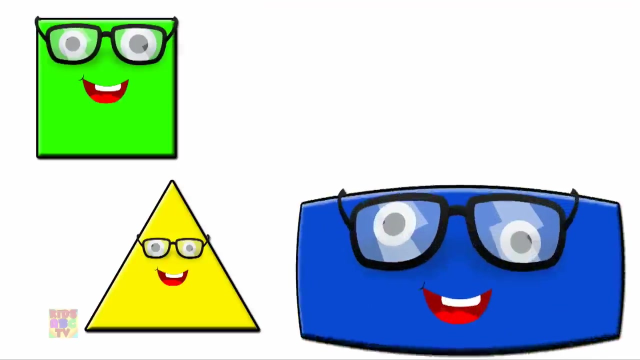 96,, 97,, 98,, 99, 100, 100, 100,, 100, 100. Here are your numbers 1 to 100. Here are your numbers 1 to 100. Seven, Two, Three, Four, Five, Six, Seven, Ten. 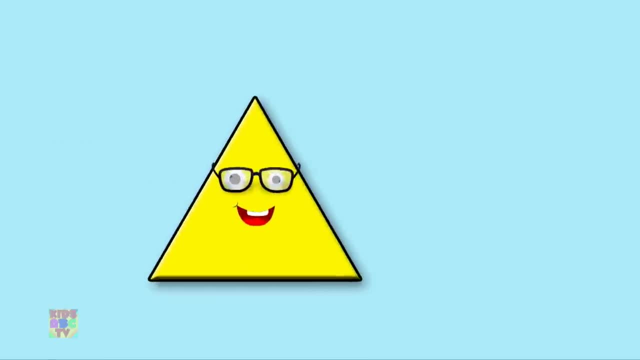 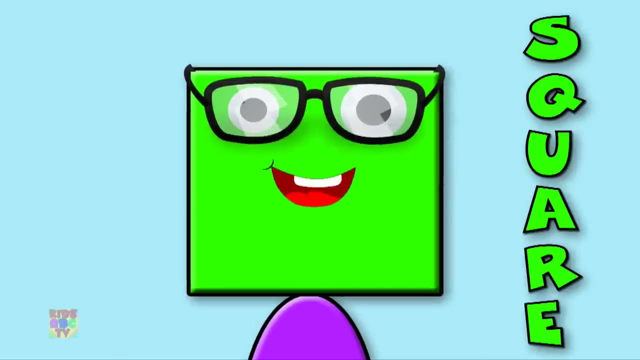 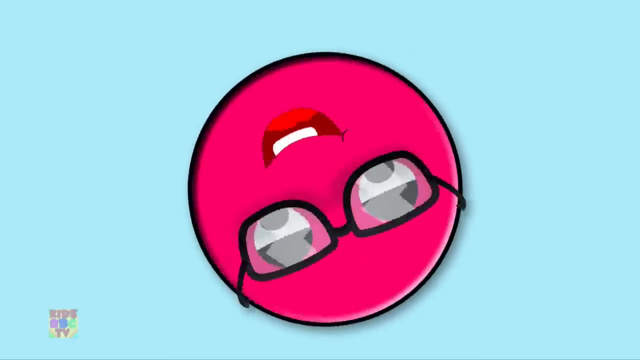 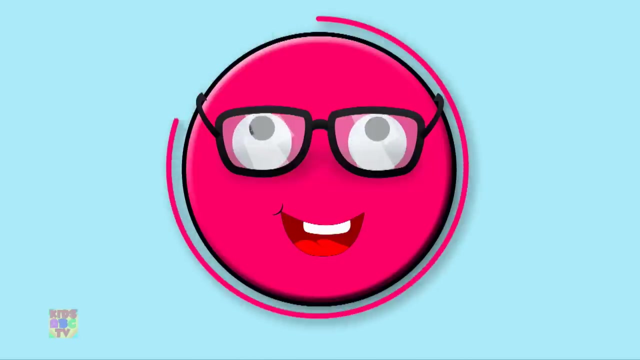 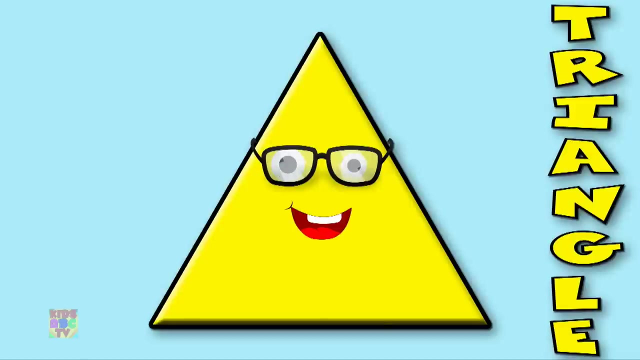 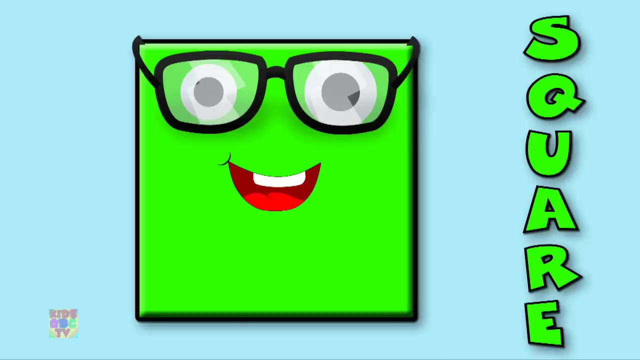 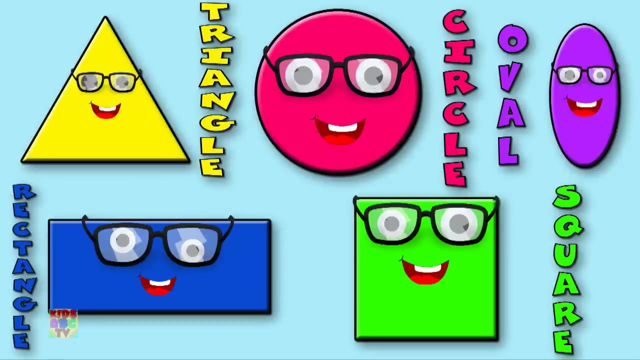 Nineteen, Nineteen, Seventeen, Eighty, Nine, Twelve, Thirteen, V calor One, Round and round, round and round. I'm a circle, Round and round and round and round I am. Triangle, rectangle, circle, oval, square. Triangle, rectangle, circle, oval, square. 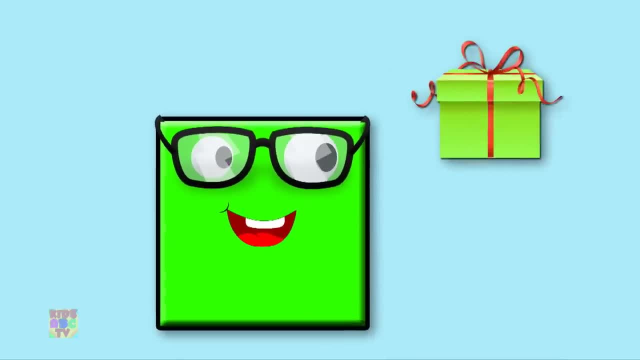 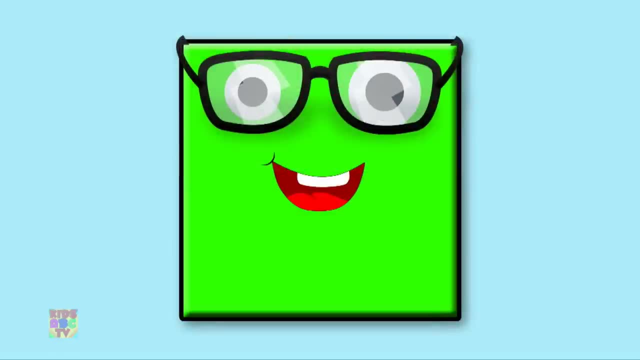 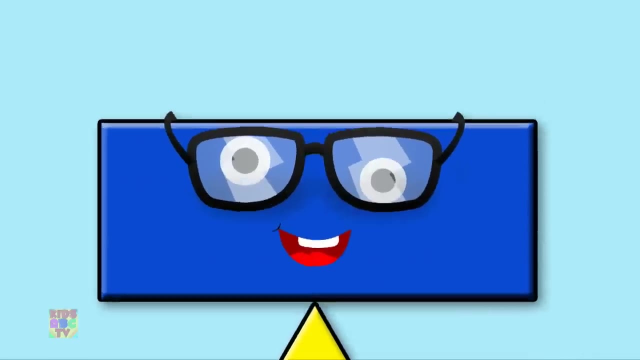 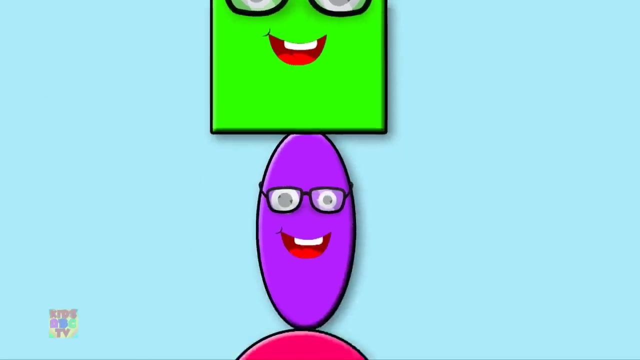 I'm a four-sided square Shaped like a box. I'm a four-sided square Shaped like a box. Shaped like a box. I'm a four-sided square And all four sides are the same. Triangle- rectangle- circle, oval square. Triangle- rectangle- circle, oval square. 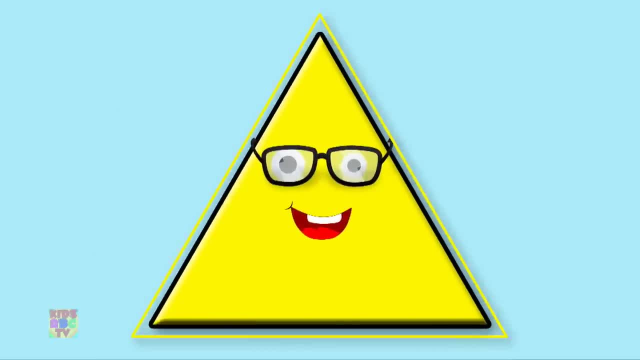 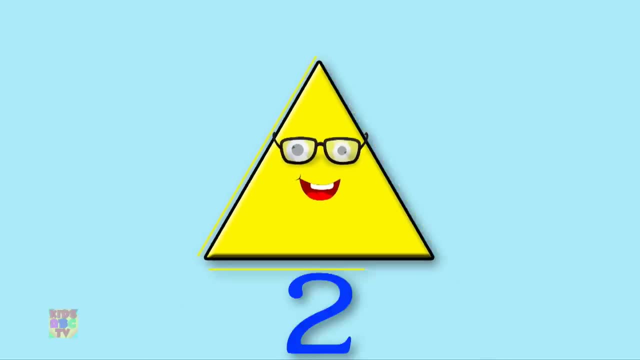 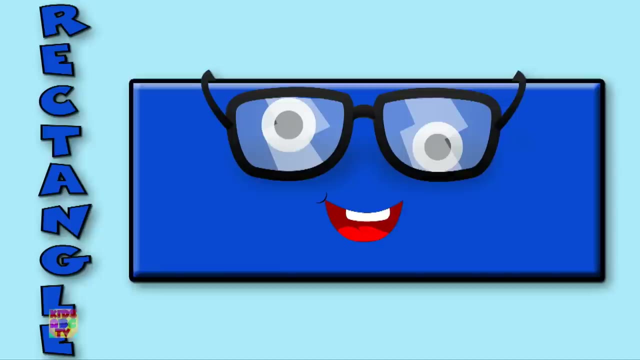 I'm a triangle with three sides, Three straight sides. I'm a triangle with three sides, Three straight sides, Three straight sides. I'm a triangle with three sides And a pointy head. Triangle, rectangle, circle, oval, square. Triangle, rectangle, circle, oval, square. 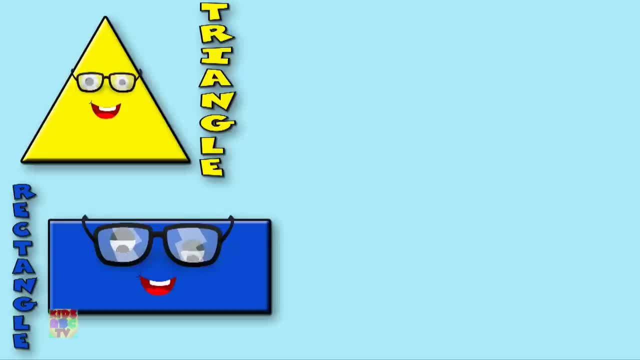 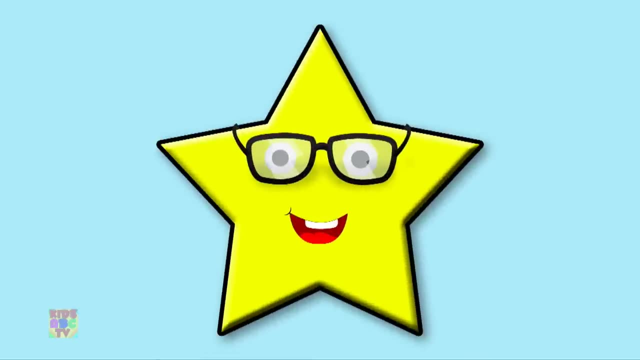 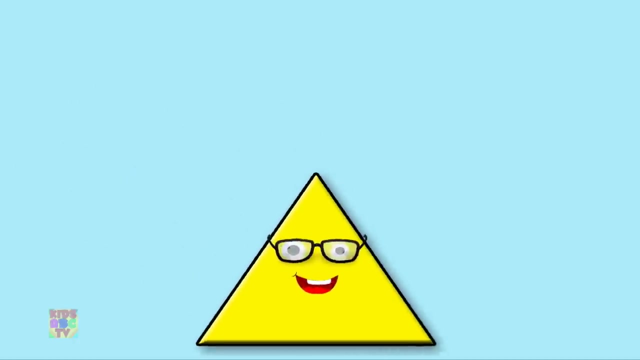 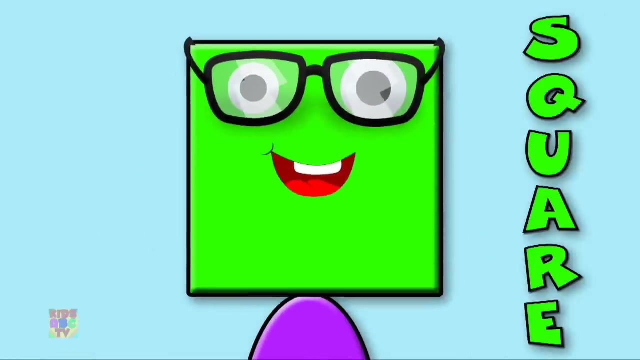 I'm a star with five points, Five little points. I'm a star with five points, Five little points, Five little points. I'm a star with five points Twinkling in the sky. Triangle, rectangle, circle, oval square. Triangle, rectangle, circle, oval, square. 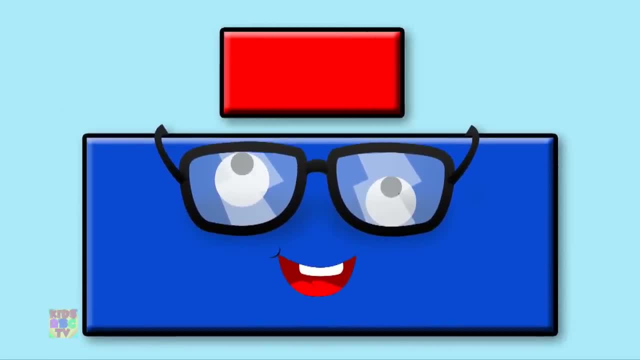 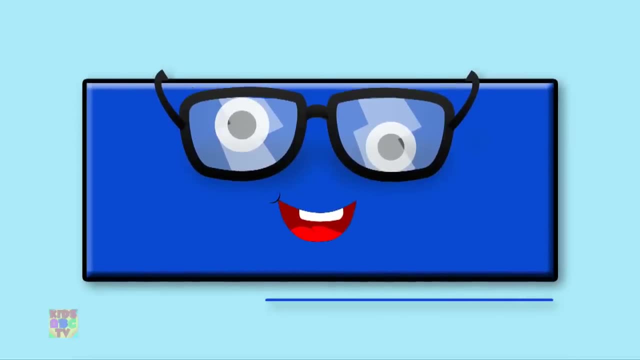 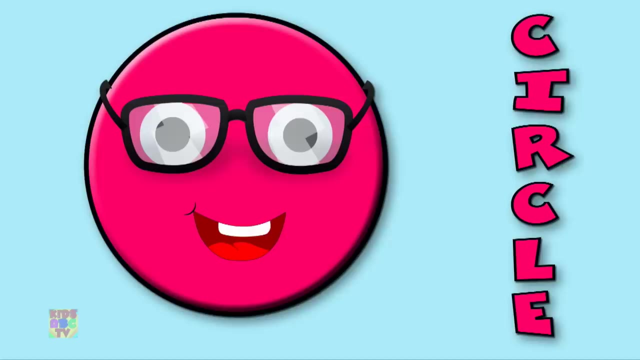 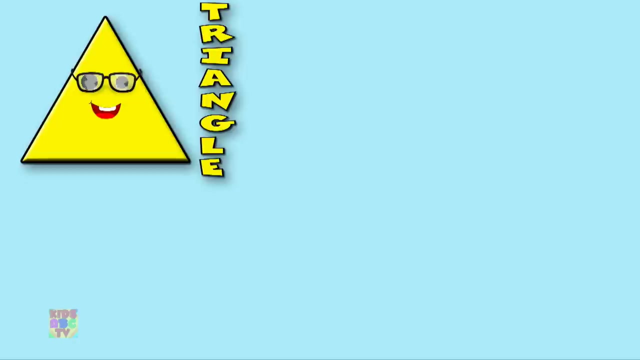 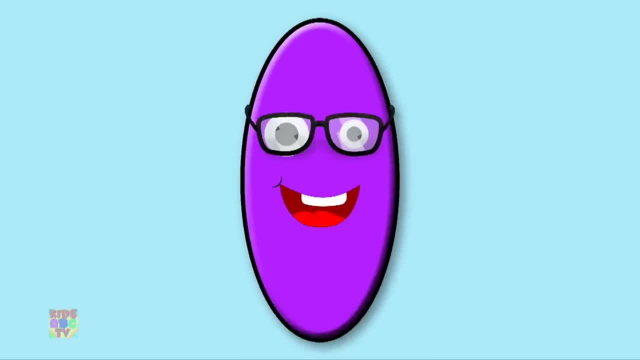 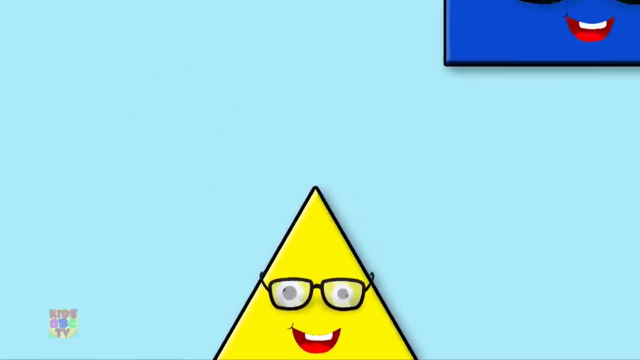 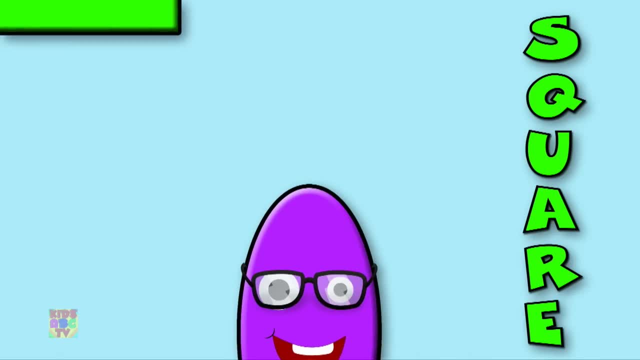 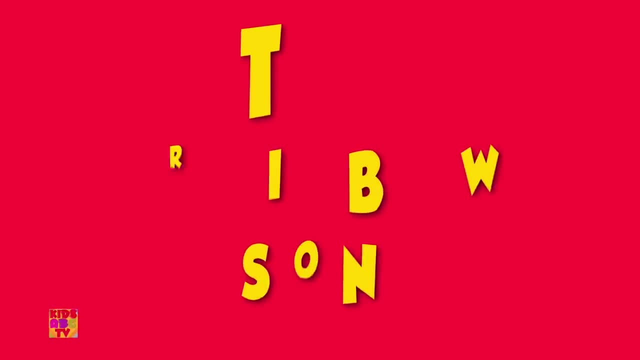 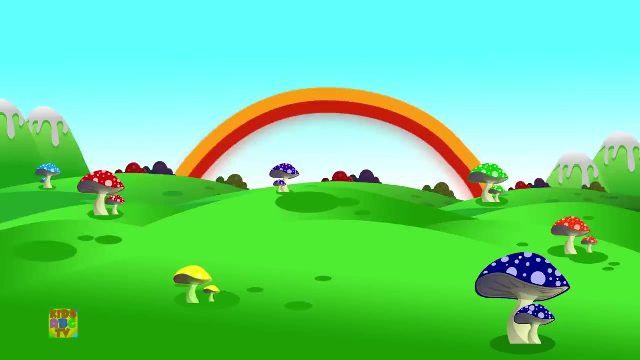 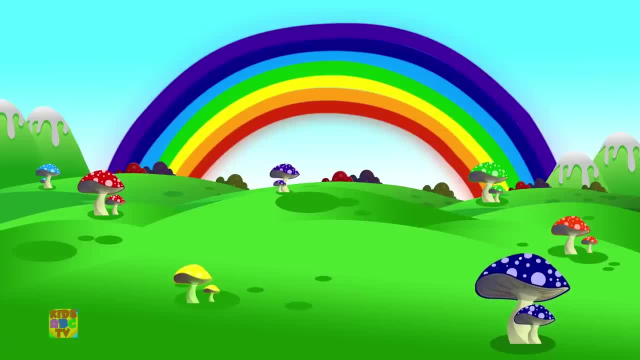 Red, orange, yellow, green: These are the colors of the rainbow. Blue, indigo and violet: These are the colors of the rainbow. Red, orange, yellow, green: These are the colors of the rainbow. Blue, indigo and violet: These are the colors of the rainbow. 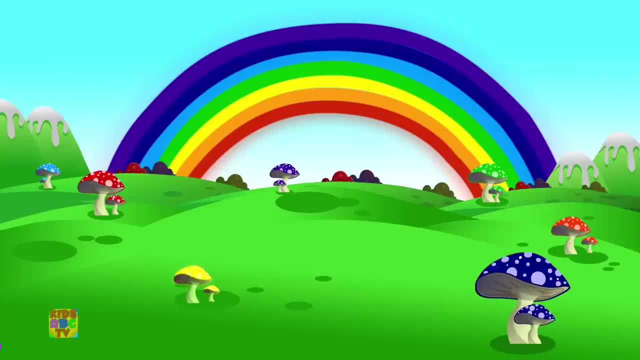 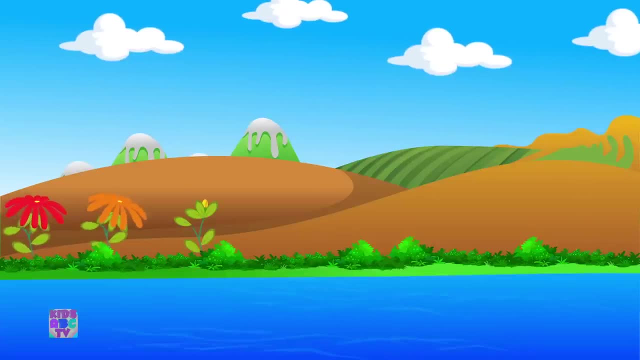 Blue, indigo and violet: These are the colors of the rainbow. Red, orange, yellow, green: These are the colors of the rainbow. Blue, indigo and violet: These are the colors of the rainbow. Red, orange, yellow, green: These are the colors of the rainbow. 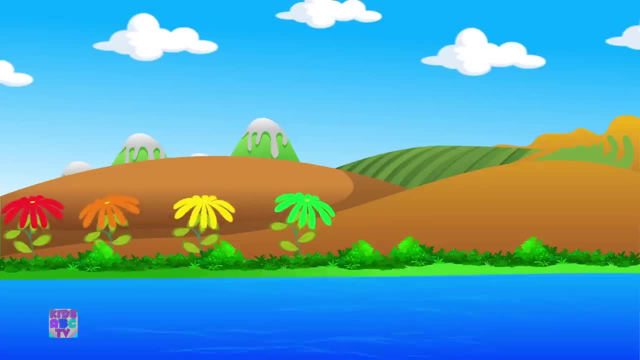 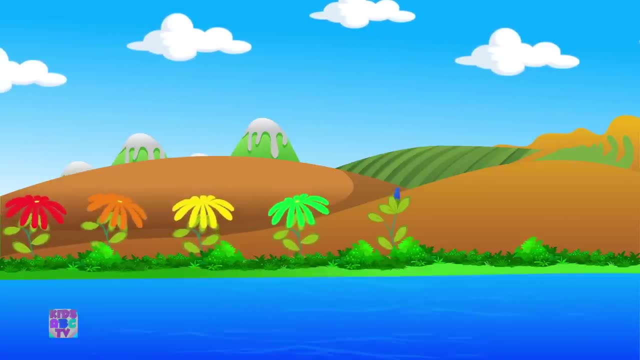 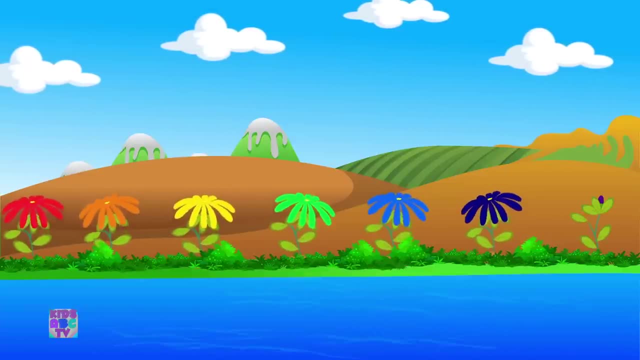 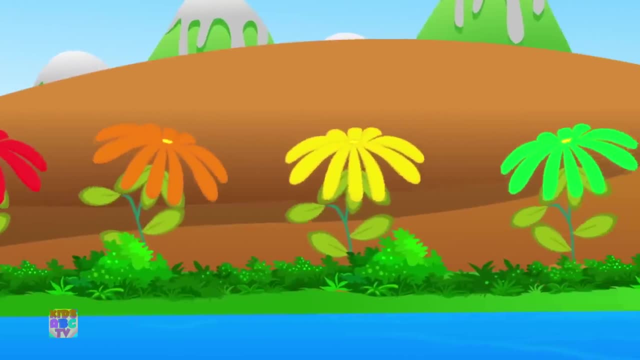 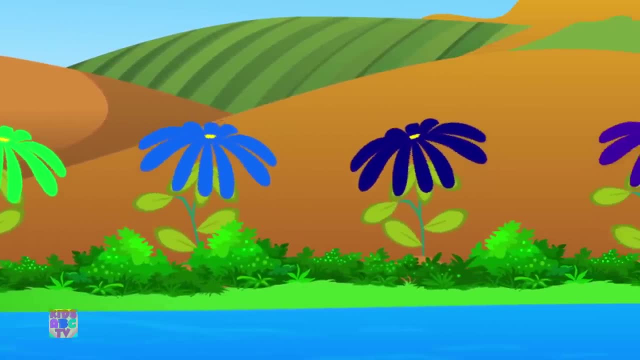 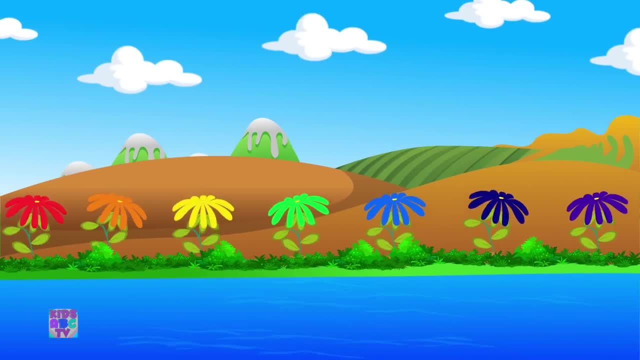 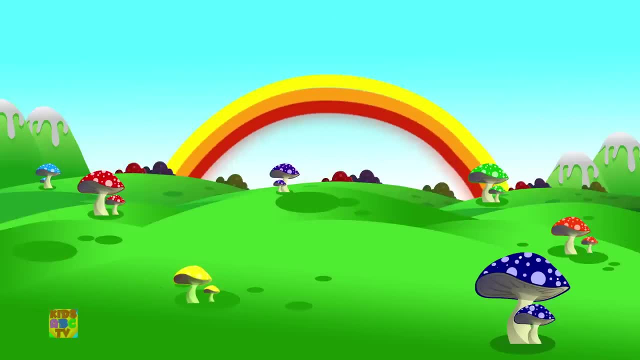 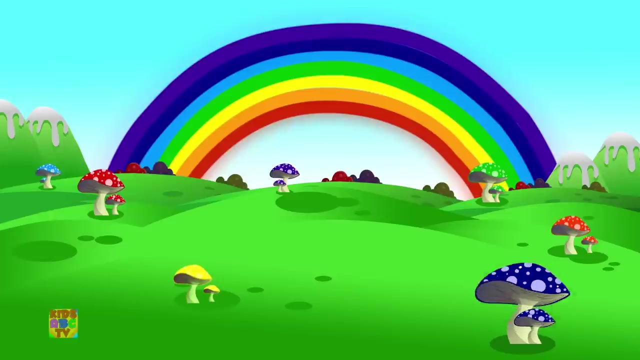 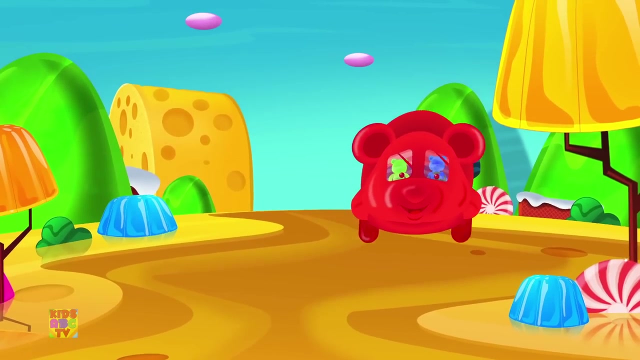 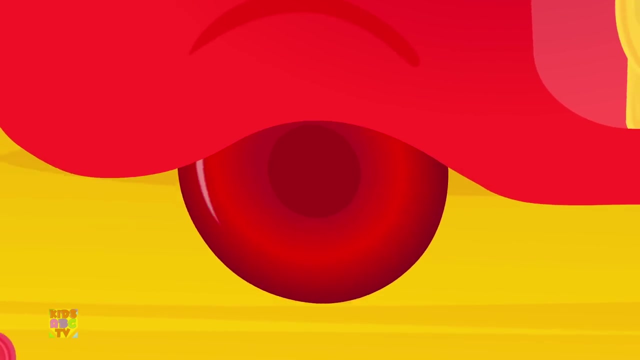 Blue, indigo and violet: These are the colors of the rainbow. Green, orange, yellow, green: These are the colors of the rainbow. Blue, indigo and violet: These are the colors of the rainbow. The wheels on the bus go round and round, round and round, round and round. 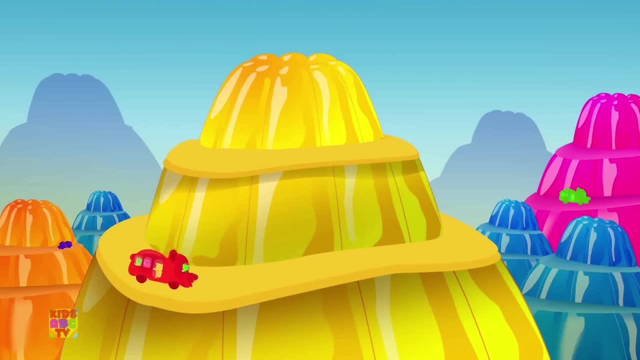 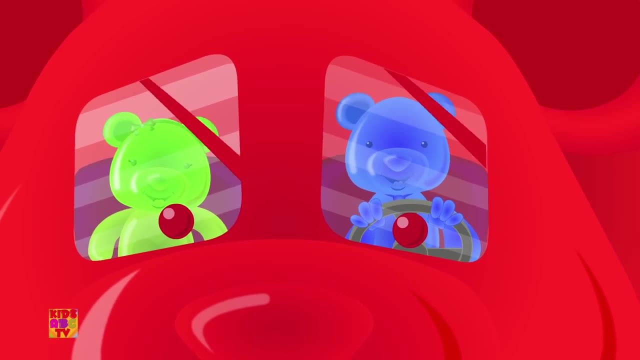 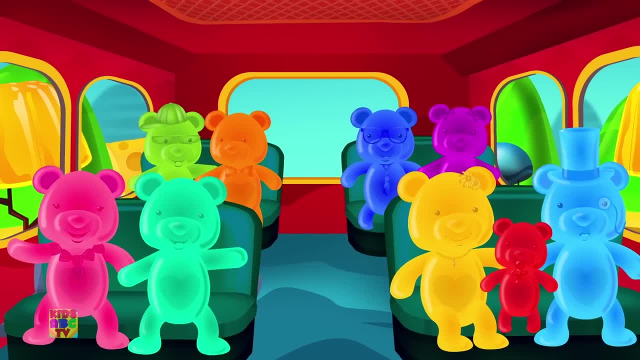 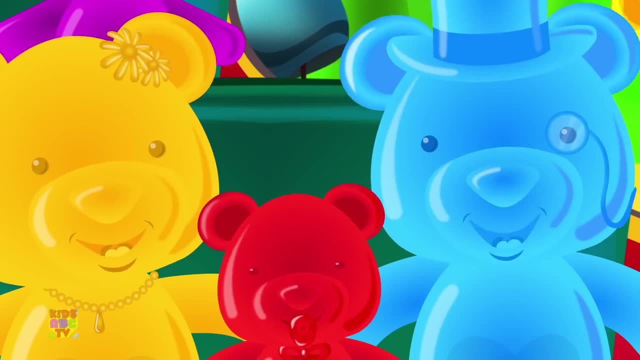 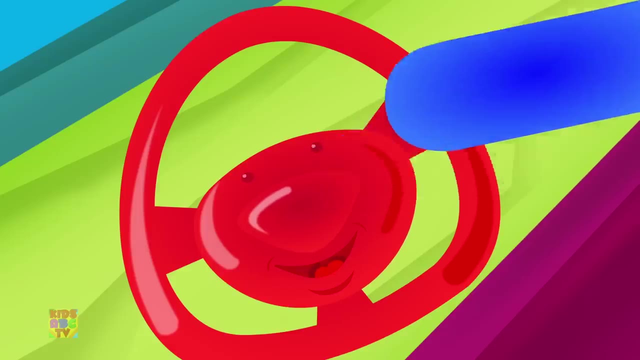 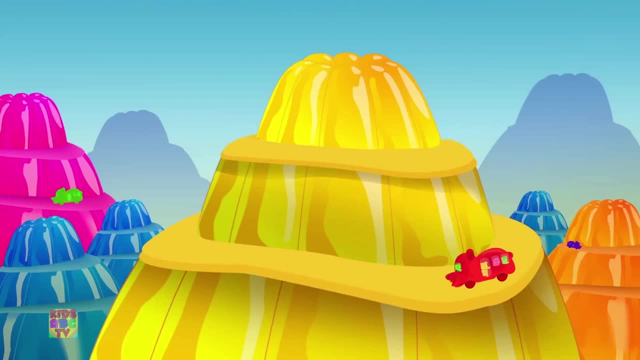 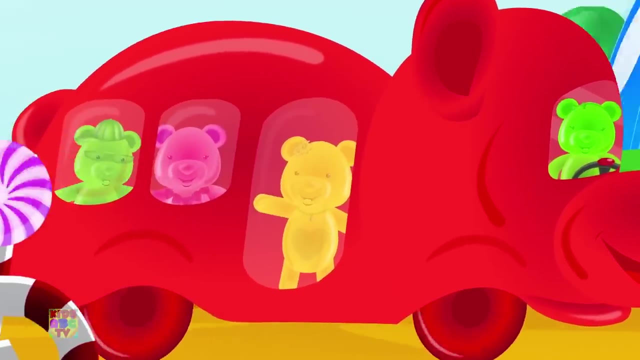 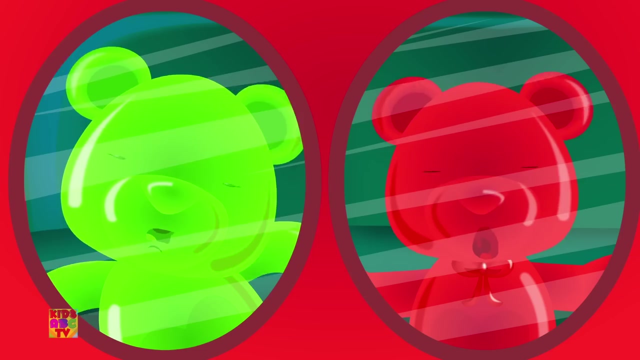 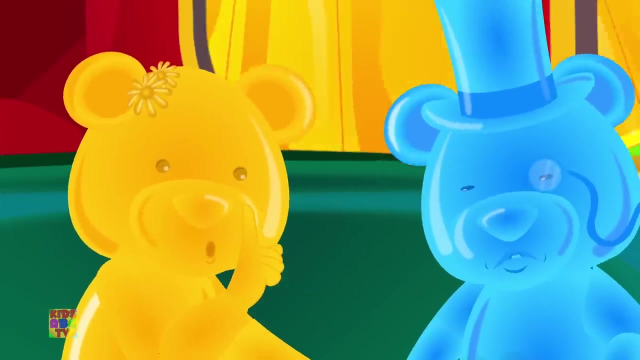 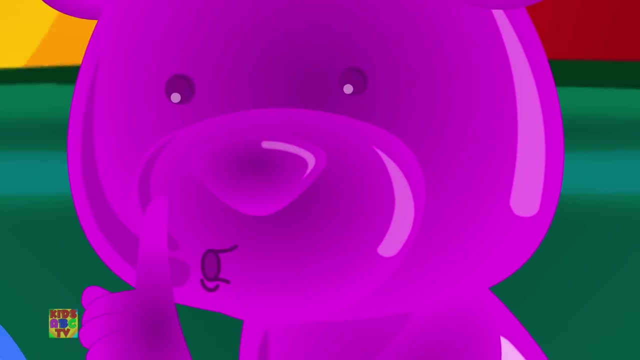 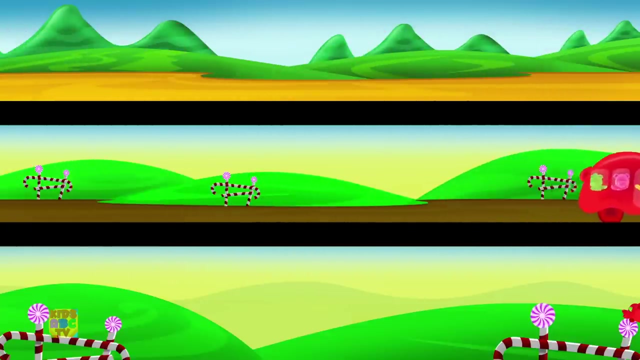 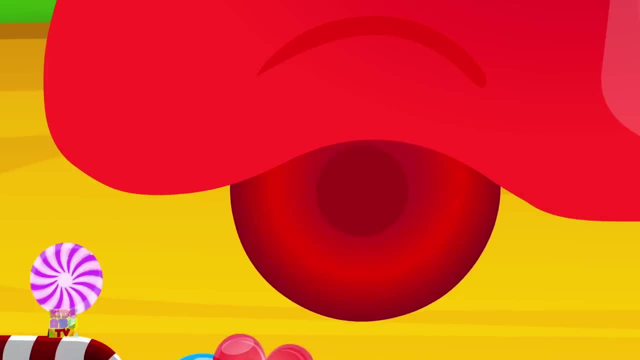 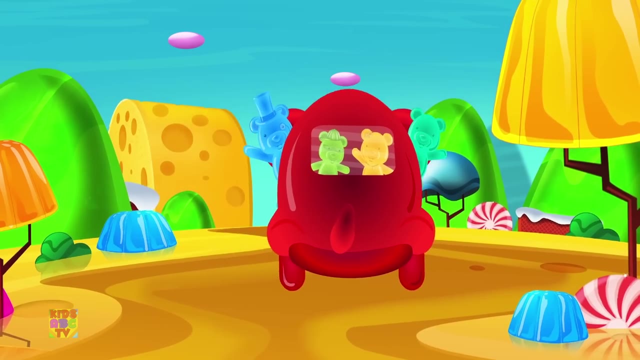 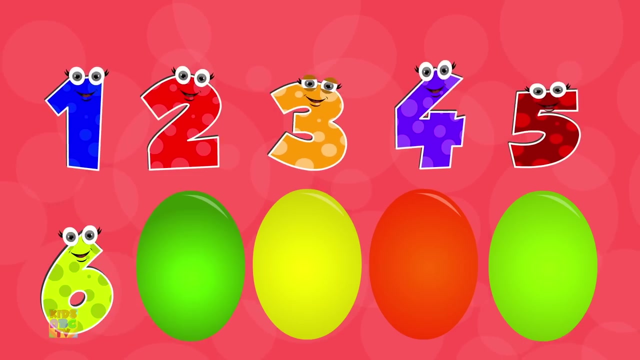 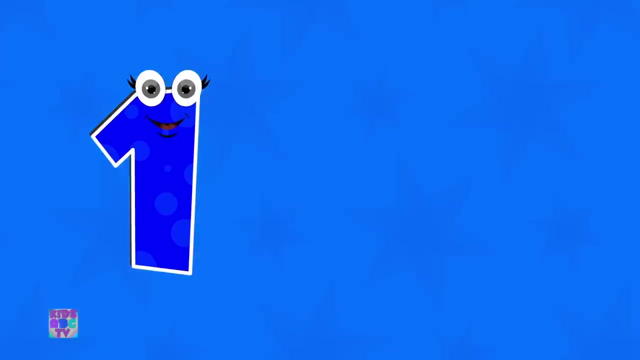 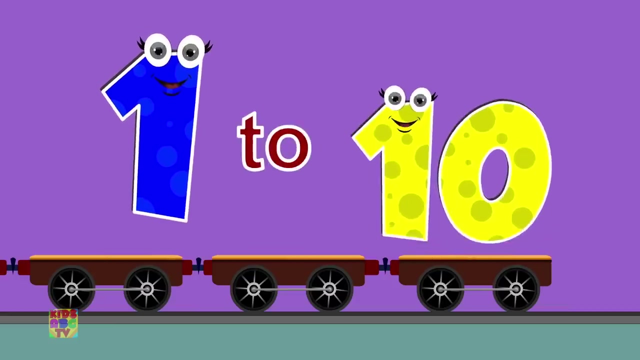 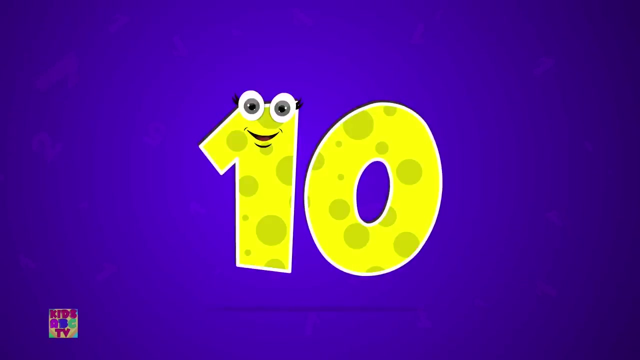 The wheels on the bus go round and round, Round and round, round and round. The wheels on the bus go round and round All through the town, One through ten. One, two, three, four, five, Six, seven, eight, nine, ten. One, two, three, four, five. 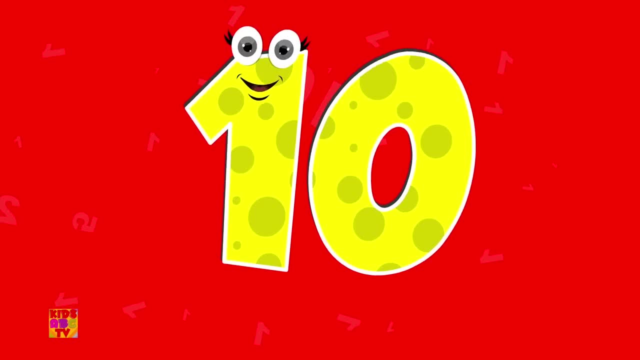 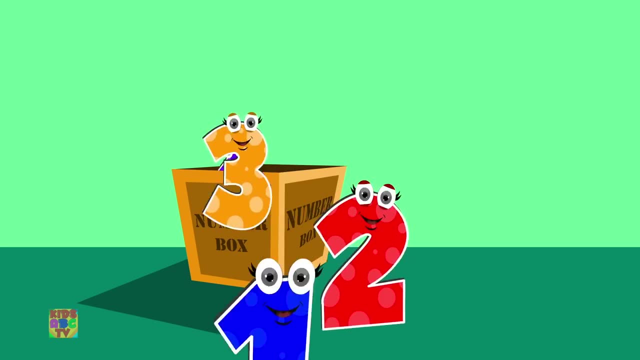 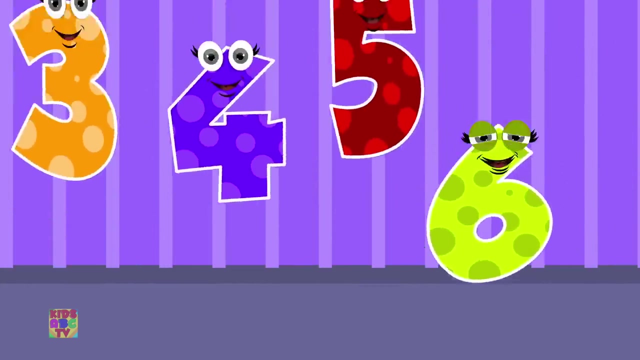 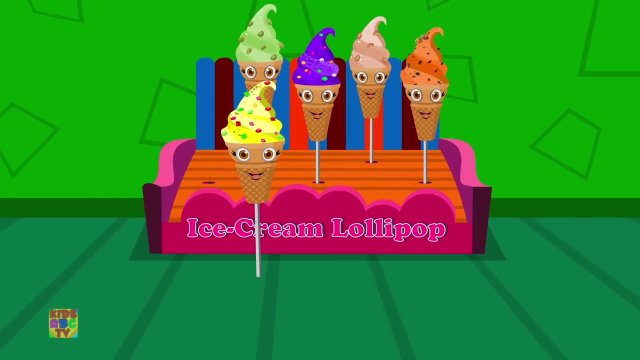 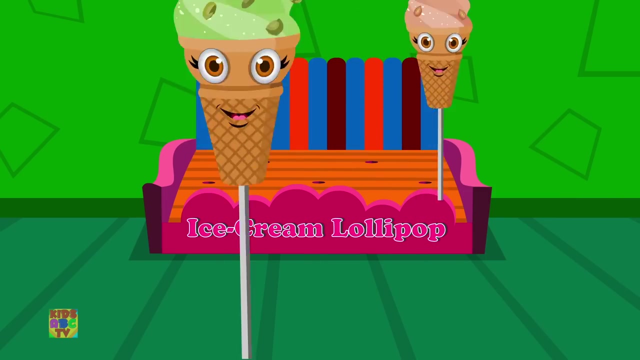 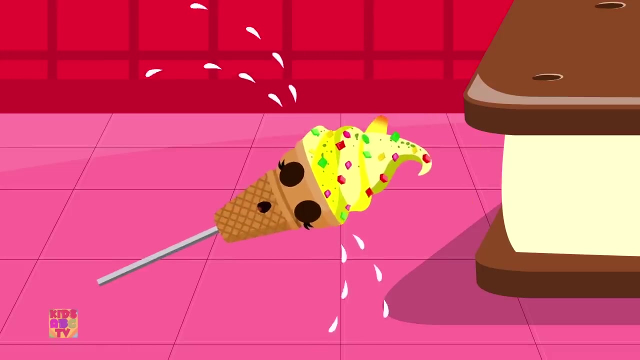 Six, seven, eight, nine, ten, Ten, ten, ten, ten. Here are your numbers One through ten. Here are your numbers One through ten. Five little lollipops jumping on the bed. One fell off and bumped his head. Baby called the doctor and the doctor said: 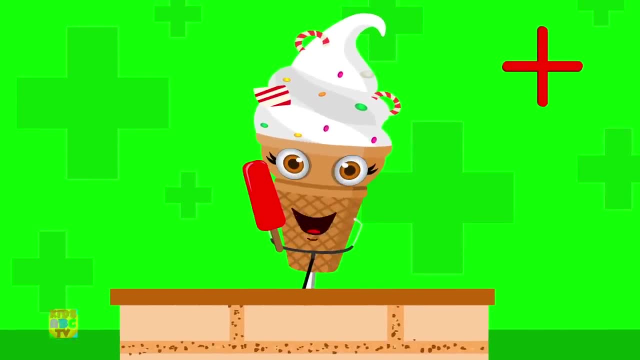 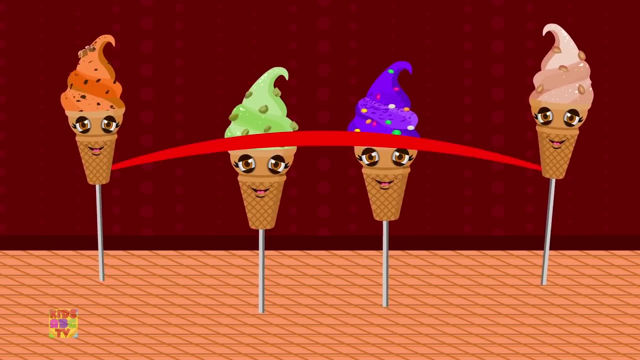 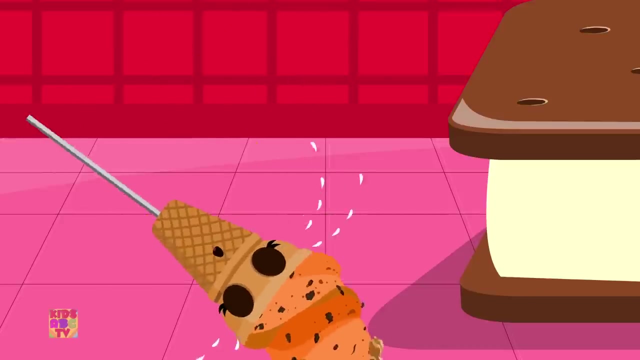 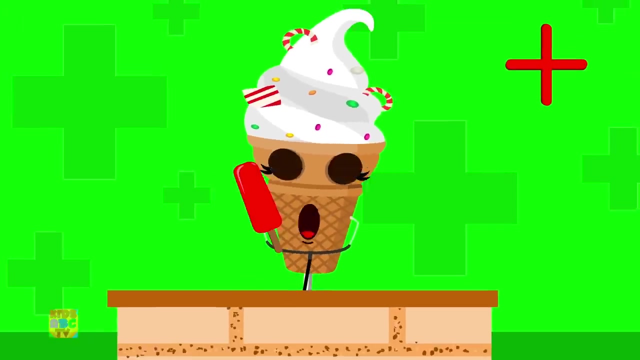 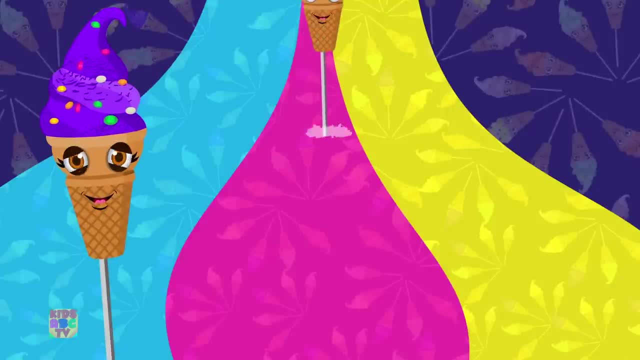 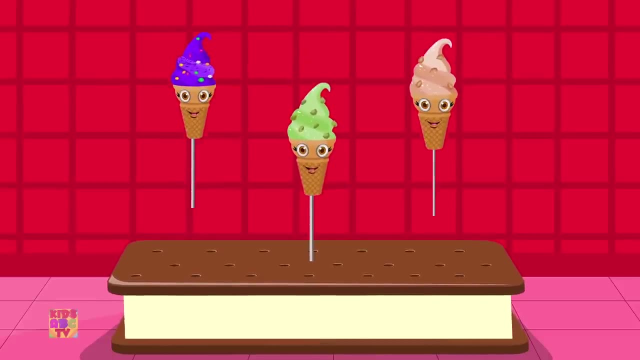 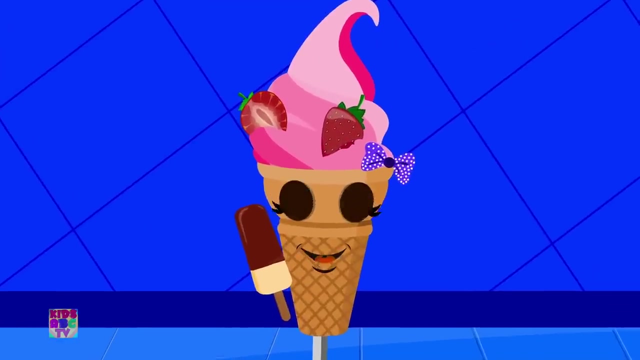 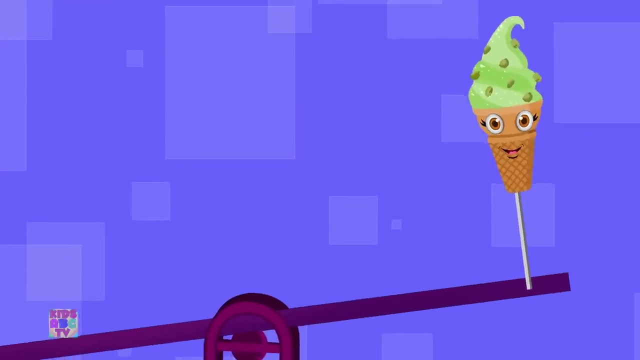 One through ten, One through ten, One through ten, One through eleven, One through twenty. Three little lollipops jumping on the bed. One fell off and bumped his head. Baby called the doctor and the doctor said: No more lollipops jumping on the bed. Here are your numbers. 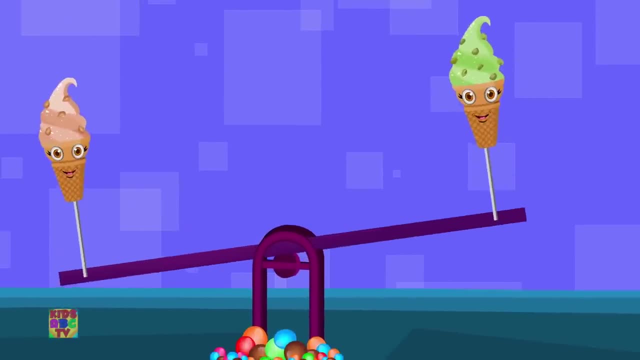 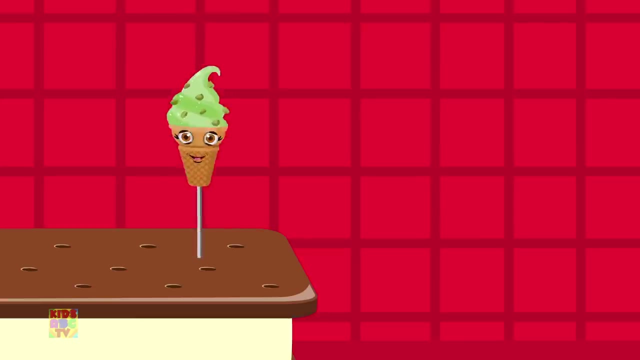 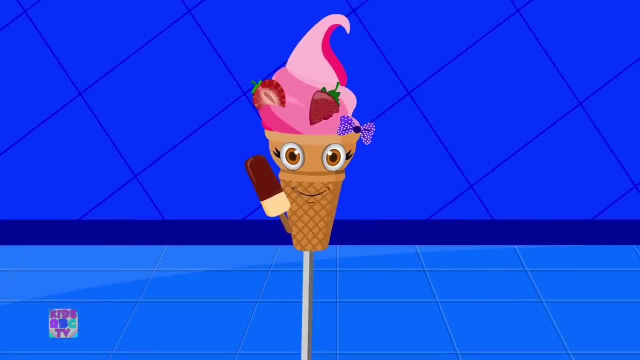 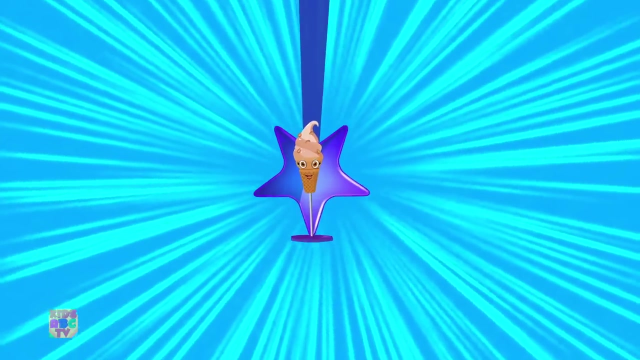 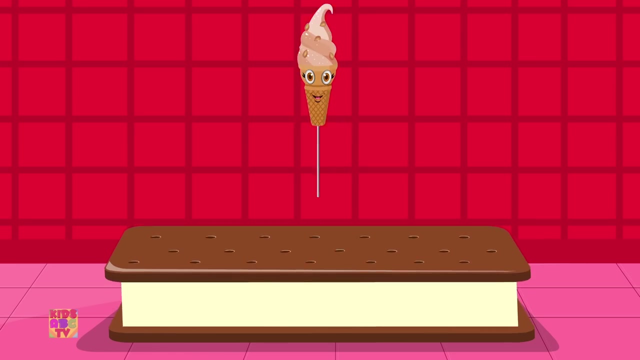 One through ten, One through ten, One through twenty and twenty. Two little lollipops jumping on the bed. One fell off and bumped his head. Baby called the doctor and the doctor said: No more lollipops jumping on the bed. One little lollipop jumping on the bed. 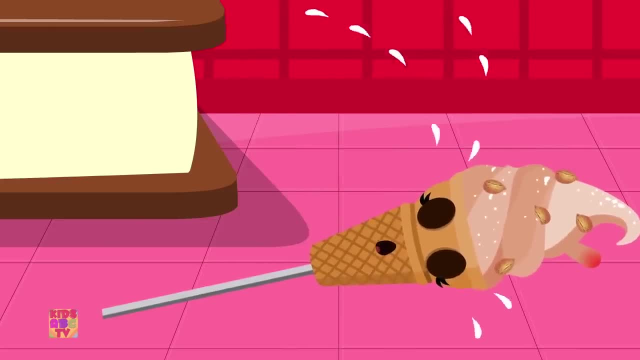 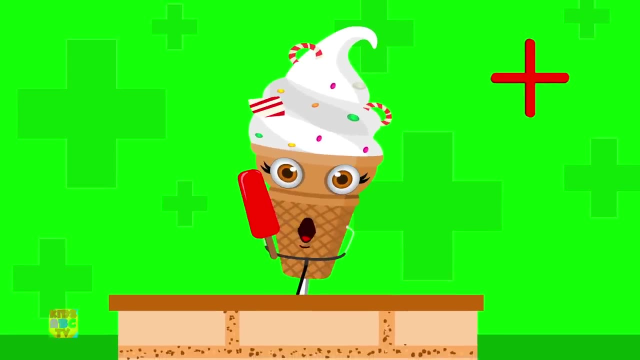 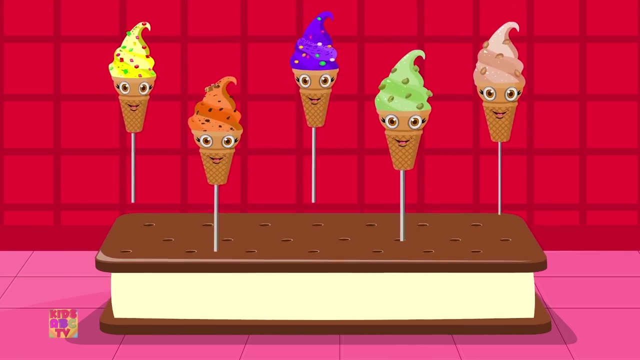 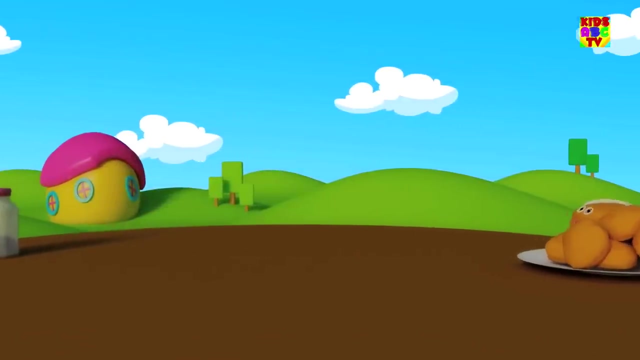 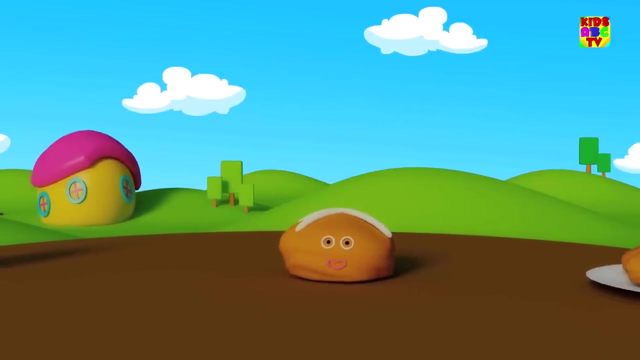 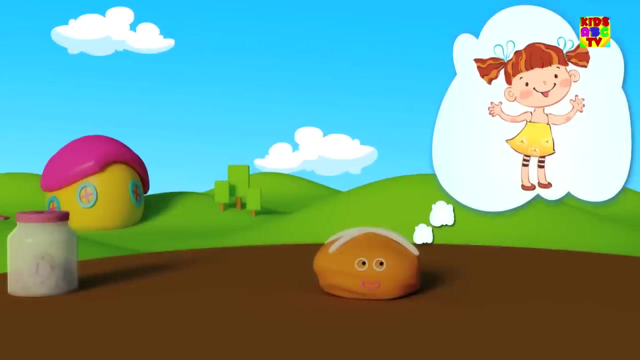 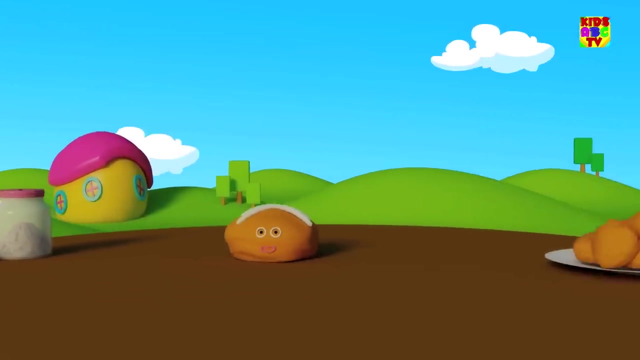 One fell off and bumped his head. Baby called the doctor and the doctor said: Put those lollipops right to bed. One a penny, two a penny hot cross buns. If you have no daughters, give them to your sons. One a penny, two a penny hot cross buns. Hot cross buns. get your hot cross buns, Hot cross buns, hot cross buns. One a penny, two a penny hot cross buns. If you have no daughters, Give them to your sons. One a penny, two a penny: hot cross buns. 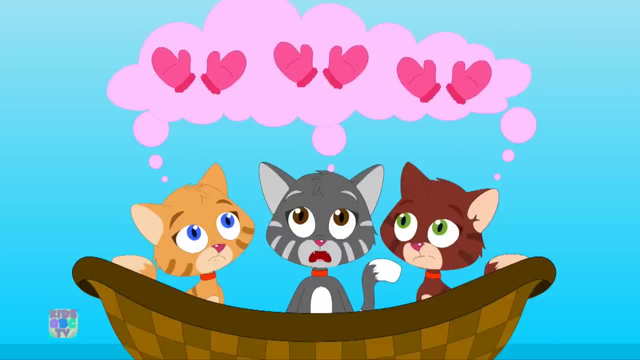 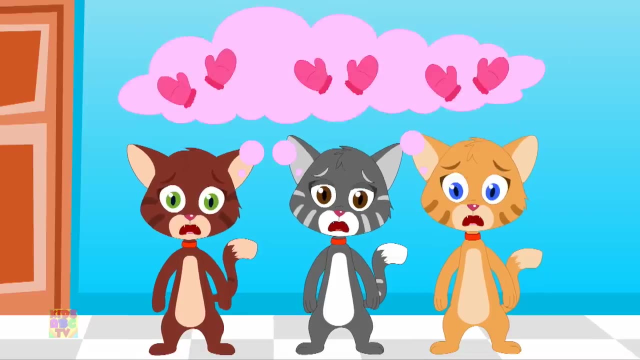 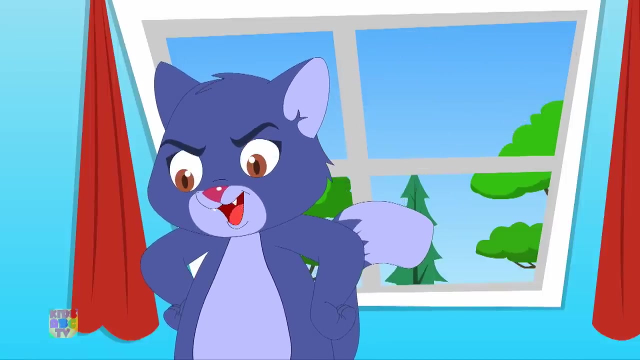 Three little kittens. they lost their mittens And they began to cry: Oh mother dear, we sadly fear Our mittens. we have lost What lost? your mittens, You naughty kittens. Then you shall have no pie. Meow, meow, meow, meow. 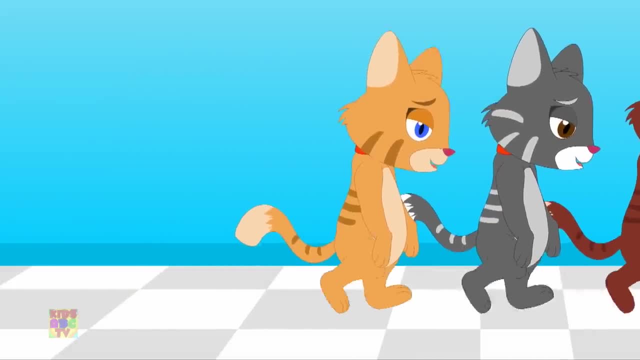 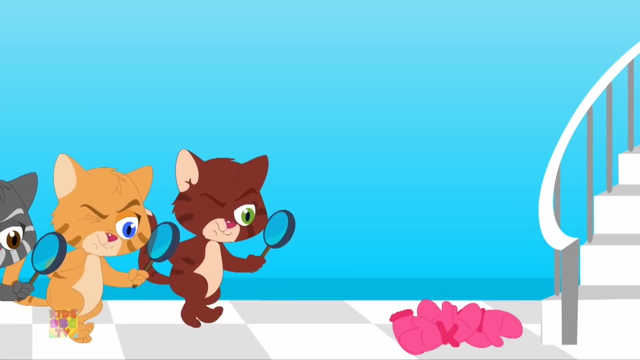 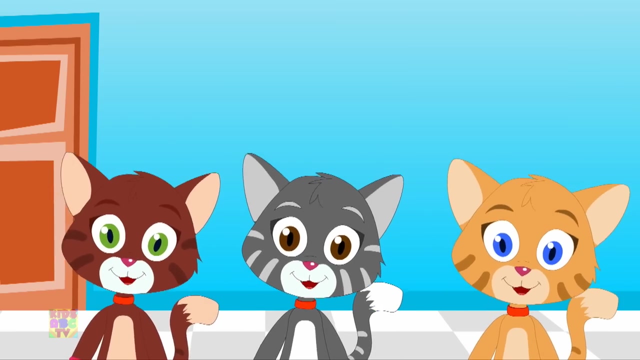 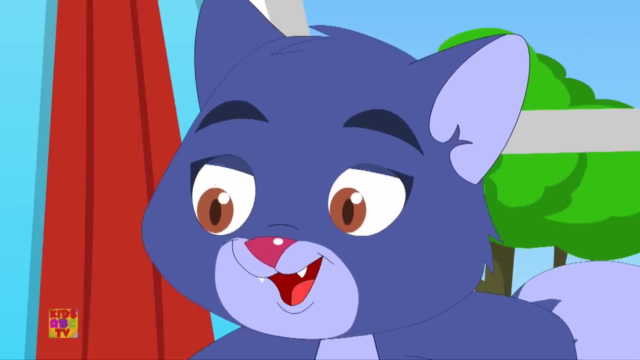 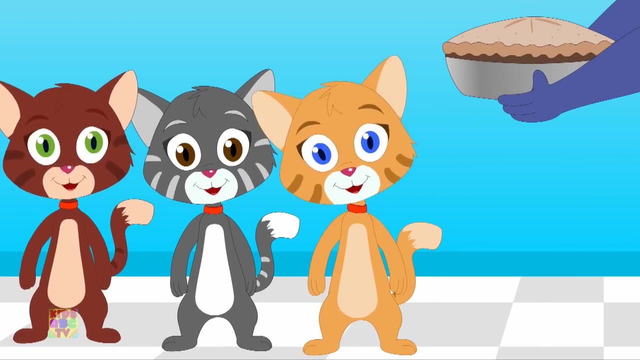 We shall have no pie. Three little kittens, They found their mittens And they began to cry: Oh mother dear, see here, see here, Our mittens. we have found What found: your mittens, You darling kittens. Then you shall have some pie, Meow, meow, meow, meow. 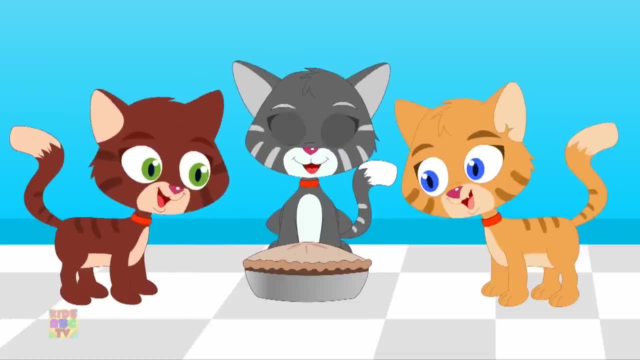 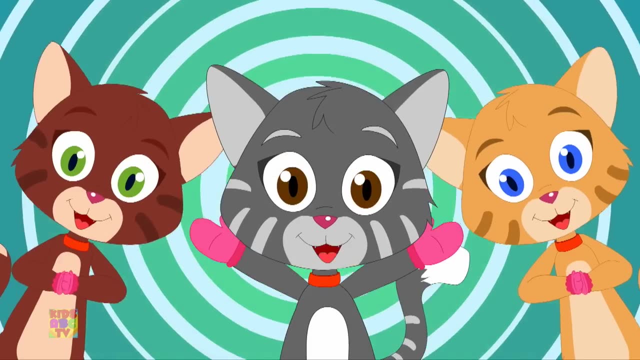 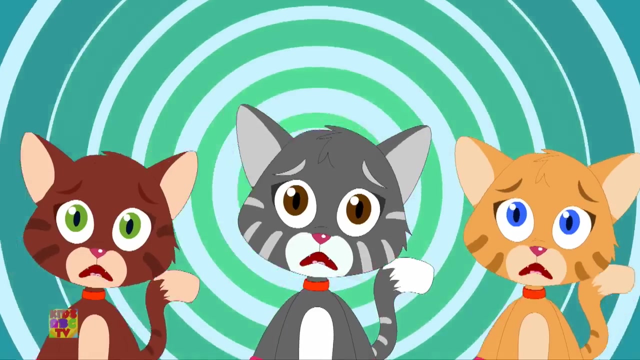 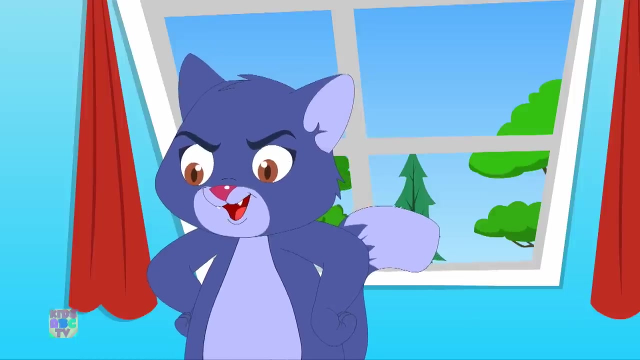 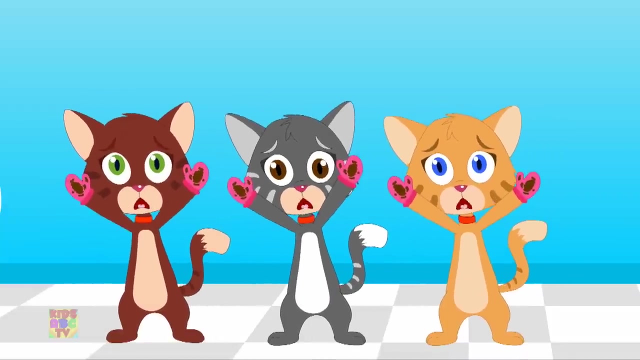 We shall have some pie. Three little kittens put on their mittens And soon ate up the pie. Oh, mother dear, we greatly fear Our mittens. we have soiled What soiled? your mittens, You naughty kittens. They began to sigh: Meow, meow, meow, meow. 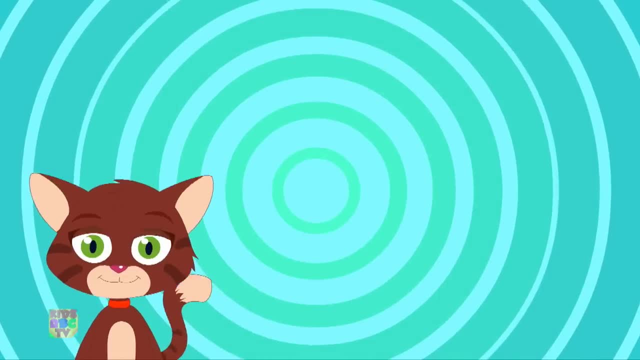 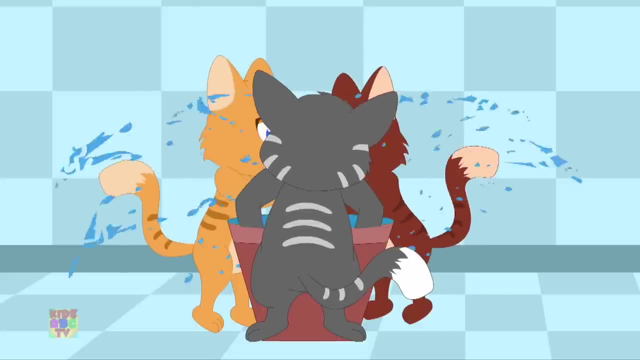 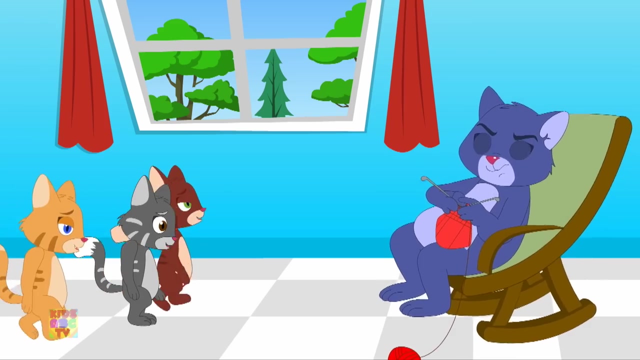 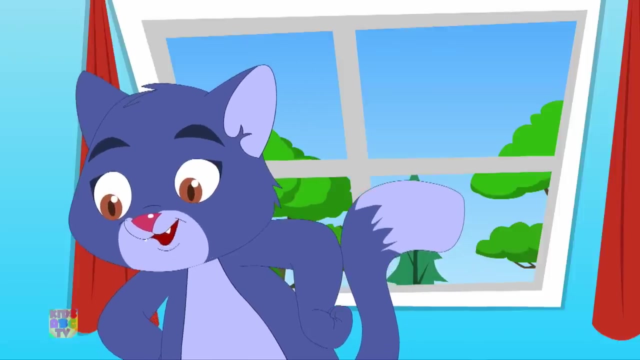 Our mittens. we have soiled Meow, meow, meow meow, Three little kittens. They washed their mittens And hung them out to dry. Oh, mother dear, look here, look here, Our mittens. we have washed What washed your mittens. 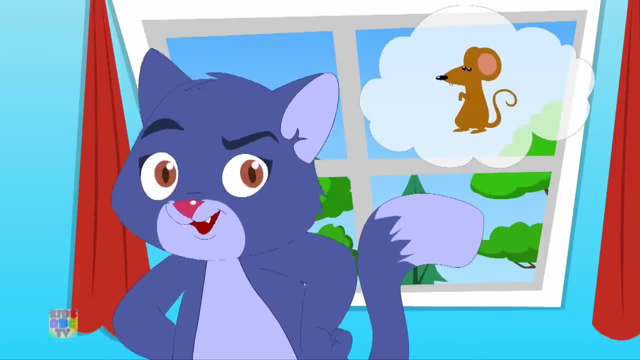 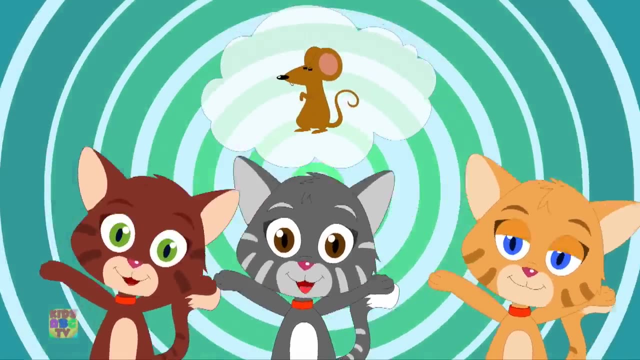 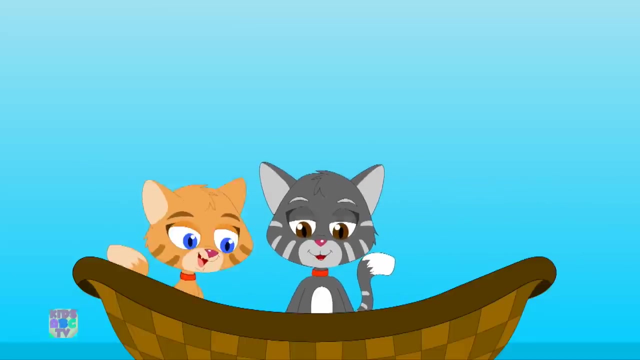 You're such good kittens. I smell a rat close by Meow, meow, meow, meow. We smell a rat close by Meow, meow, meow, meow. We smell a rat close by Meow meow, meow, meow. 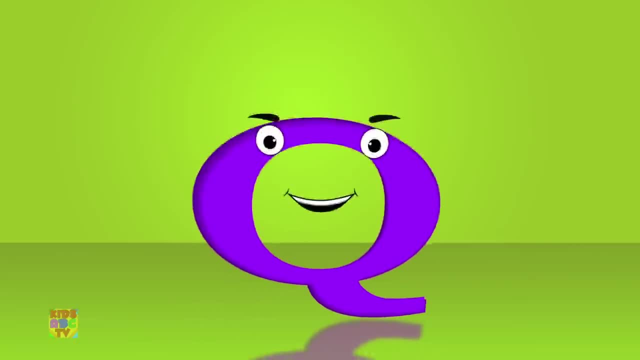 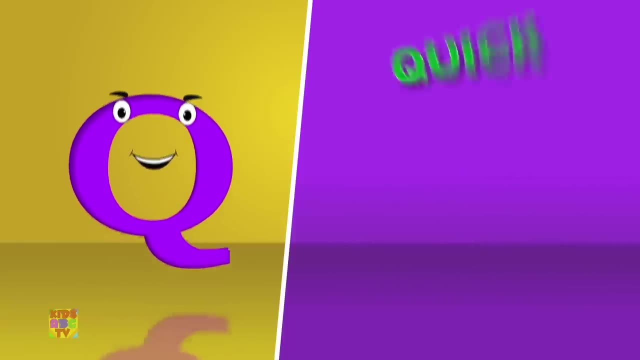 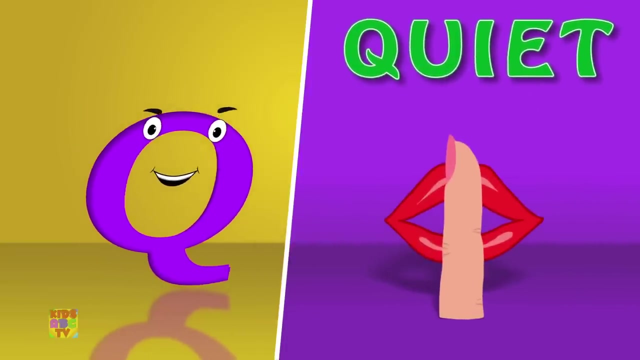 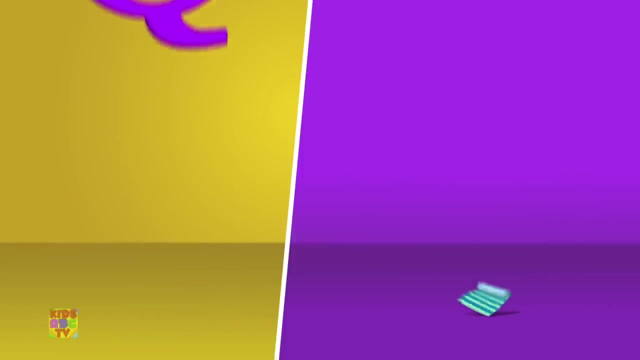 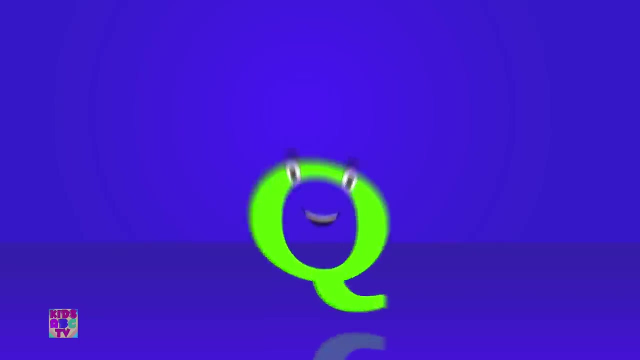 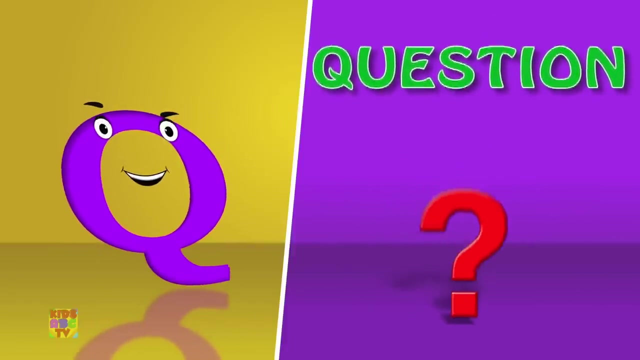 Here comes the letter: Q Q is for Queen Q Q. Queen Q is for Quick Q Q. Quick Q is for Quiet Q Q. Quiet Q is for Quilt Q Q. Quilt Q is for Question Q Q. Question Q is for Quiz Q Q. Quiz Q is for Quiver. 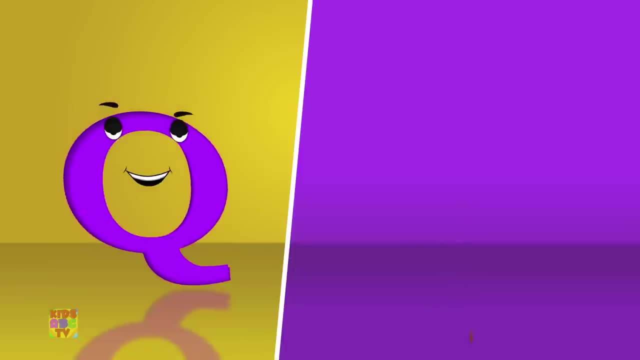 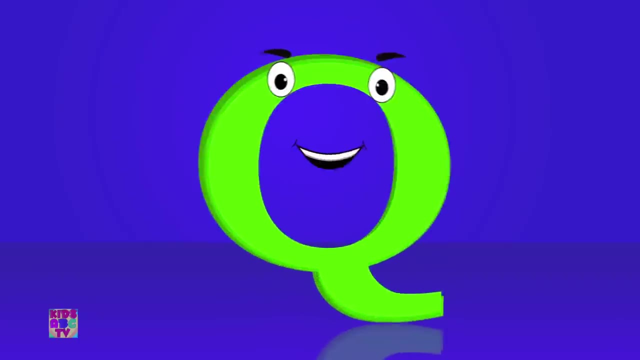 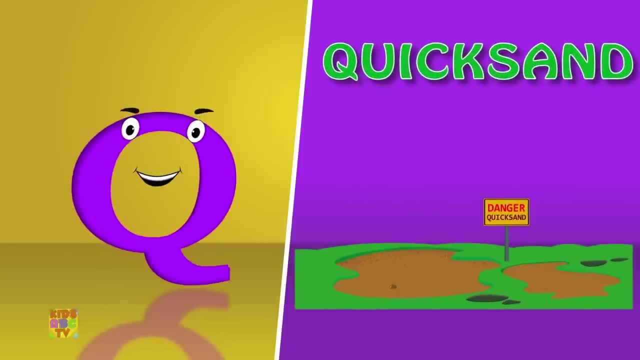 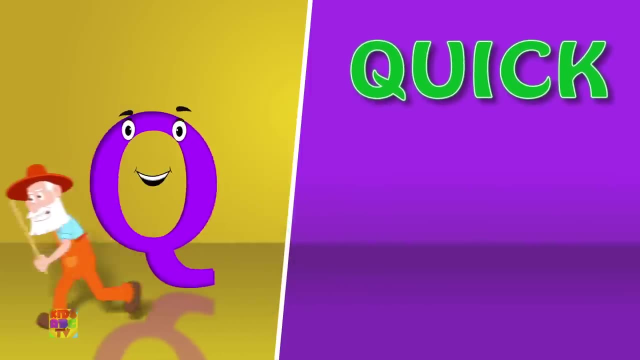 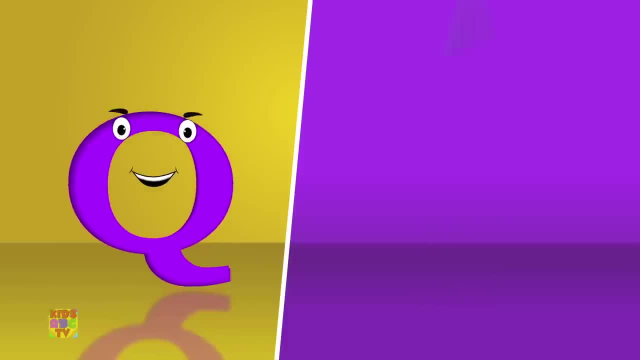 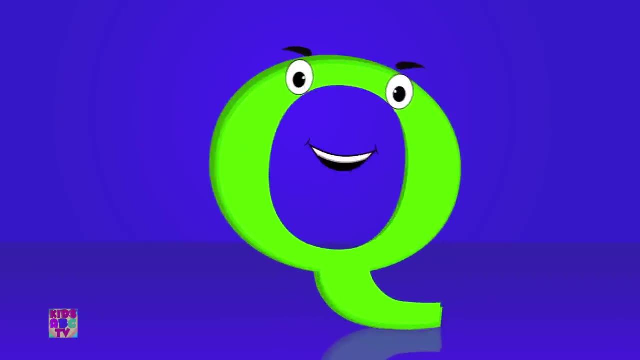 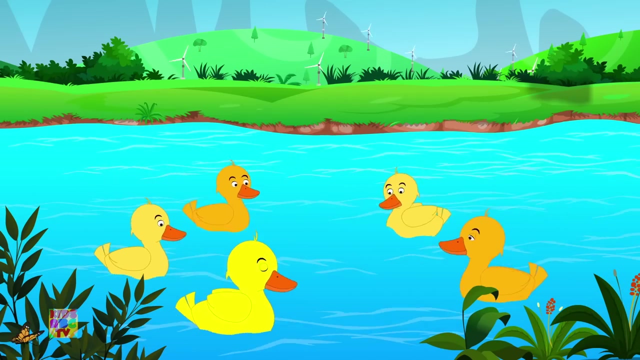 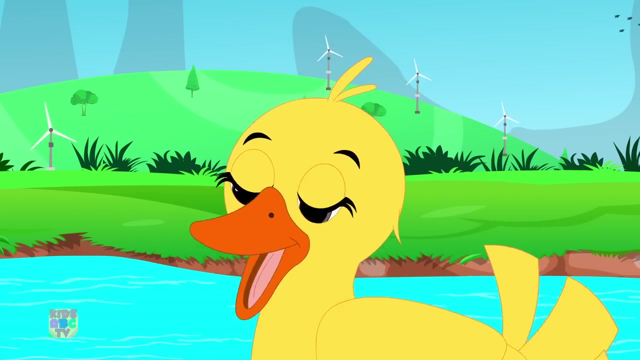 Question q q. question Q is for Queen Bee, q q, Queen Bee. Five little ducks went swimming one day Over the hill and far away, Mother duck said quack, quack, quack, And only four little ducks came back. 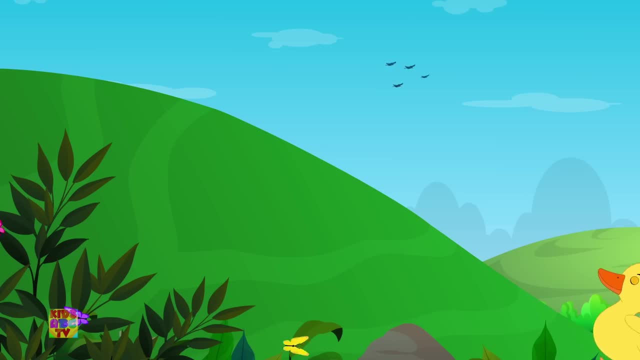 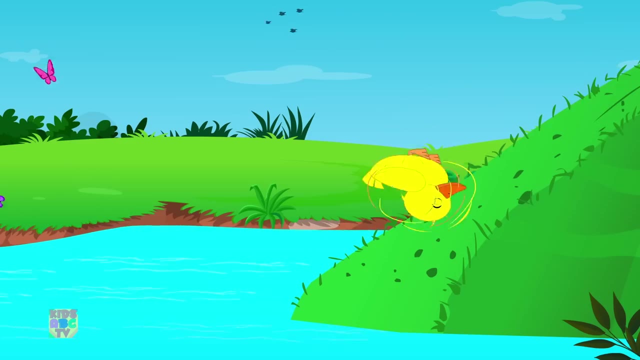 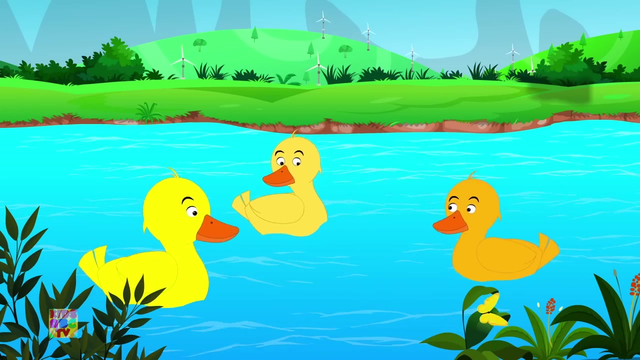 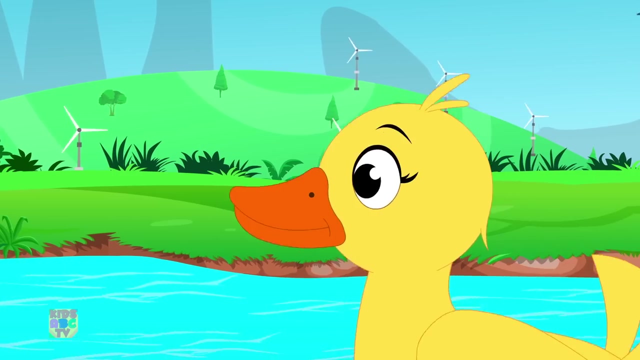 Four little ducks went swimming one day Over the hill and far away, Mother duck said quack, quack, quack, And only three little ducks came back. Three little ducks went swimming one day Over the hill and far away, Mother duck said quack, quack, quack, And only two little ducks came back. 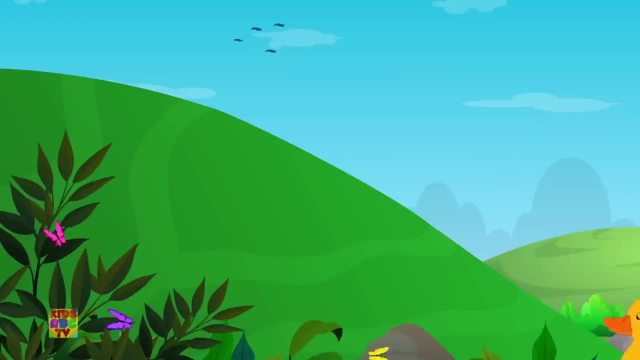 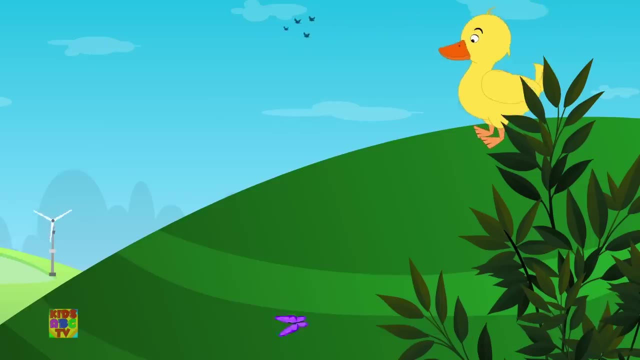 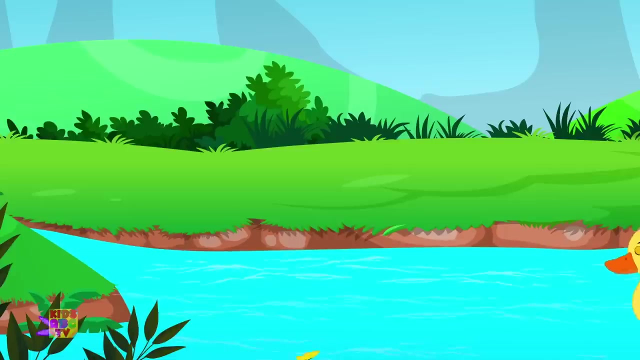 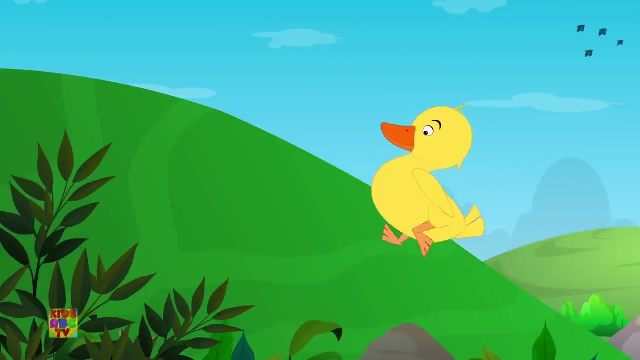 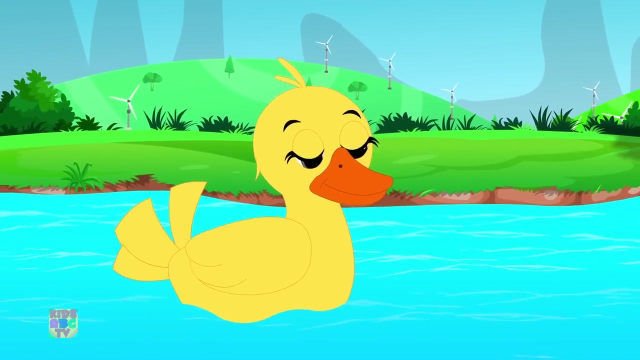 Two little ducks went swimming one day Over the hill and far away, Mother duck said quack, quack, quack, And only one little duck came back. One little duck went swimming one day Over the hill and far away, Mother duck said quack, quack, quack, And all five little ducks came back. 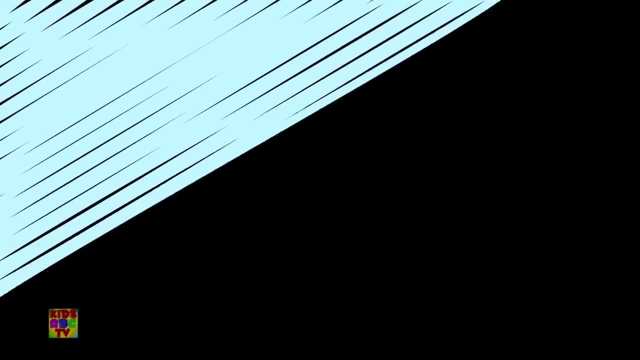 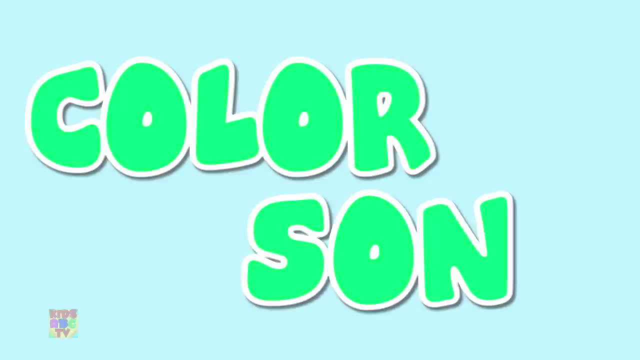 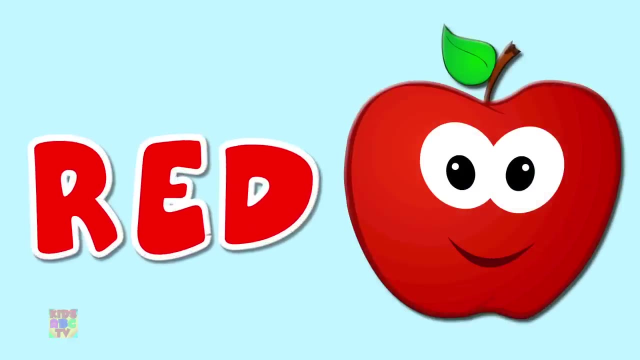 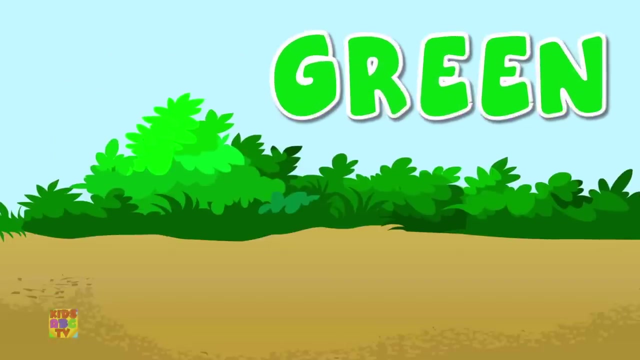 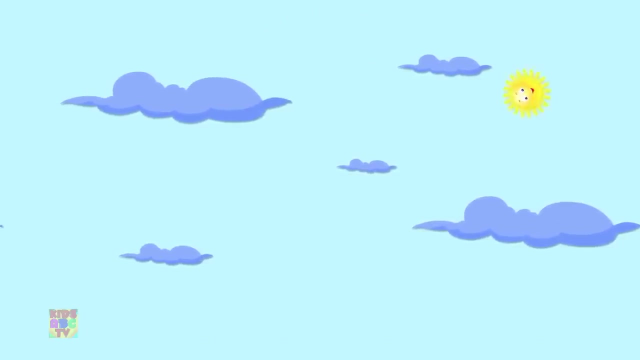 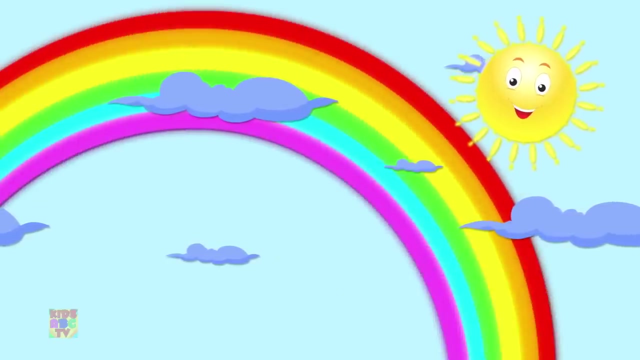 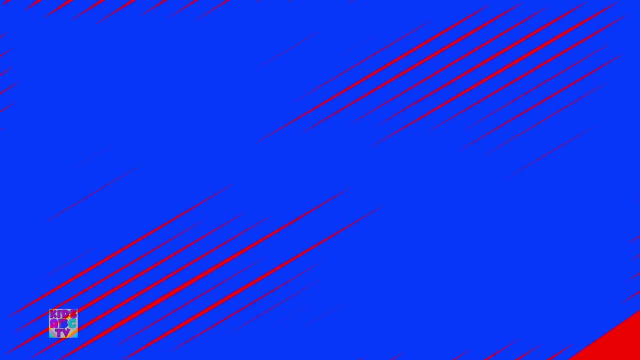 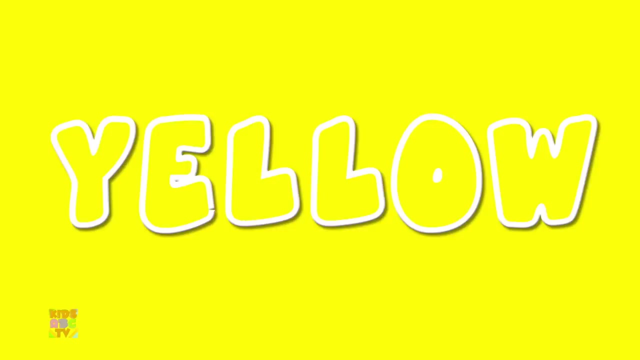 An apple is red, red, red. The sky is blue, blue, blue. The grass is green, green, green. The sun is yellow, yellow. So many colors everywhere. Look at them all around. So many colors everywhere. Look at them all around. The snow is white, white, white. 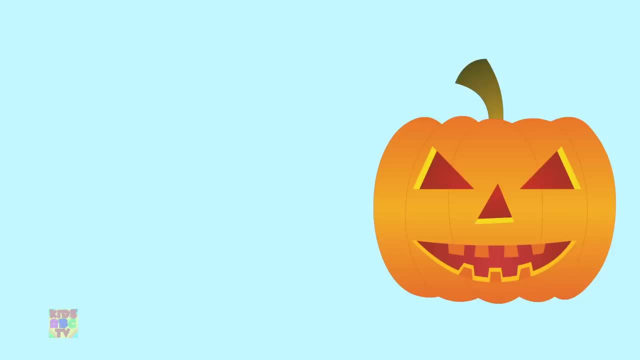 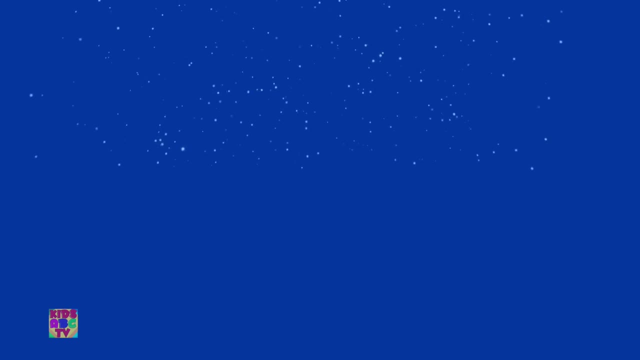 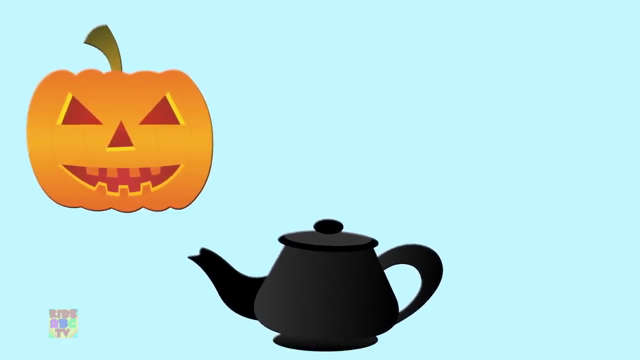 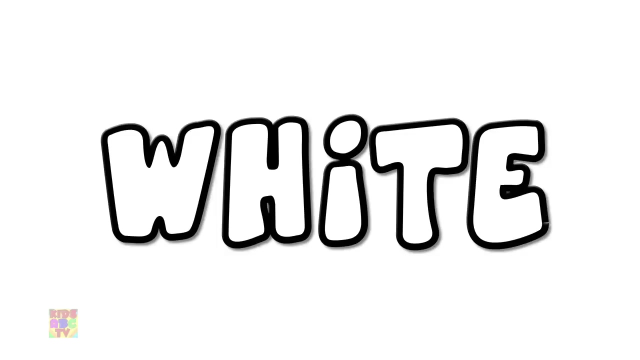 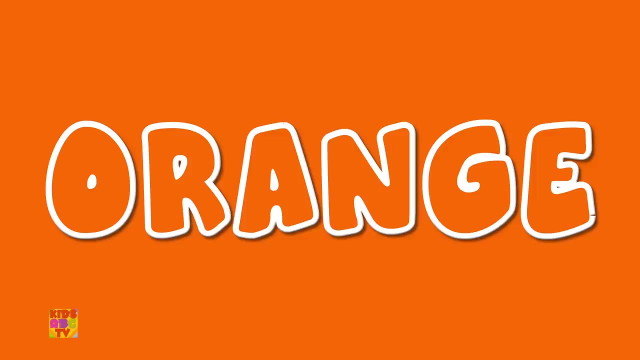 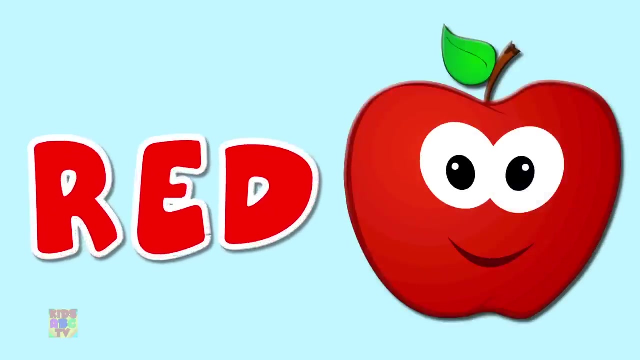 The kettle is black, black, black, The pumpkin is orange, orange, And my tongue is pink, pink, pink. So many colors everywhere. Look at them all around. So many colors everywhere. Look at them all around. An apple is red, red, red. The sky is blue, blue, blue. 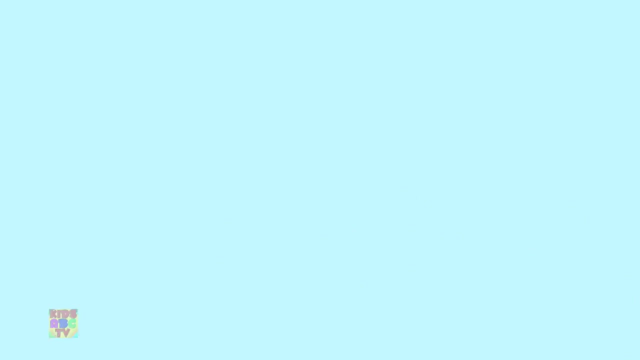 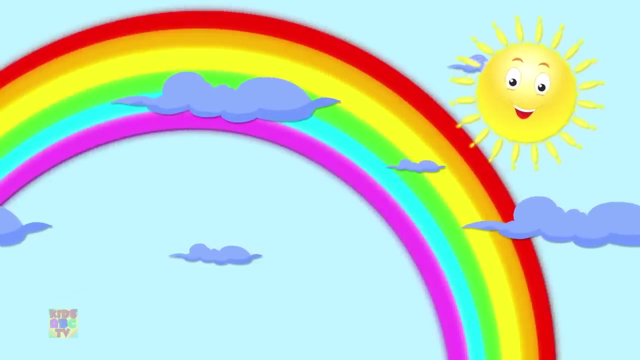 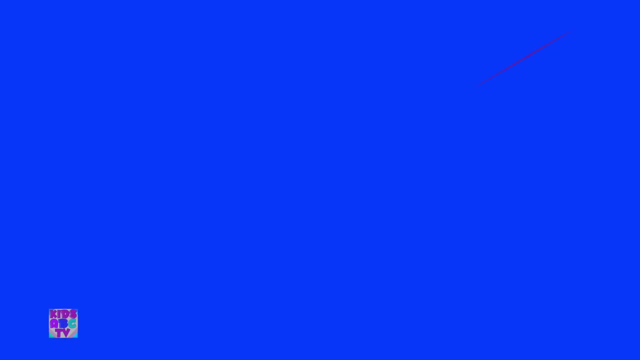 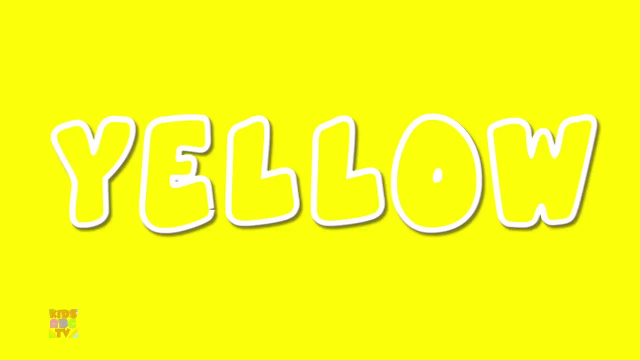 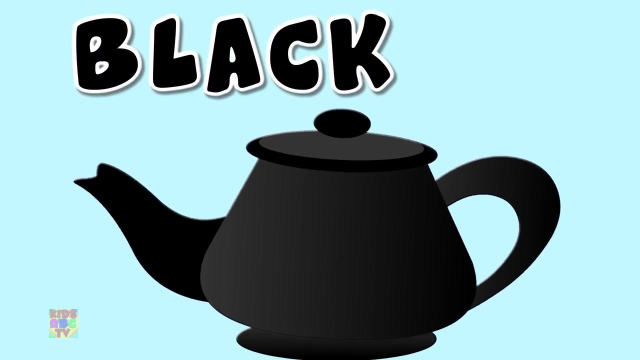 The grass is green, green, green. The sun is yellow, yellow. So many colors everywhere. Look at them all around. So many colors everywhere. Look at them all around. Look at them all around. The snow is white, white, white. The kettle is black, black, black. 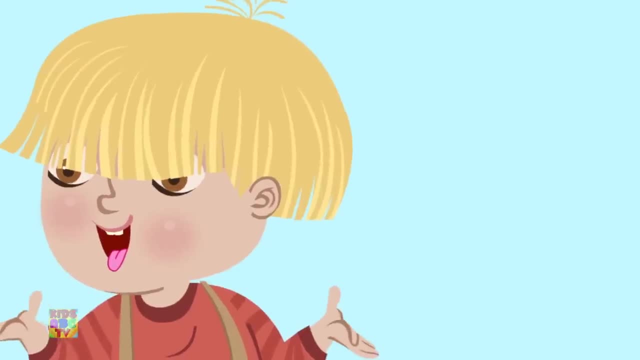 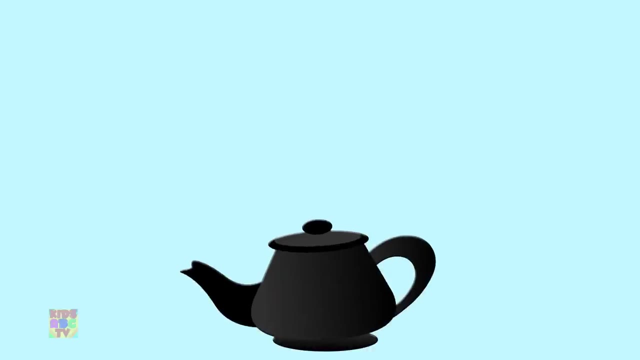 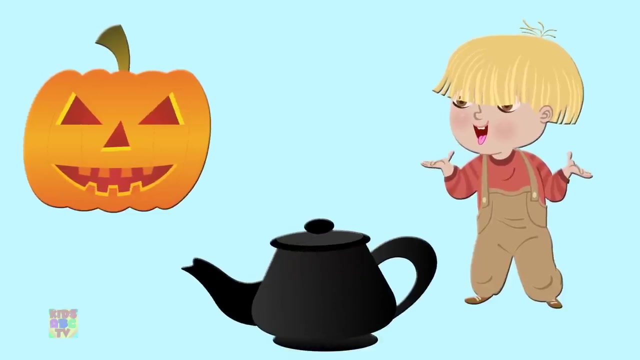 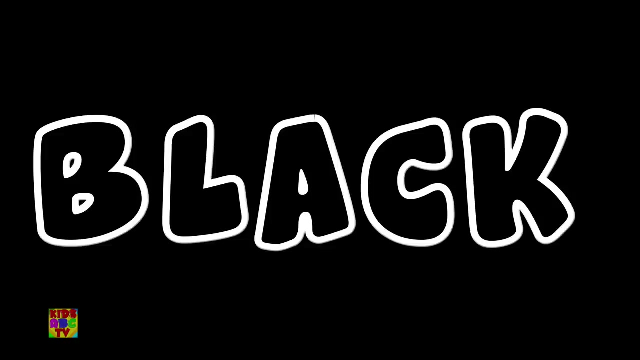 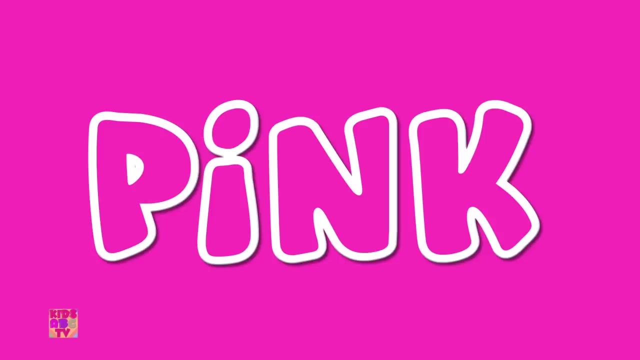 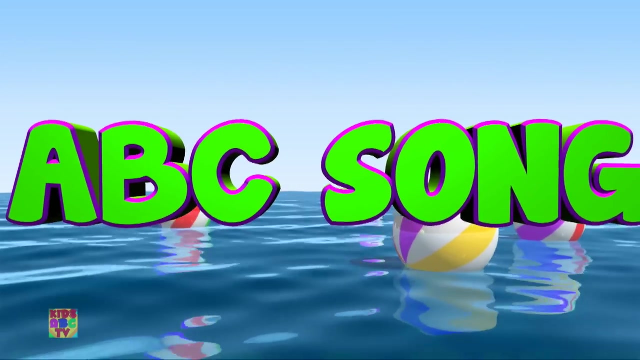 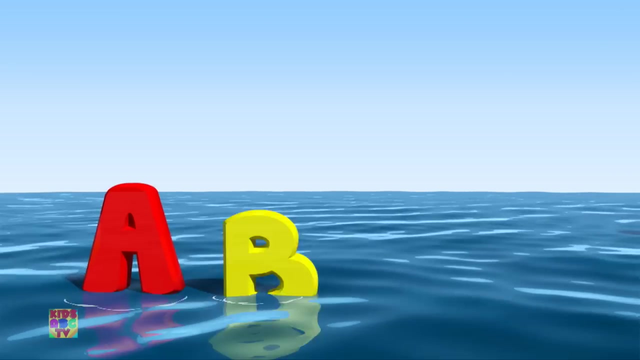 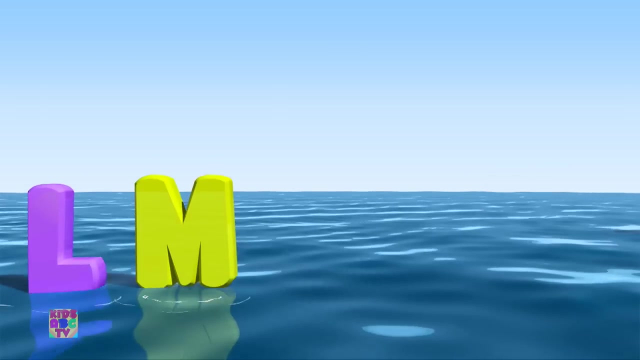 The pumpkin is orange, orange And my tongue is pink, pink, pink. So many colors everywhere. Look at them all around. So many colors everywhere. Look at them all around. A, B, C, D, E, F, G, H, I, J, K, L, M, N, O, P. 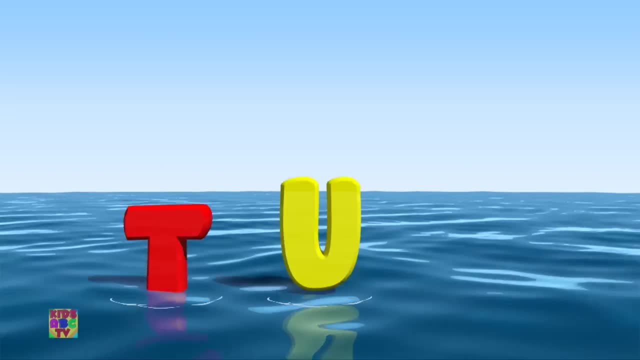 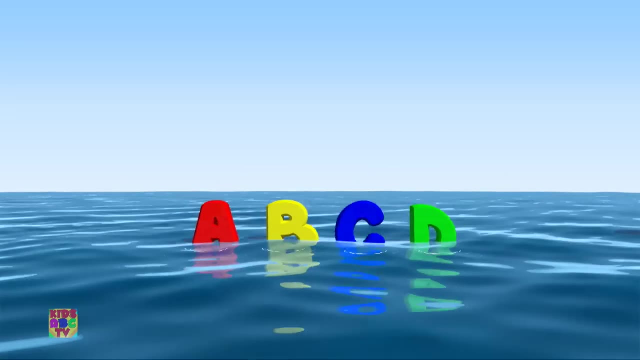 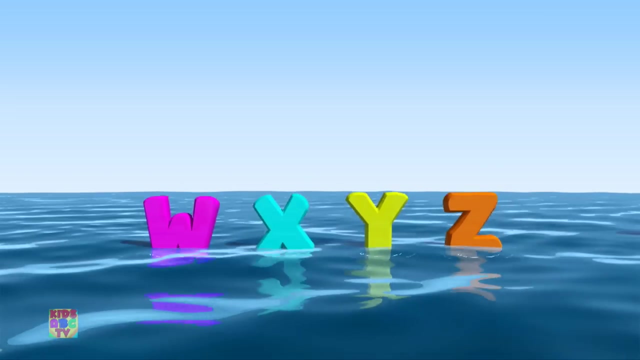 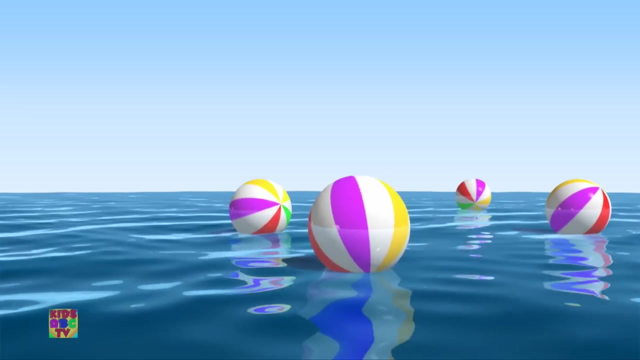 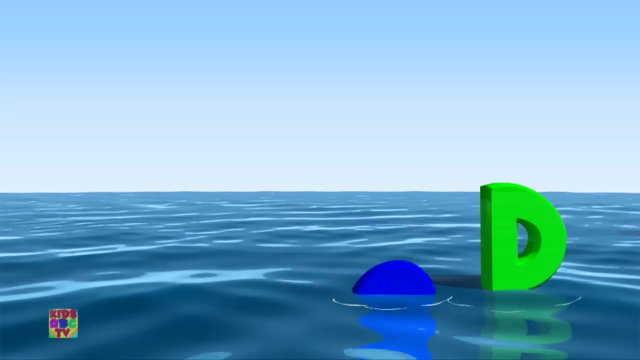 Q, R, S, T, U, V, W, X, Y and Z. Now I know my ABCs. Twenty twenty, twenty, Twenty, twenty, twenty, Twenty-six letters from A, to Z, A, B, C, D, E, F, G. 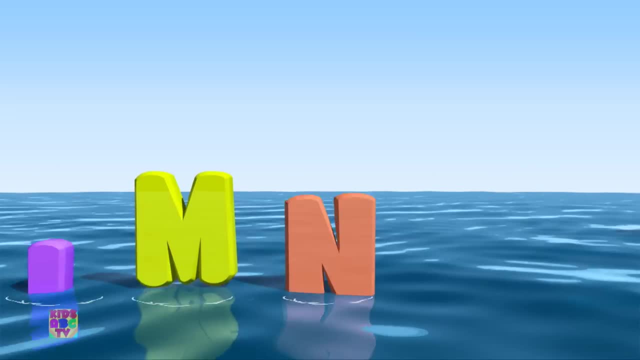 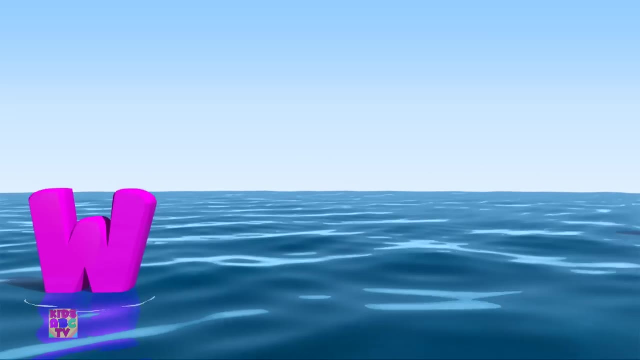 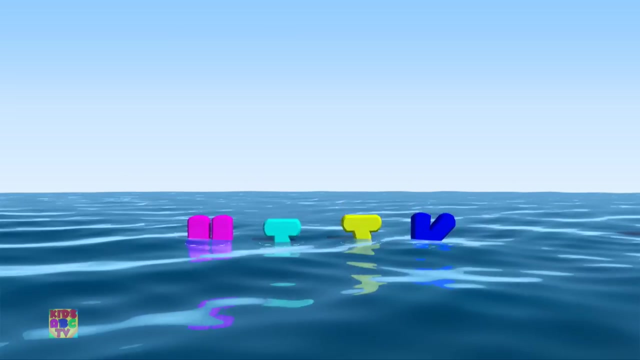 H I J K L M N O P. Q R S T U V W, X, Y and Z. H I J K L M N O P. 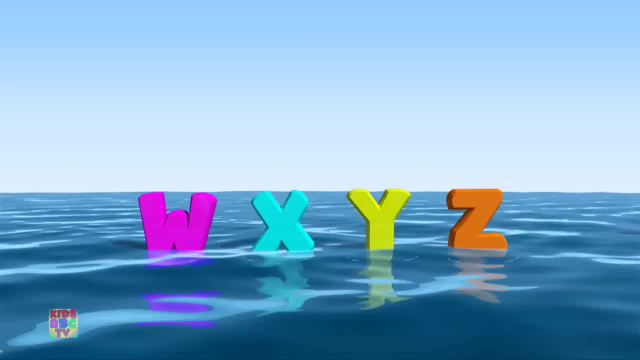 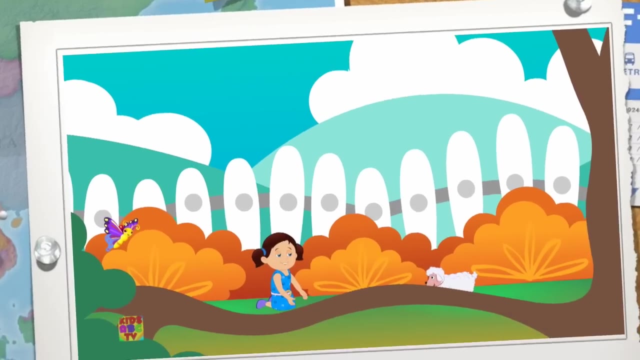 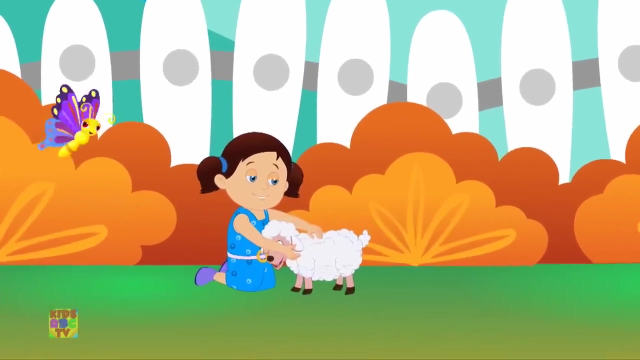 Q R S T U V, X, Y and Z Q R S T U V. Q R S T U V A, B, C, D, E, F, F, Y, L, X. 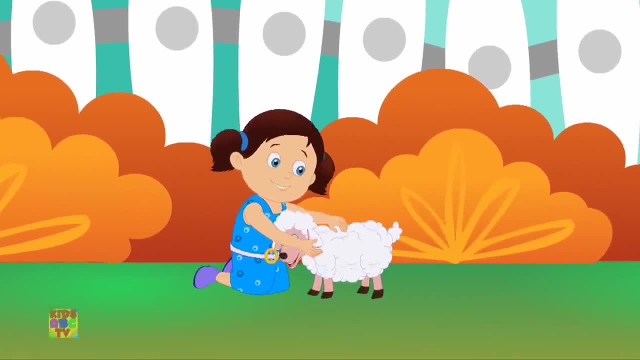 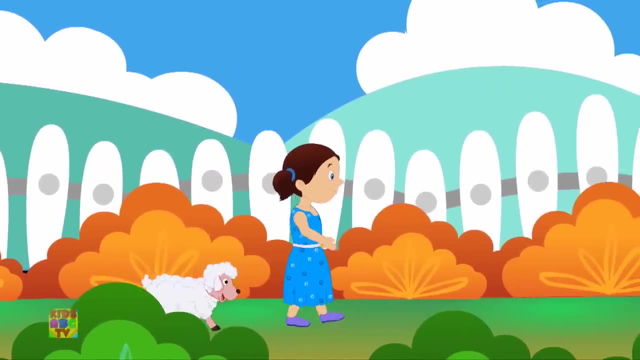 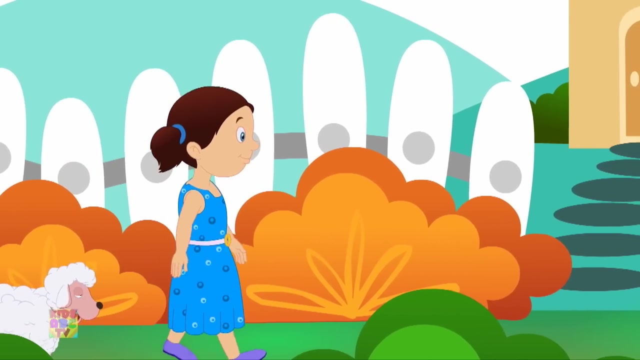 Y Y Z, Q R S T U V, Q R S T U V. White as snow. And everywhere that Mary went, Mary went, Mary went. And everywhere that Mary went, The lamb was sure to go. It followed her to school one day. 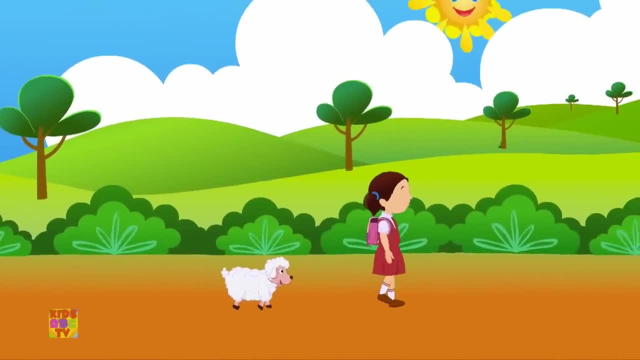 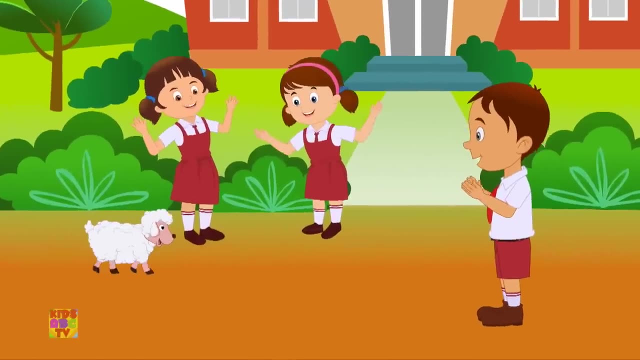 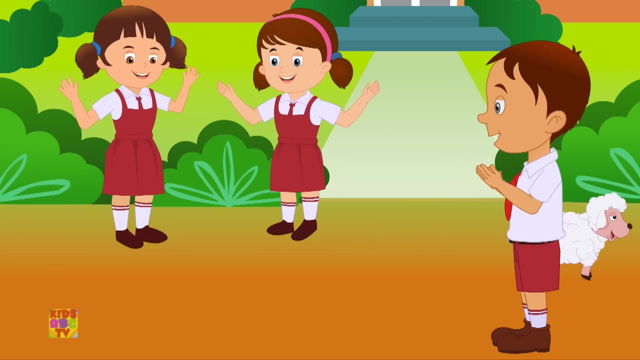 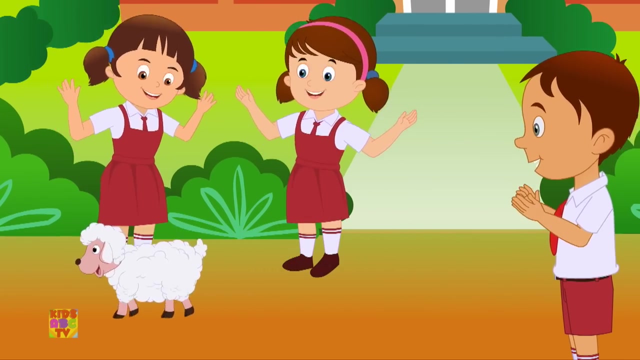 School one day- School one day. It followed her to school one day, Which was against the rules. It made the children laugh and play, Laugh and play, Laugh and play. It made the children laugh and play To see a lamb at school, And so the teacher turned it out. 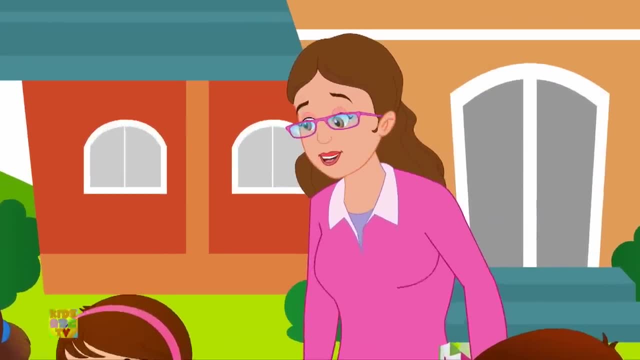 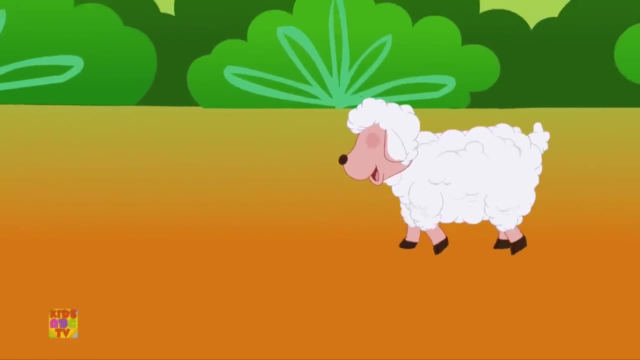 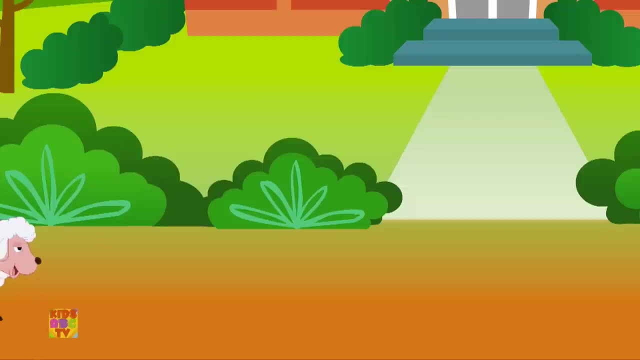 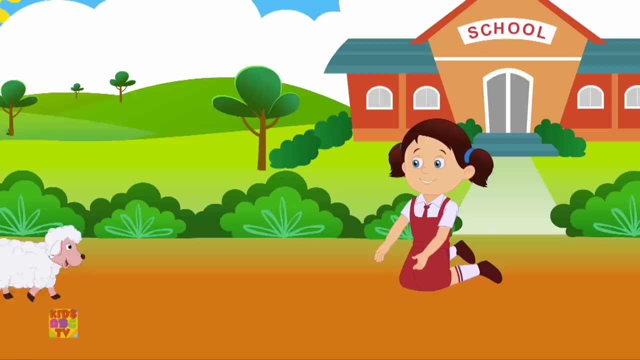 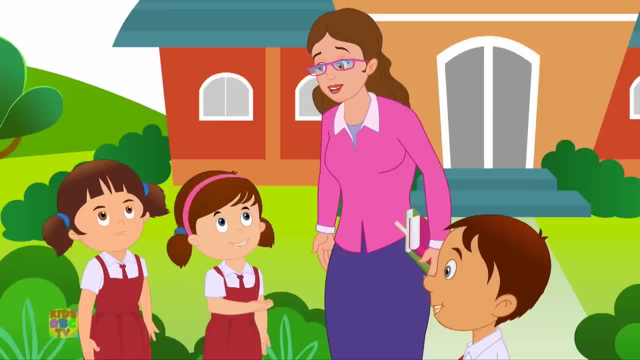 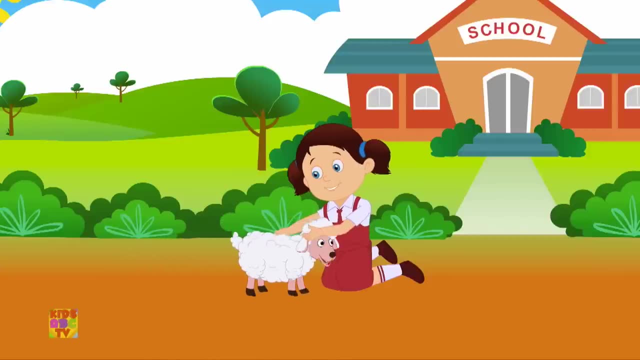 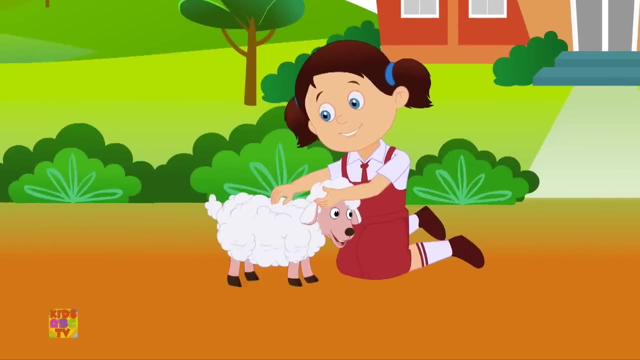 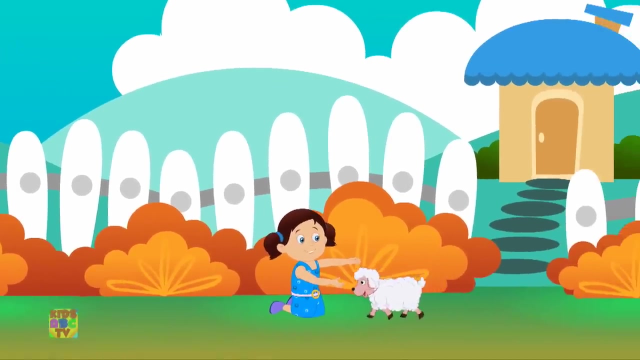 Love Mary. so Why does the lamb love Mary? so The eager children cried, Why Mary loves the lamb. you know The lamb, you know The lamb, you know Why Mary loves the lamb, you know The teacher did reply. The teacher did reply: Mary had a little lamb, Little lamb. 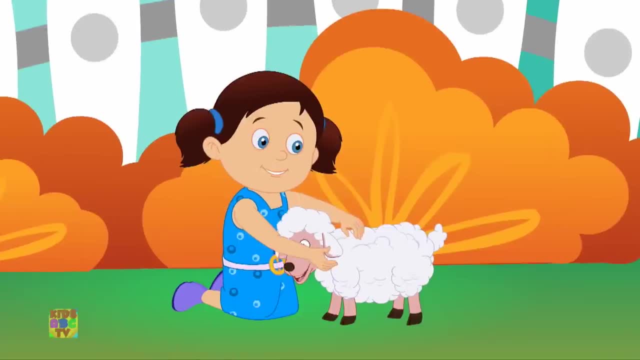 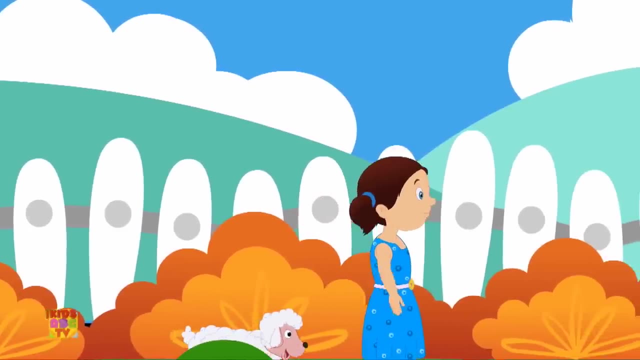 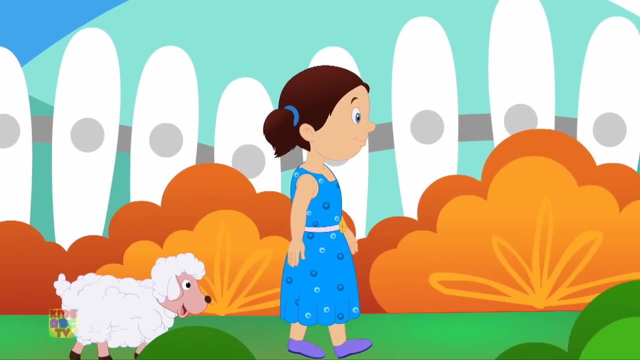 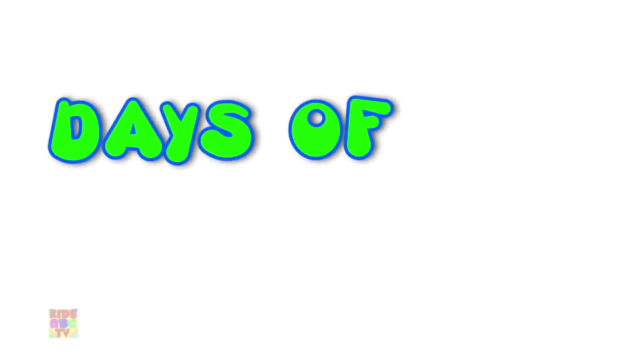 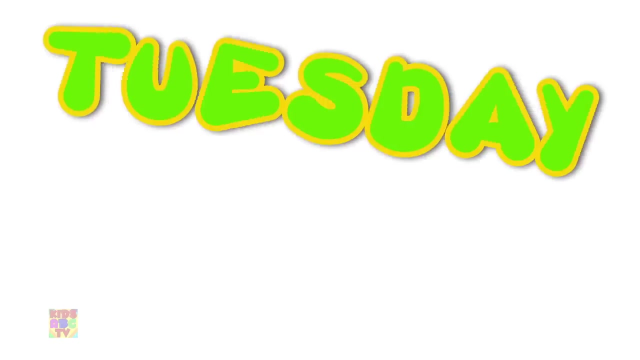 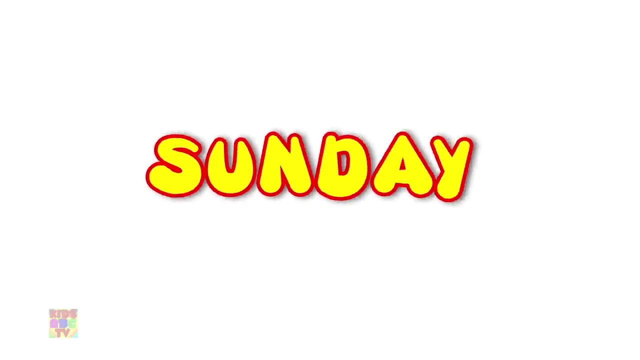 Little lamb. Mary had a little lamb. Its fleece was white as snow, And everywhere that Mary went, Mary went, Mary went, And everywhere that Mary went, The lamb was sure to go. Sunday, Monday, Tuesday, Wednesday, Thursday, Friday, Saturday, And it's Sunday once again- Sunday Monday. 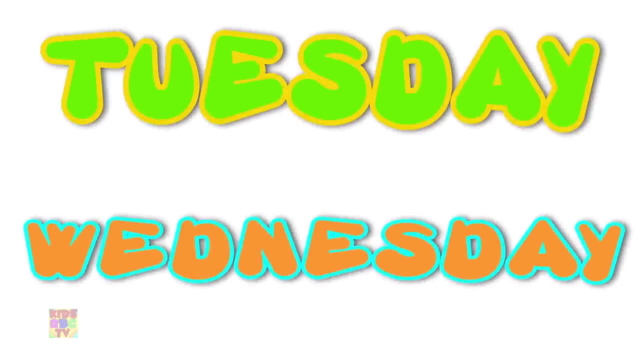 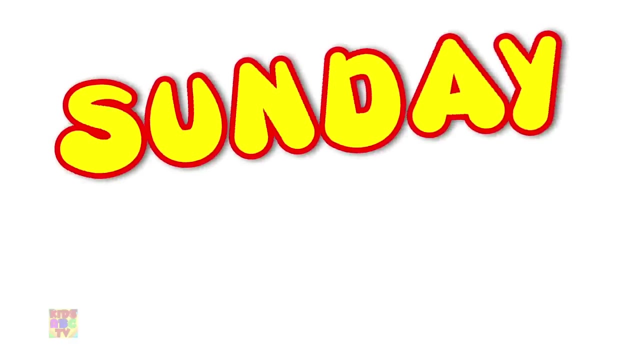 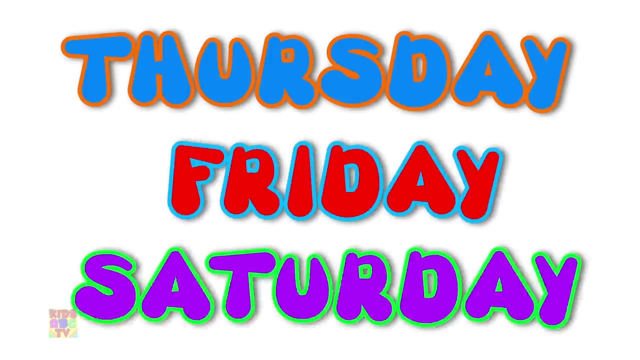 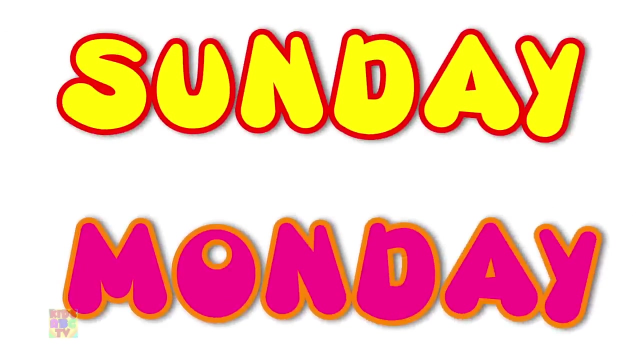 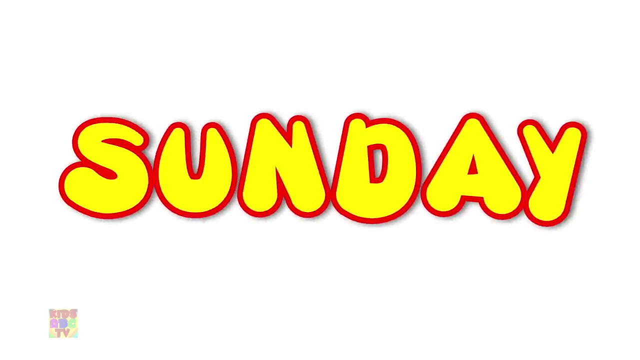 Tuesday, Wednesday, Thursday, Monday, Sunday, And it's Sunday once again. Sunday, Monday, Tuesday, Wednesday, Thursday, Friday, Saturday, And it's Sunday once again. Sunday, Monday, Tuesday, Wednesday, Thursday, Friday, Sunday, And it's Sunday once again. These are the days of the week. 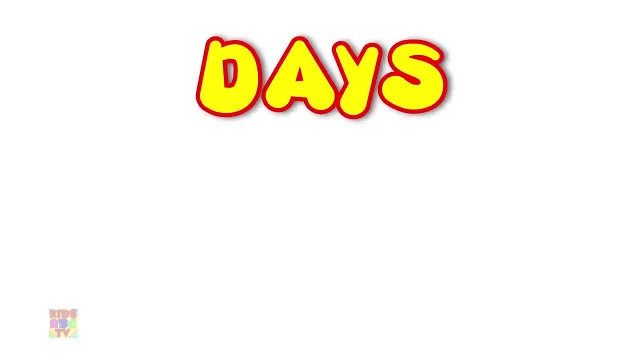 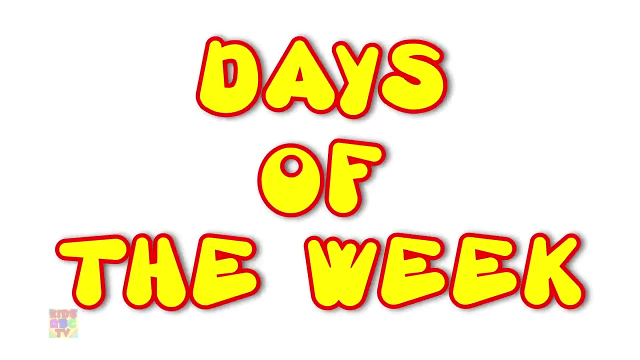 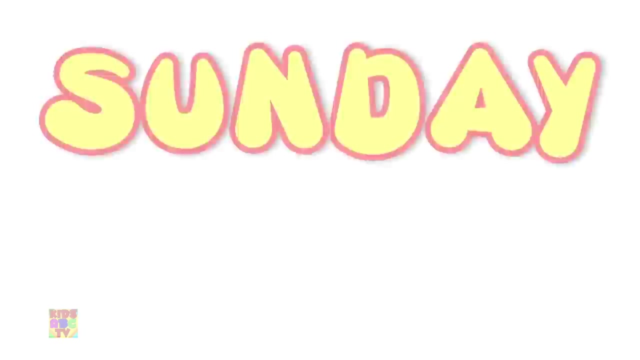 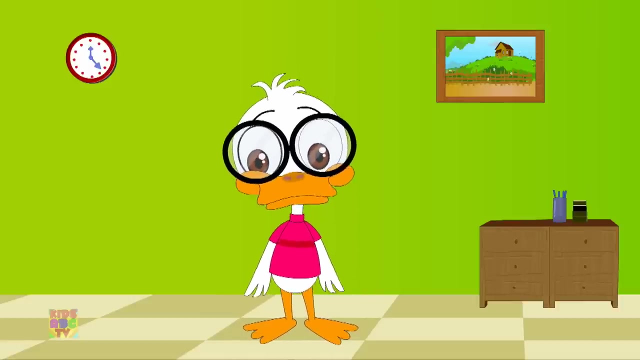 These are the days of the week. These are the days of the week, And seven days there are. These are the days of the week. These are the days of the week. These are the days of the week, And seven days there are: Sunday, Monday, Goosey goosey gander. 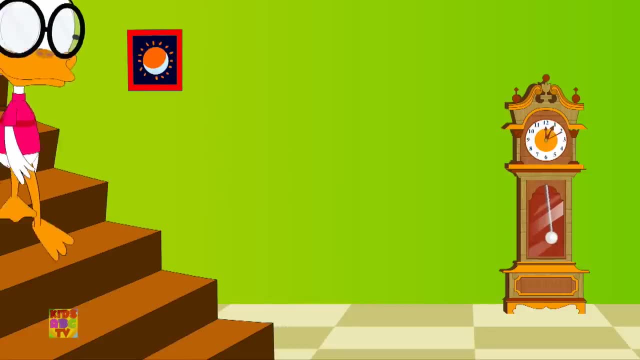 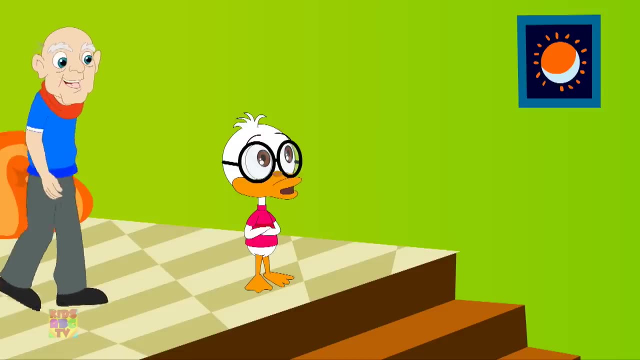 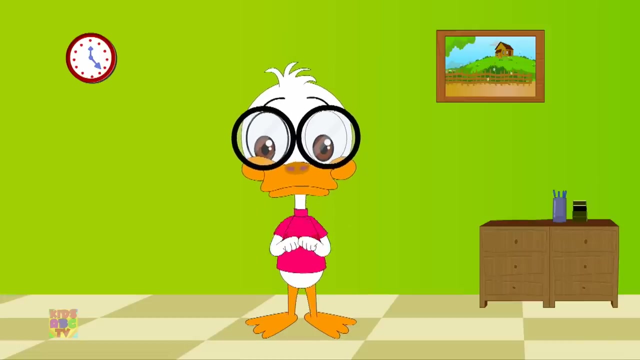 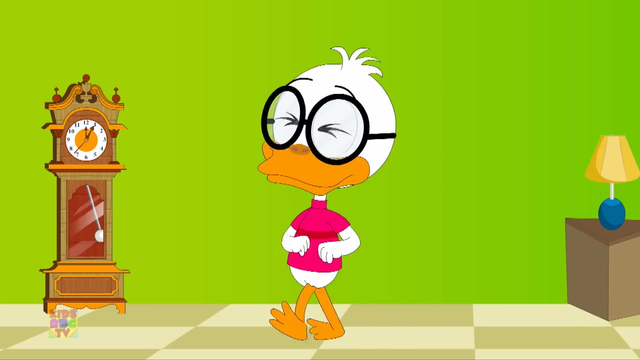 Whither, shall I wander? Upstairs and downstairs And in my lady's chamber. There I met an old man Who would not say his prayers. I took him by the left leg And threw him down the stairs. Goosey, goosey, gander. Whither, shall I wander? 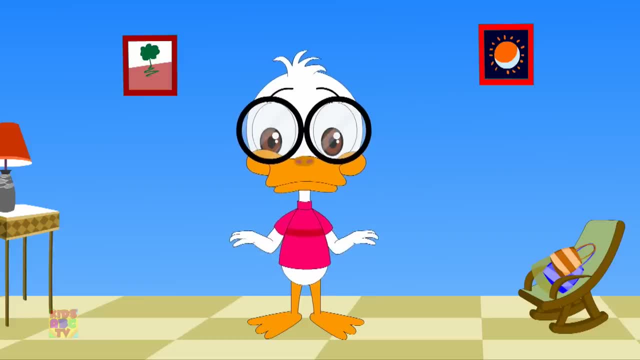 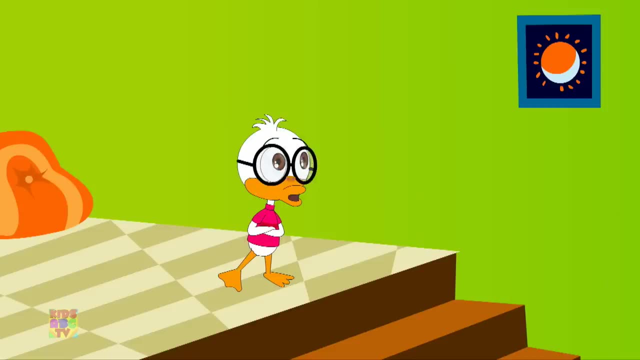 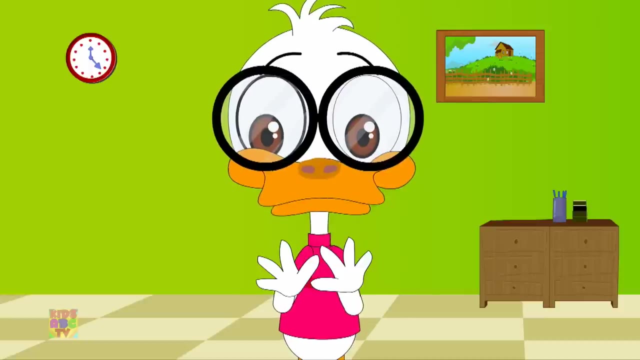 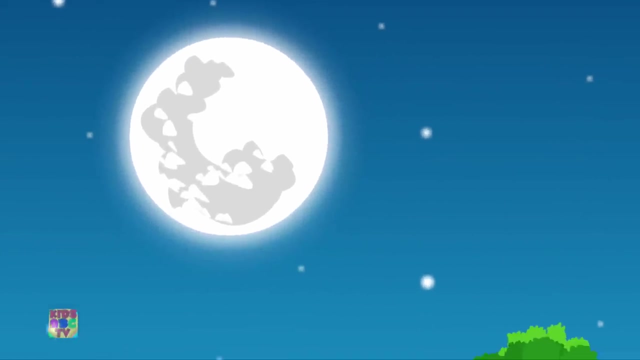 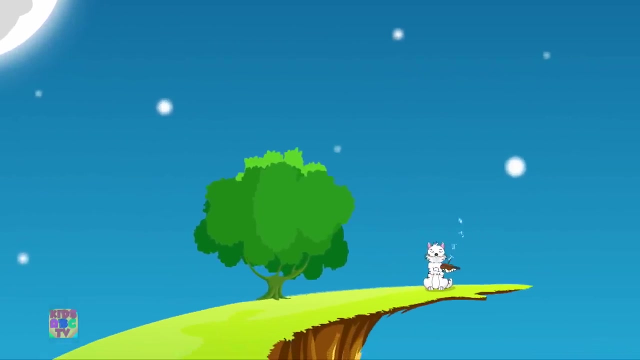 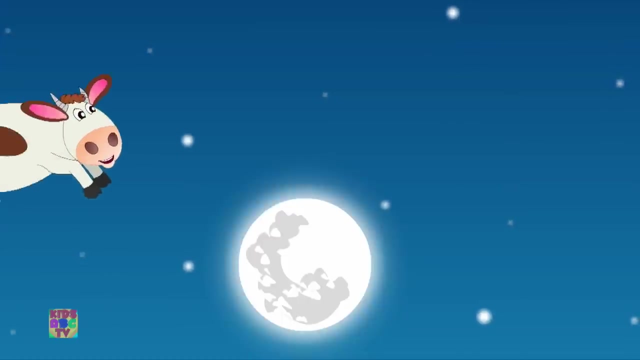 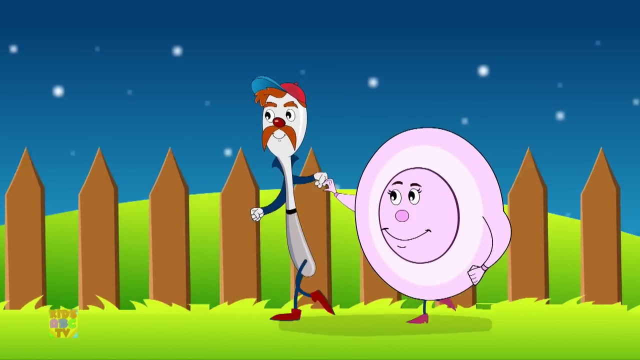 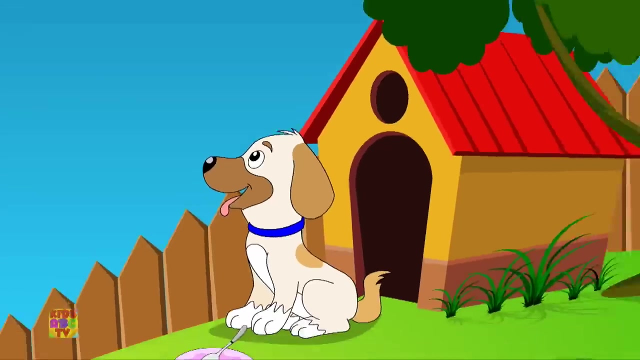 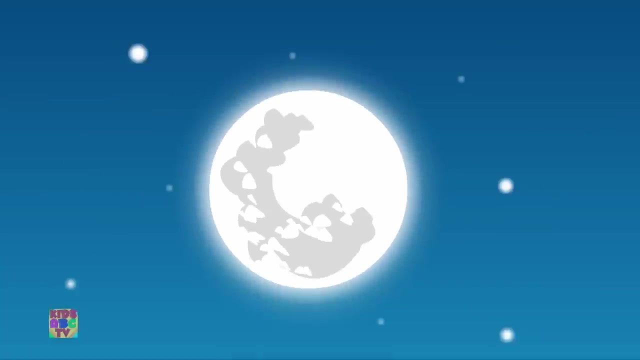 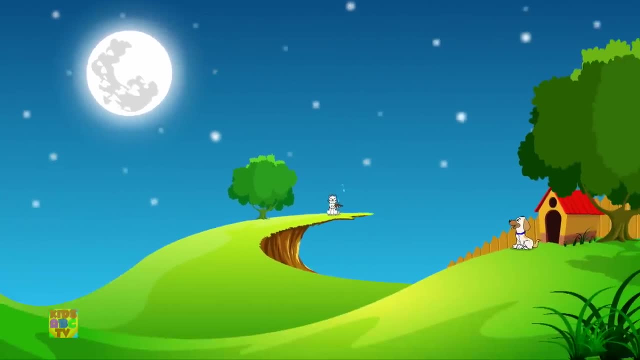 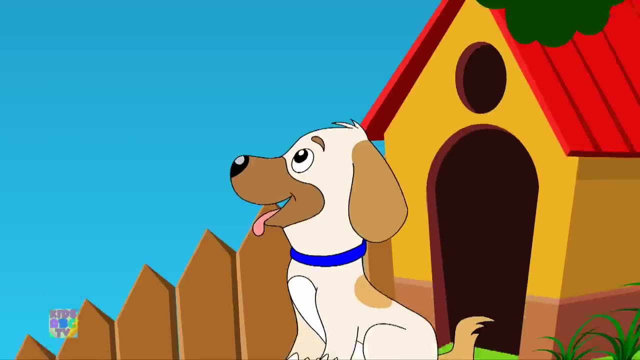 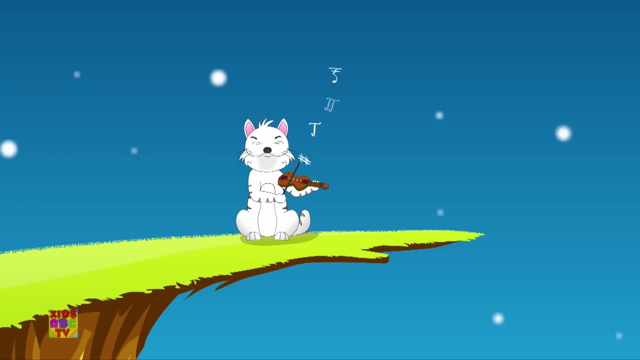 Oh, what a wonderful sight, Isn't that amazing? Hey diddle diddle, the cat and the fiddle The cow jumped over the moon. The little dog laughed to see such fun And the dish ran away with the spoon. Hey diddle diddle, the cat and the fiddle The cow jumped over the moon. 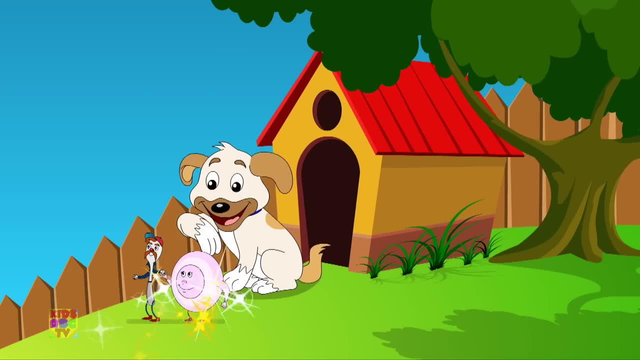 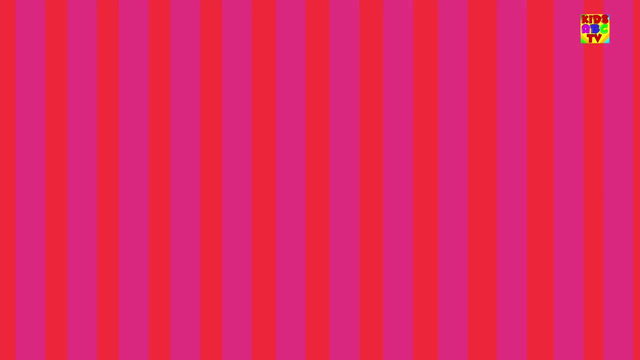 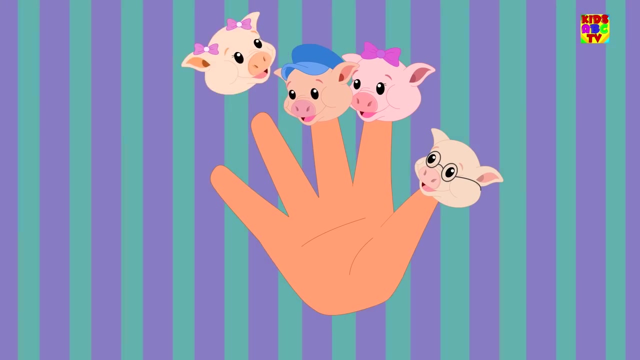 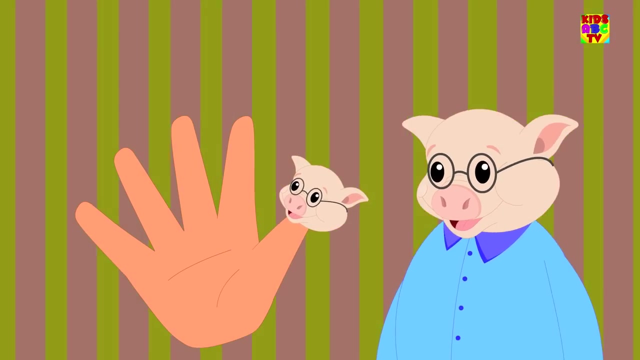 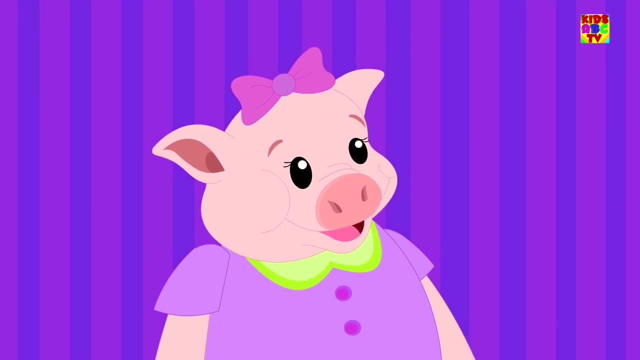 The little dog laughed to see such fun And the dish ran away with the spoon. Daddy Finger, Daddy Finger, where are you Here? I am here, I am. how do you do? Mommy Finger, Mommy Finger, where are you Here? I am here, I am, how do you do. 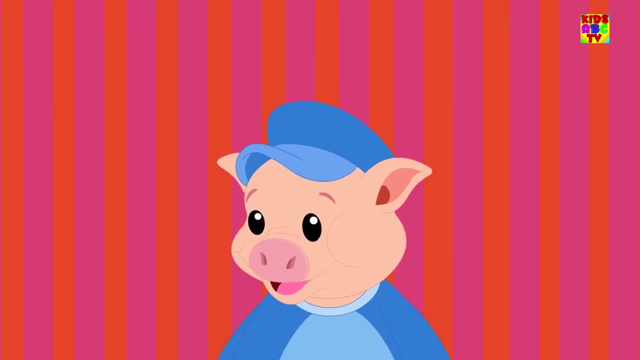 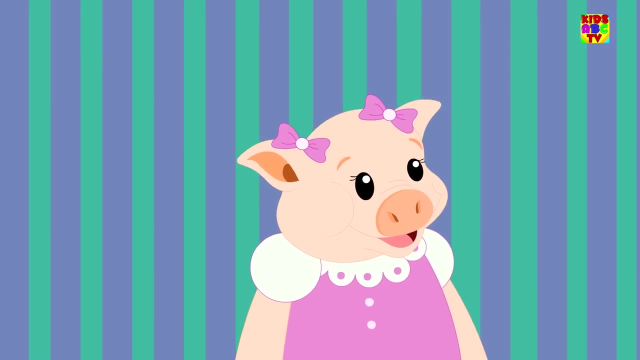 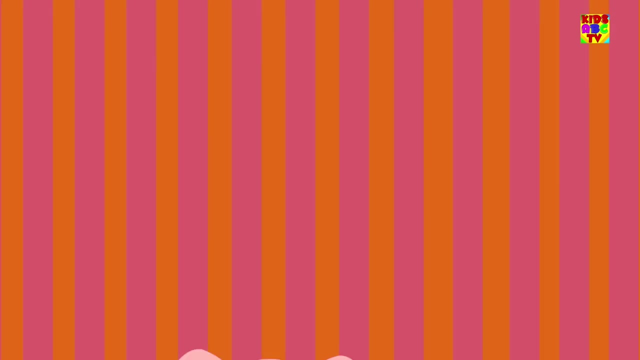 Brother Finger, Brother Finger, where are you Here? I am here, I am. how do you do Sister Finger? Sister Finger, where are you Here? I am here, I am. how do you do Baby Finger, Baby Finger, where are you Here? I am here, I am. how do you do? 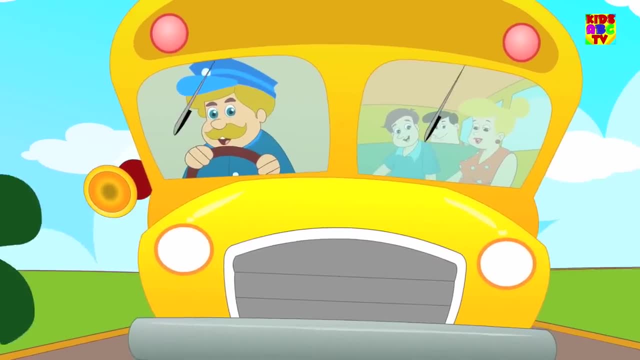 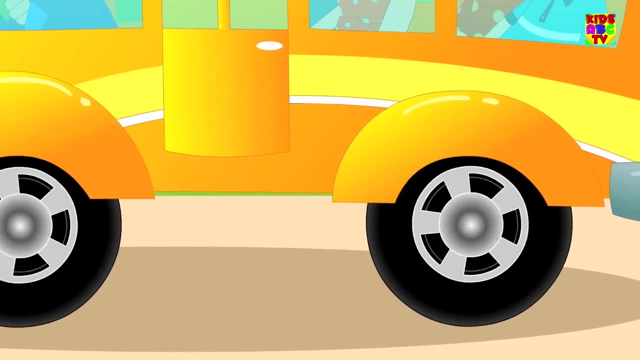 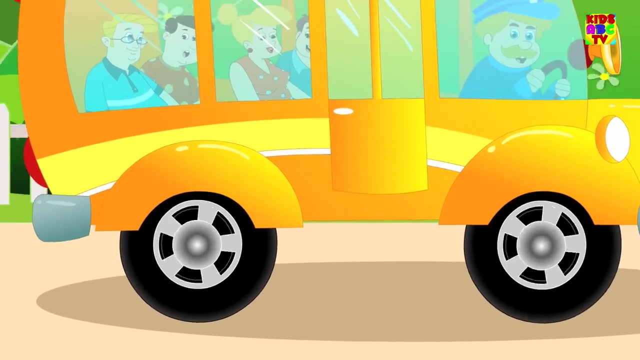 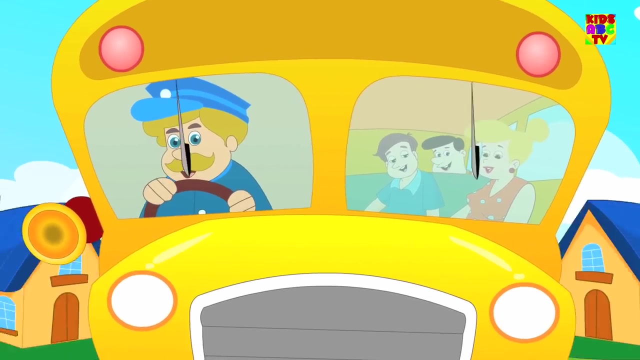 Hey diddle diddle the cat and the fiddle The cow jumped over the moon. Hey diddle diddle the cat and the fiddle The cow jumped over the moon And the dish ran away with the spoon. SHE SAYS NOOOO. 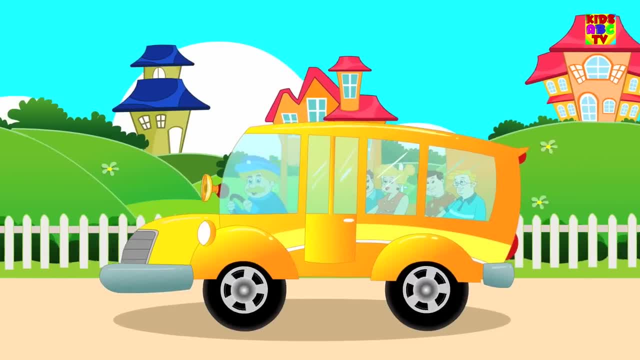 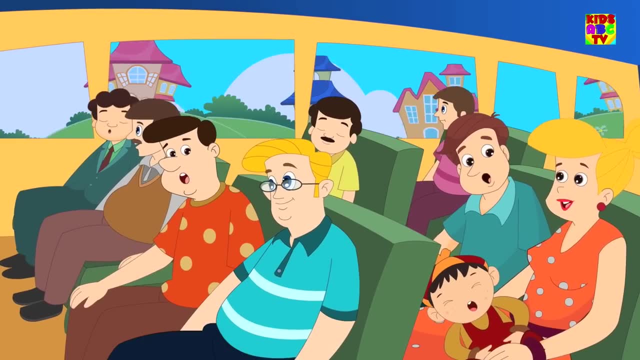 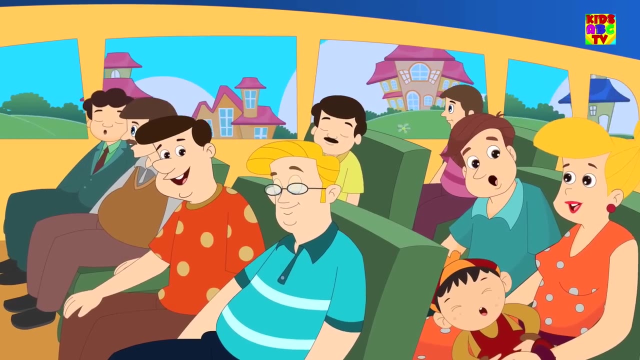 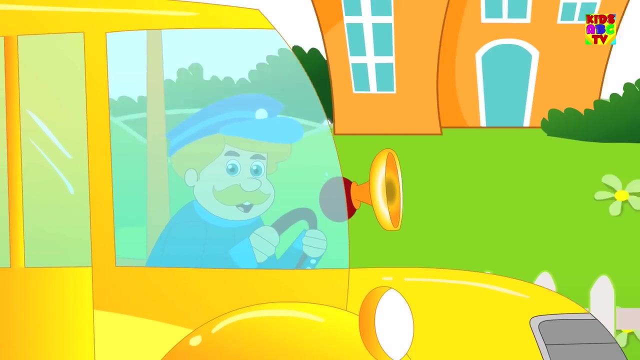 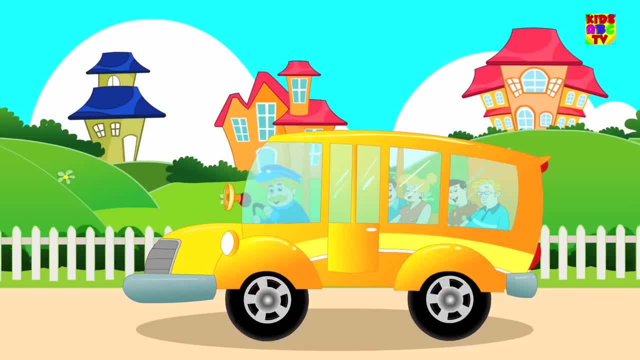 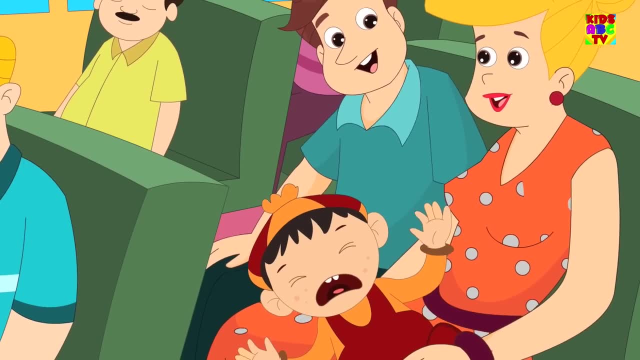 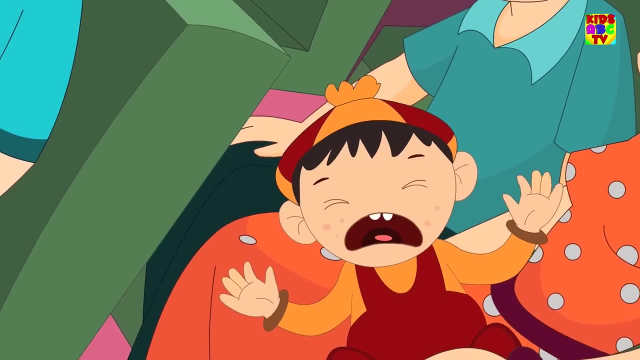 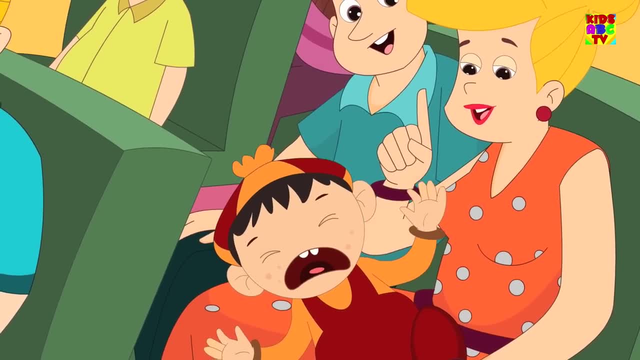 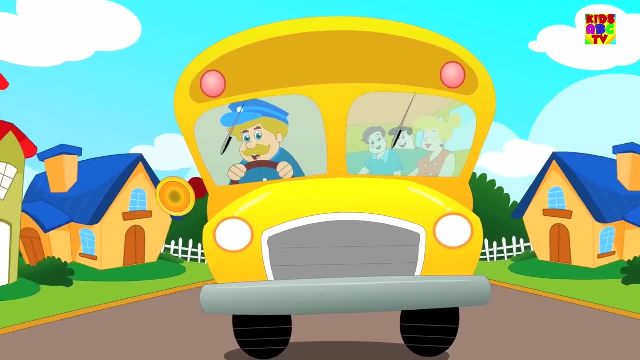 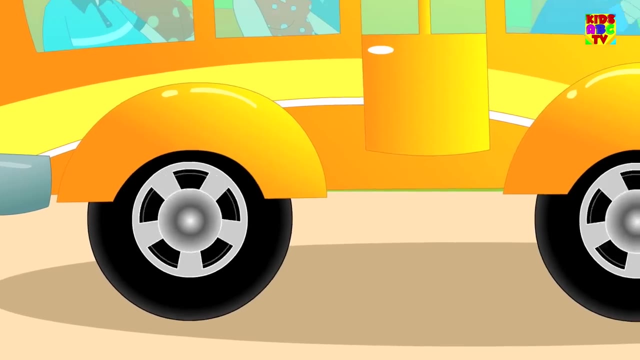 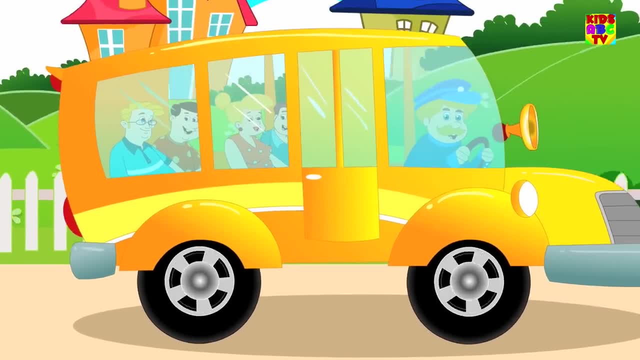 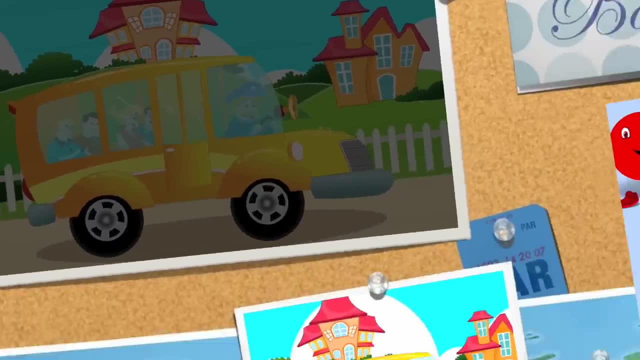 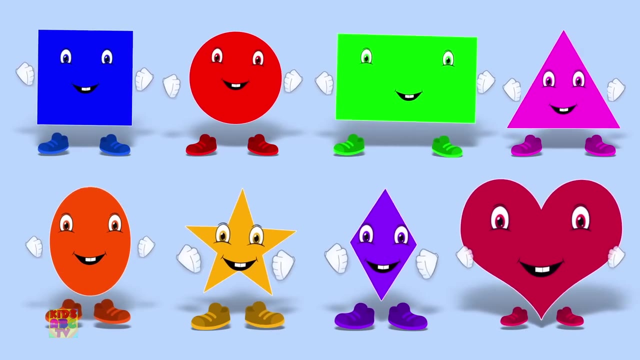 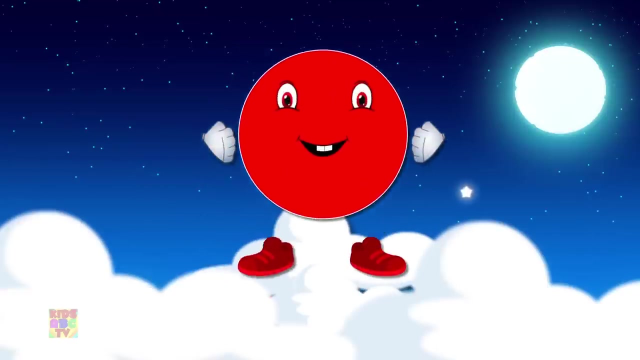 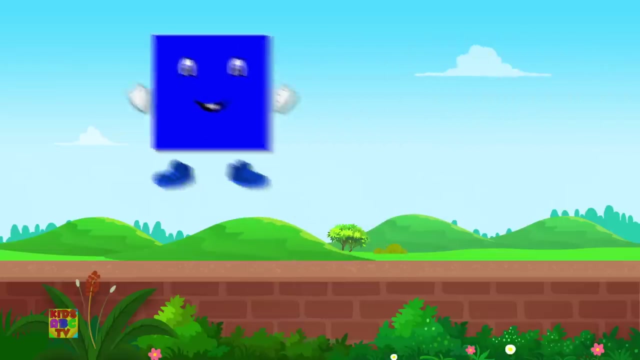 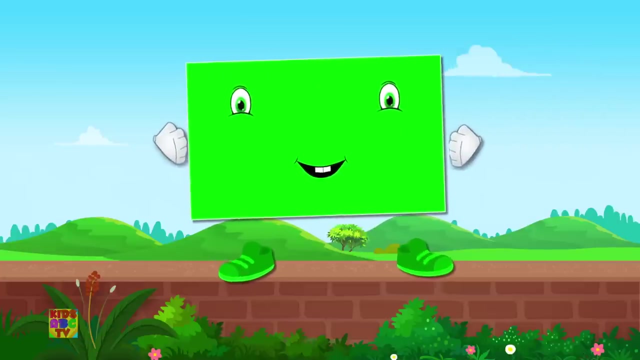 and round, round and round, round and round, round and round. The wheels on the bus go round and round all through the town. Let's have fun with shapes. Alright, let's go. Square Circle- Rectangle Triangle. Square Circle, Rectangle Triangle. 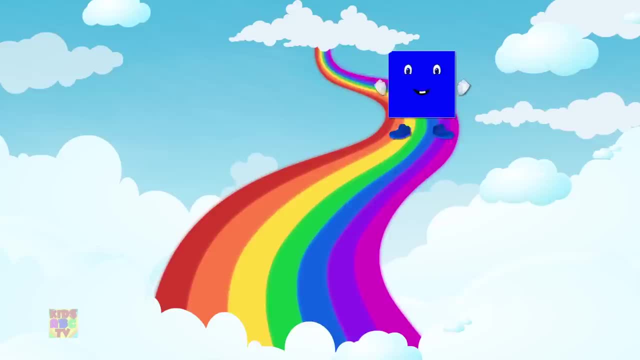 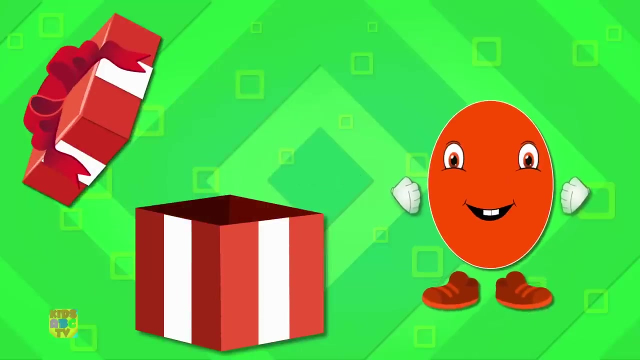 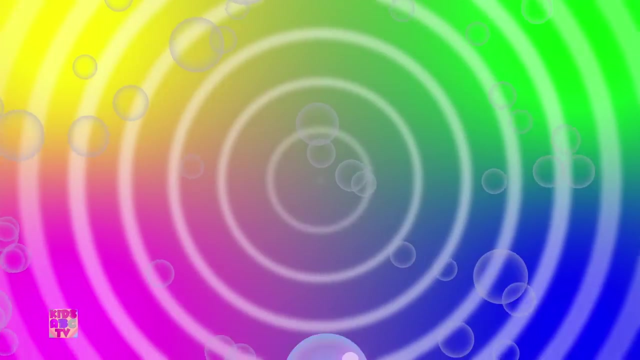 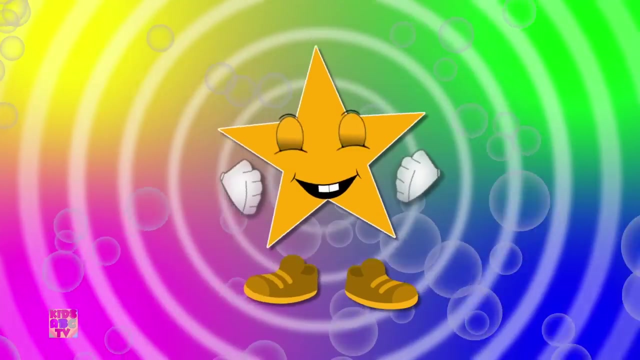 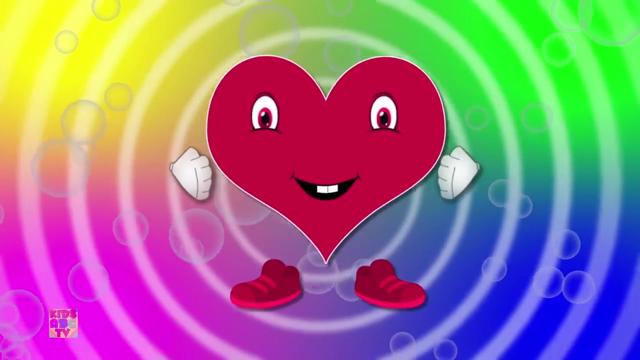 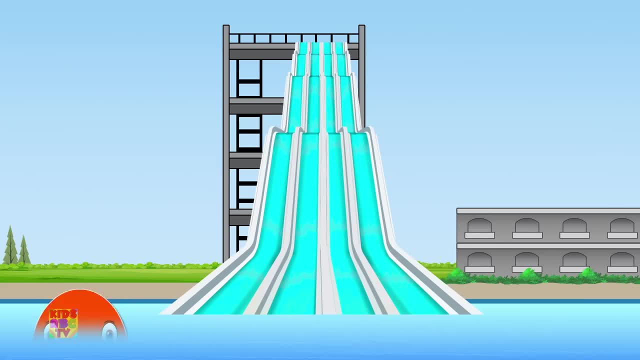 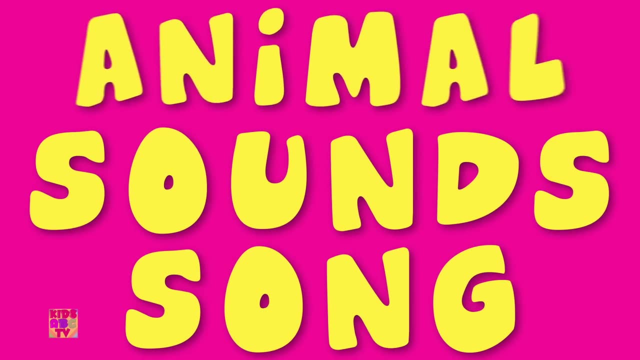 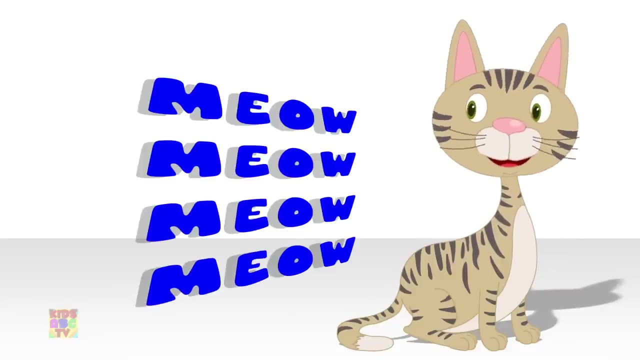 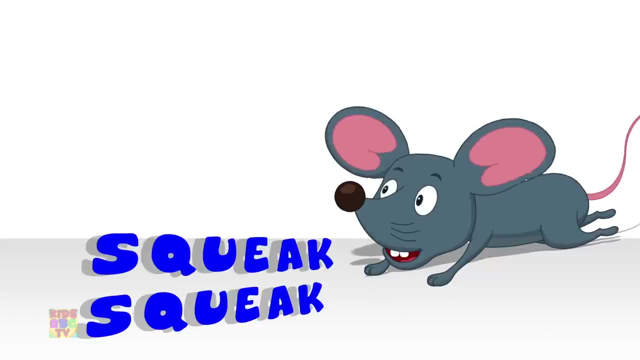 Oval Star, Diamond, Heart. Aren't these shapes lovely too? The cat goes meow, meow, meow, meow. The dog goes woof, woof, woof, woof. Mouse goes squeak, squeak, squeak, squeak and the fly goes buzz, buzz, buzz. 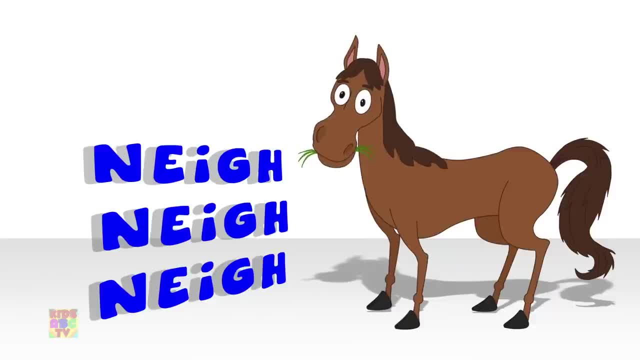 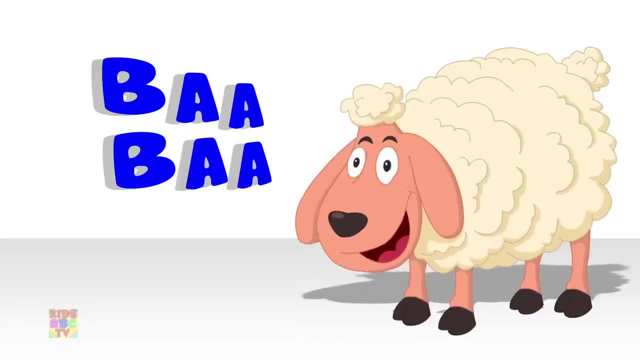 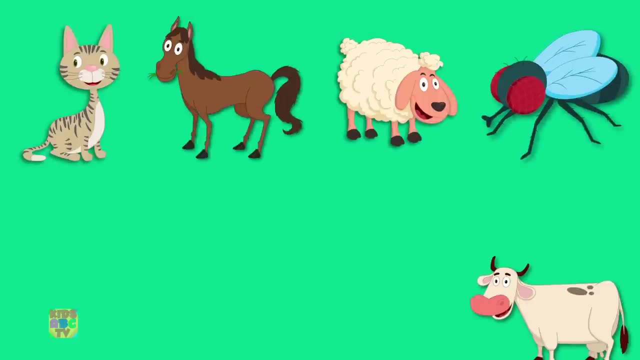 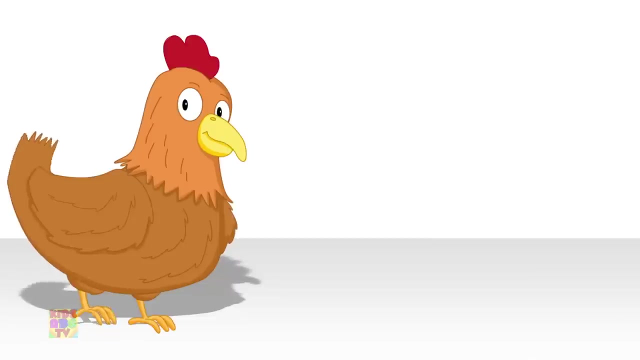 The horse goes nay, nay, nay, nay. the pig goes oink, oink, oink, oink. The sheep goes bah, bah, bah, bah, and the cow goes moo, moo, moo. These are the animal sounds. These are the animal sounds. The hen goes cluck, cluck, cluck, cluck. the duck goes quack. 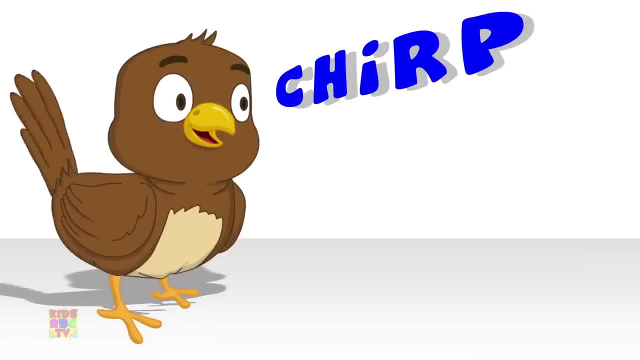 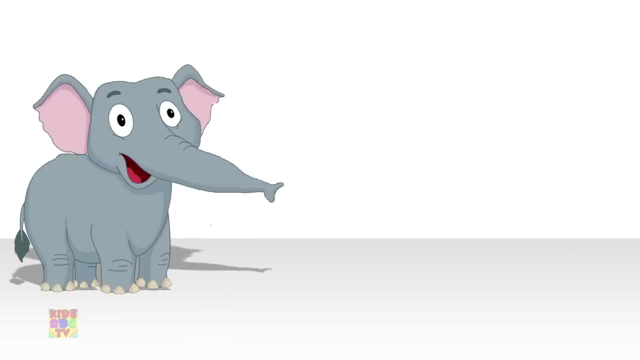 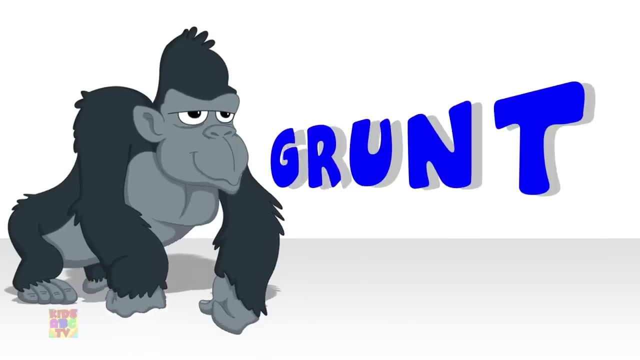 quack, quack, quack. the sparrow goes chirp, chirp, chirp, chirp, and the turkey goes gobble, gobble, gobble. The elephant goes trumpet, trumpet, trumpet, trumpet. the gorilla goes grunt, grunt, grunt, grunt. The hippopotamus rumbles, Rumble, rumble, rumble. 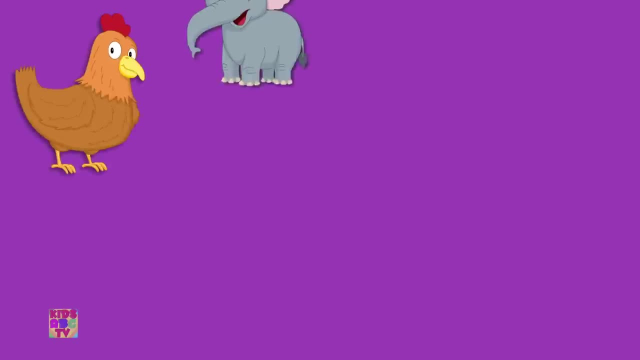 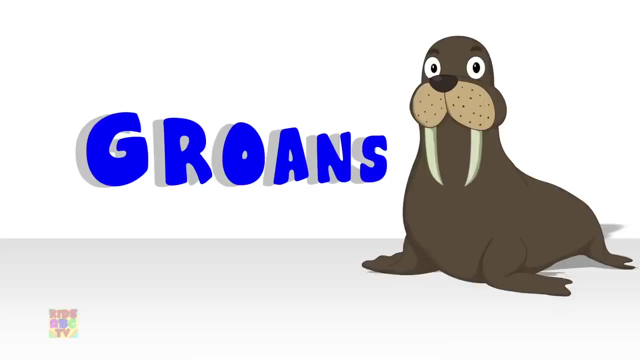 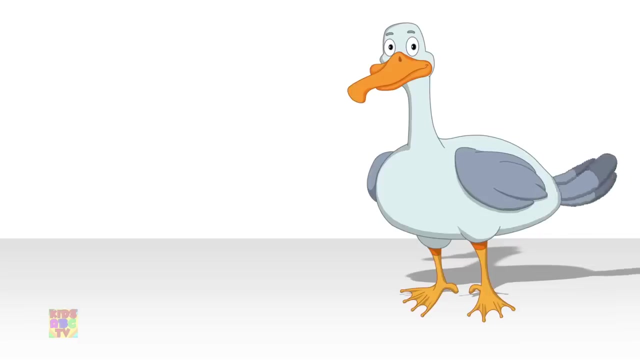 And the lion goes roar, roar, roar. These are the animal sounds. These are the animal sounds. The whales, they sing, sing, sing, sing. The walrus groans, groan, groan, groan. The seals go bark, bark, bark, bark. And the seagull goes squawk, squawk, squawk. 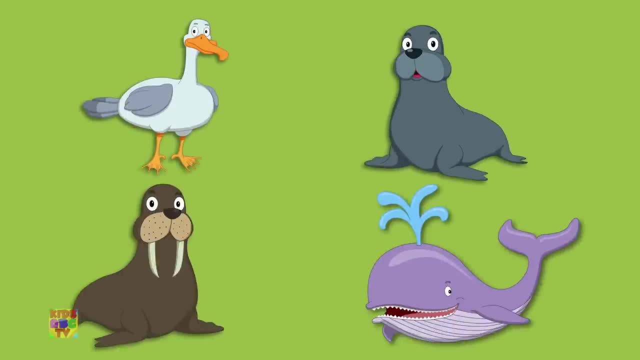 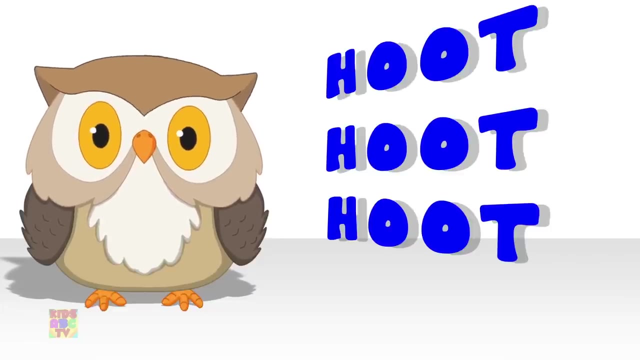 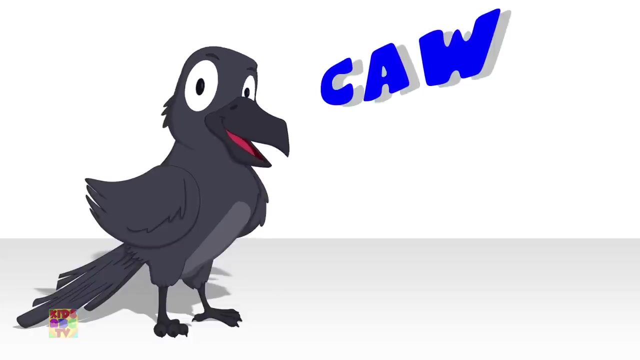 These are the animal sounds. These are the animal sounds. The owl goes hoot hoot, hoot, hoot. The parrot goes screech, screech, screech, screech. The crow goes caw caw, caw, caw. And the cuckoo goes coo coo, coo, coo. 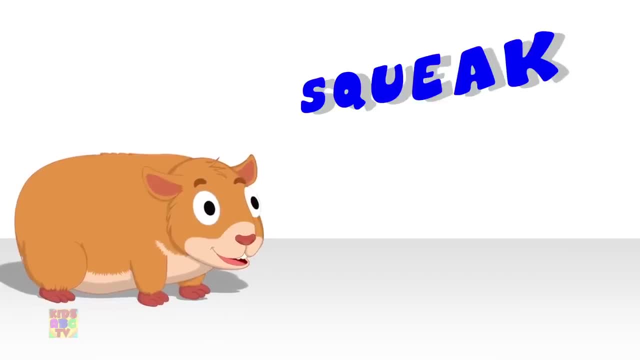 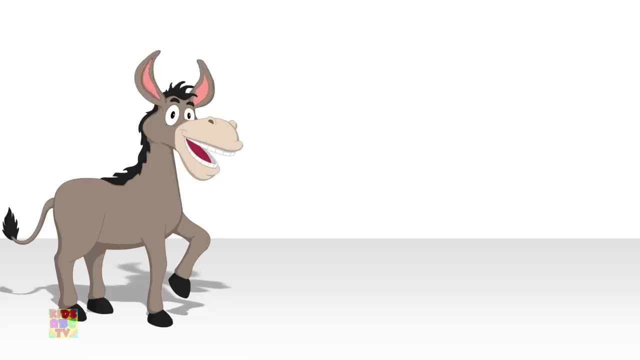 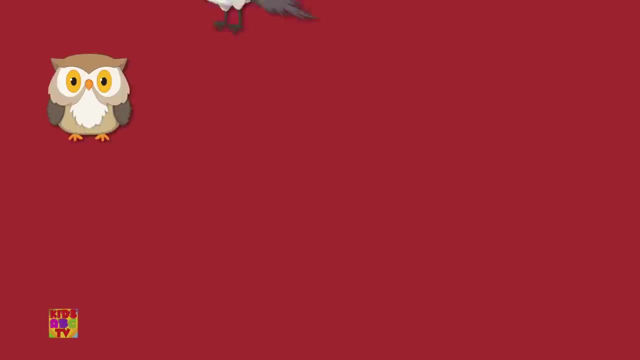 The hamster goes squeak, squeak, squeak, squeak. The hog goes grunt, grunt, grunt, grunt. The donkey goes haw haw, hee haw, And the zebra goes whinny, whinny, whinny. 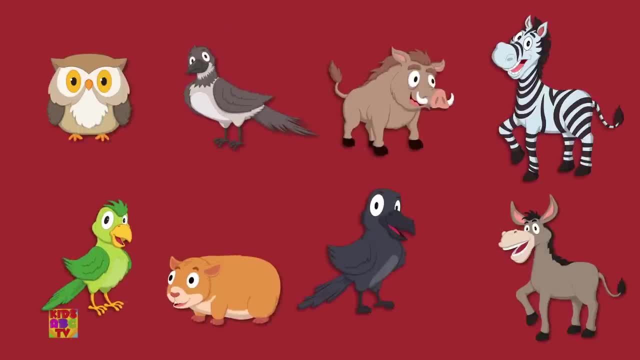 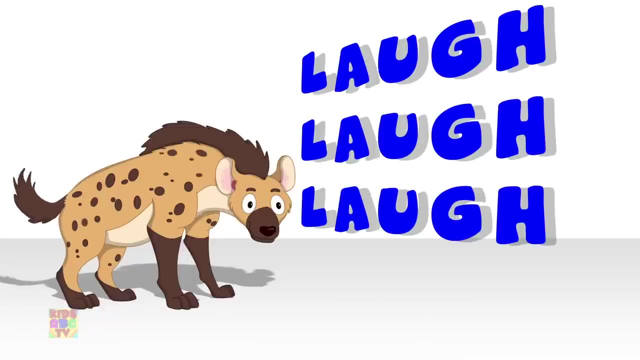 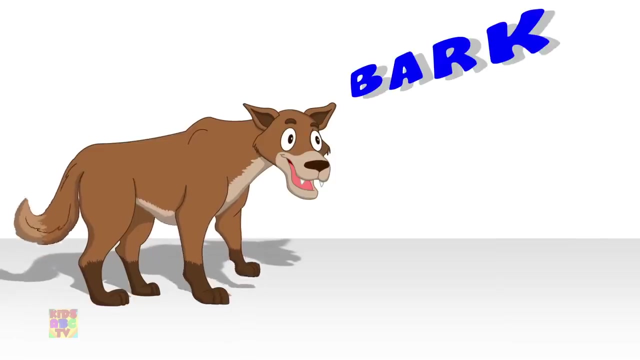 These are the animal sounds. These are the animal sounds. The hyena goes, laugh, laugh, laugh, laugh. The snake goes, hiss, hiss, hiss, hiss. The coyote goes: bark, bark, bark, bark. 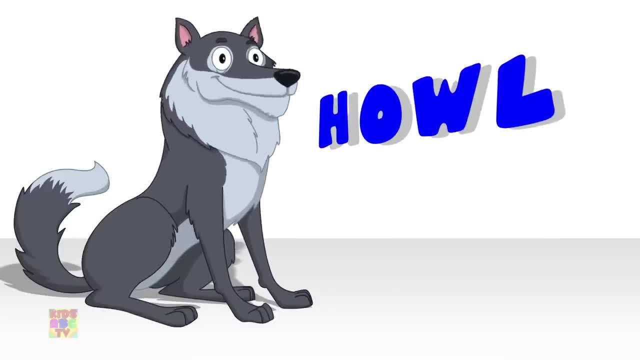 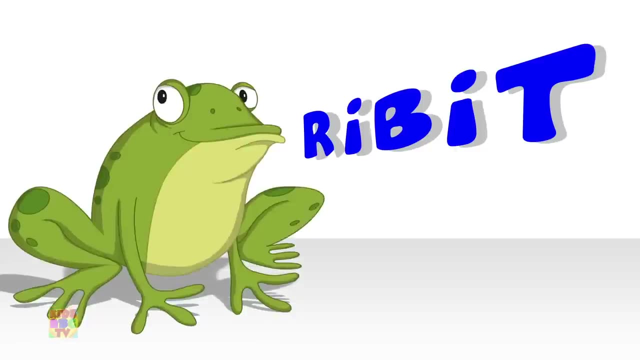 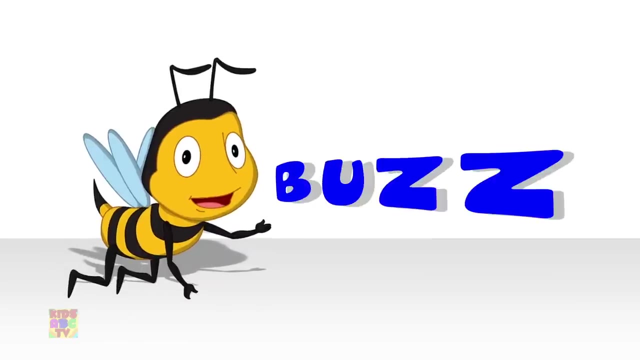 And the wolves go howl, howl, howl. The guinea pig squeaks, squeaks, squeaks, squeaks. The frog goes ribbit, ribbit, ribbit, ribbit. The squirrels go chatter, chatter, chatter, chatter, And the bees go buzz, buzz, buzz. 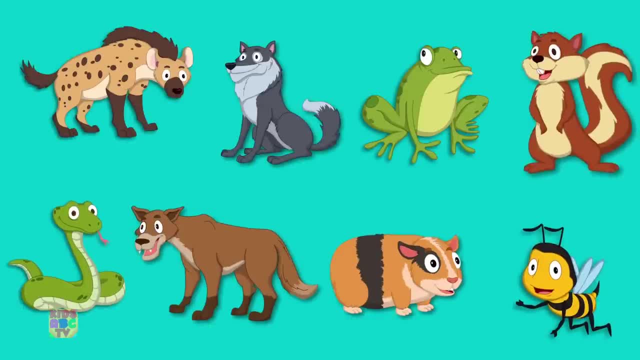 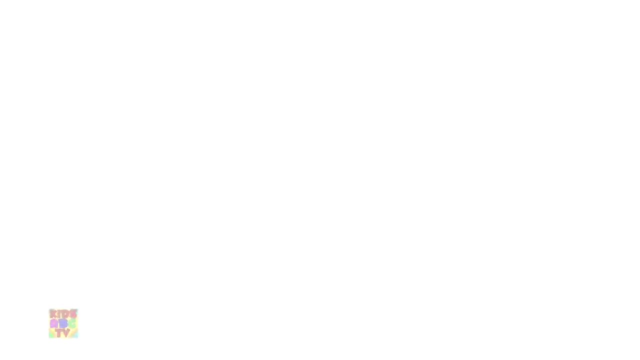 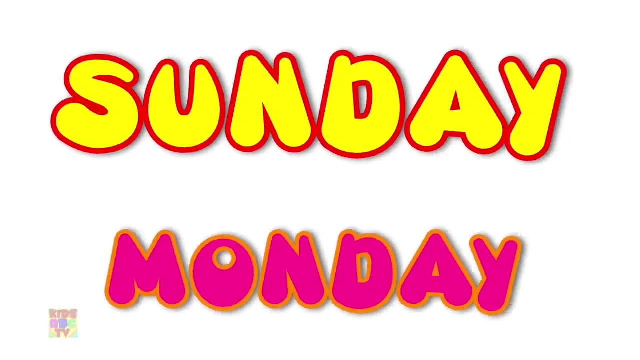 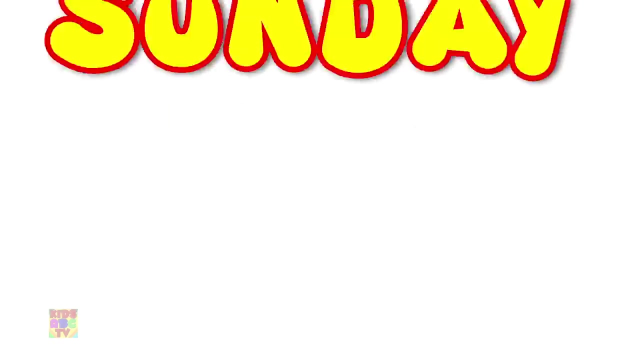 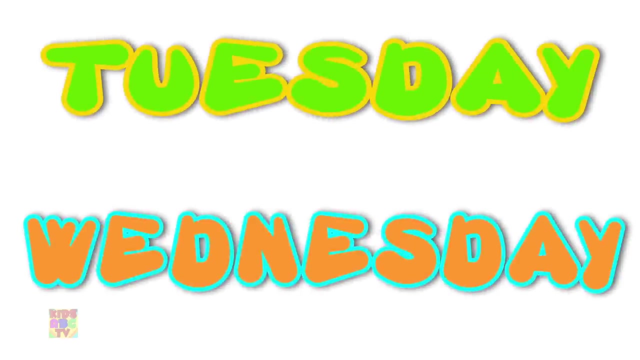 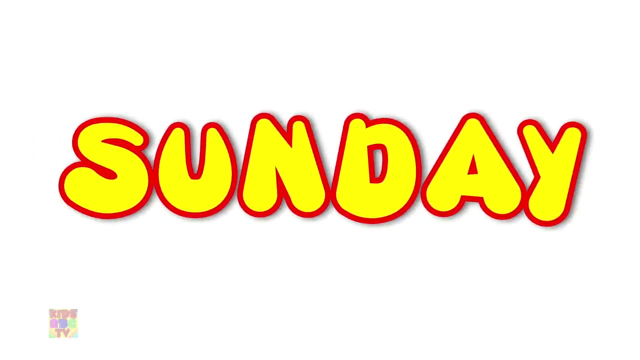 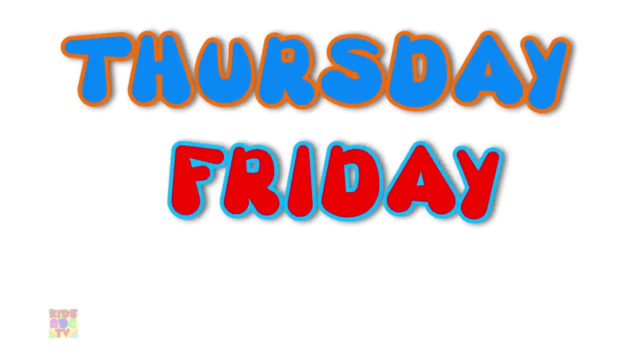 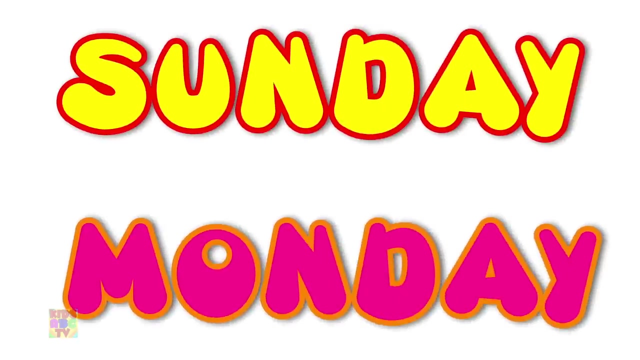 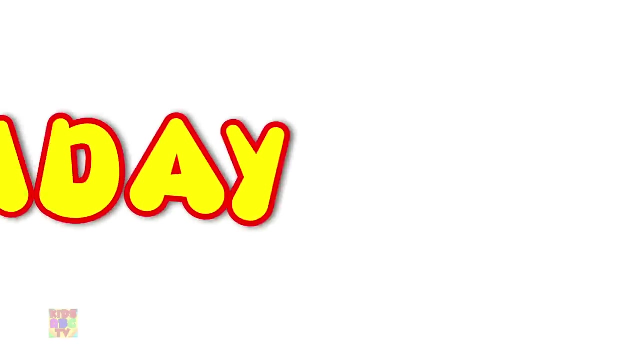 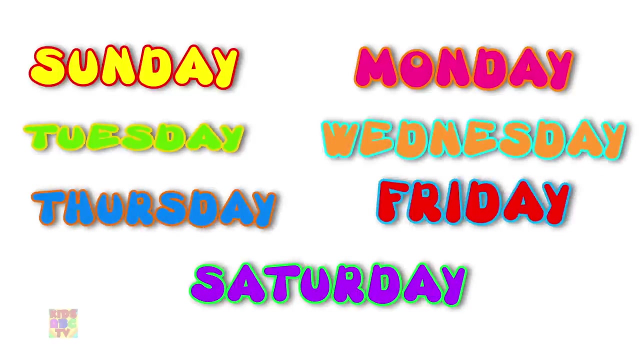 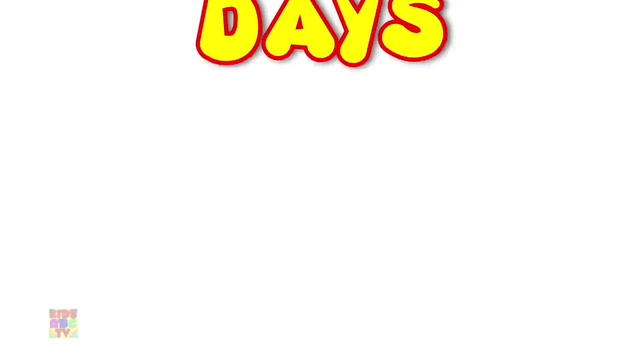 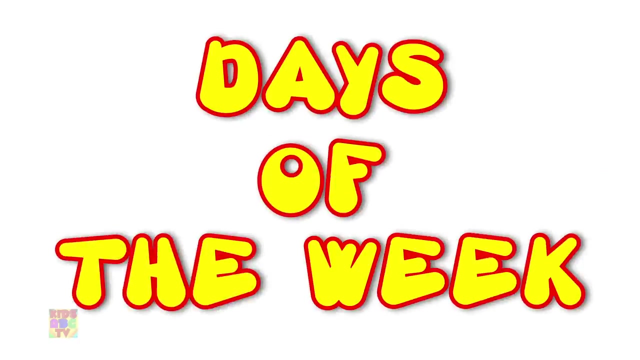 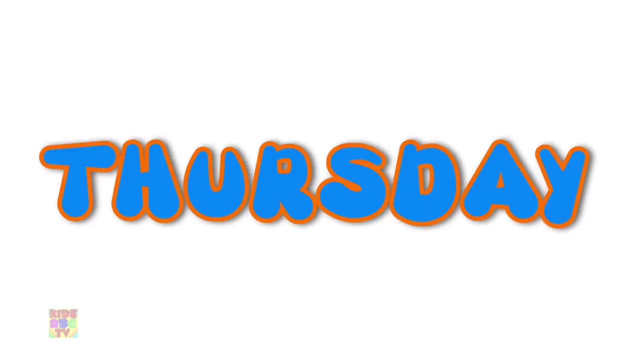 These are the animal sounds. These are the animal sounds. These are the animal sounds. 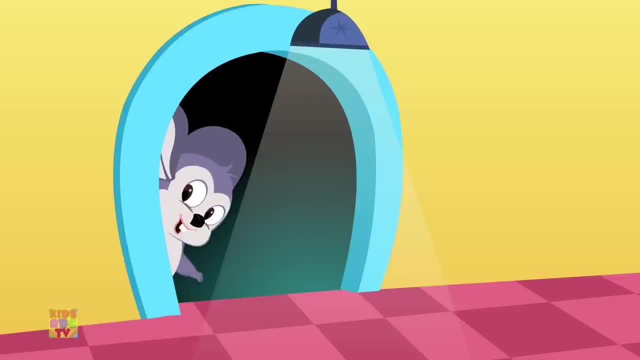 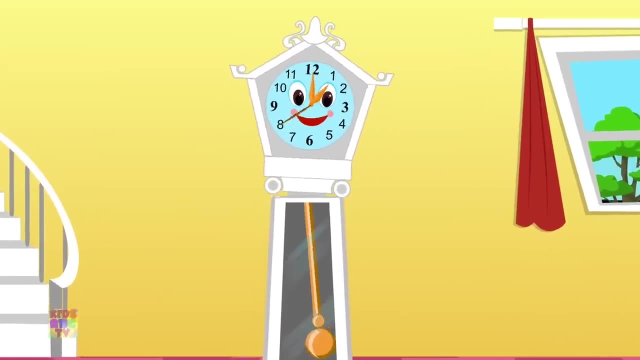 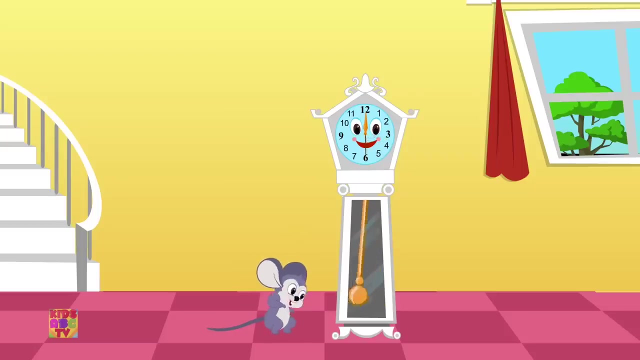 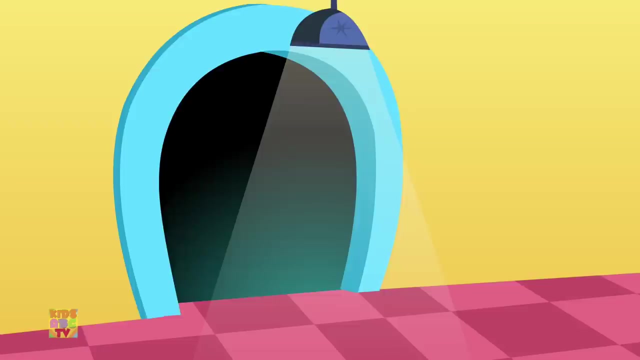 Tick, Tock, Tick, Tick, Tock, Tick, Hickory-dickory-dock, The mouse ran up the clock. The clock struck one. the mouse ran down Hickory-dickory-dock, Hickory-dickory-dock, The mouse ran up the clock. 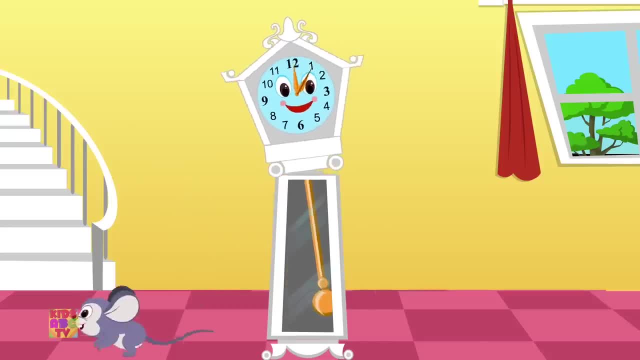 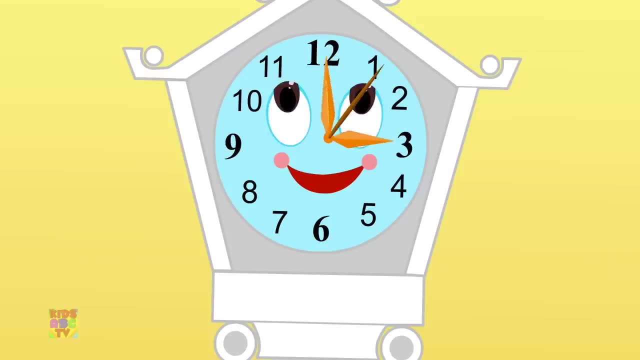 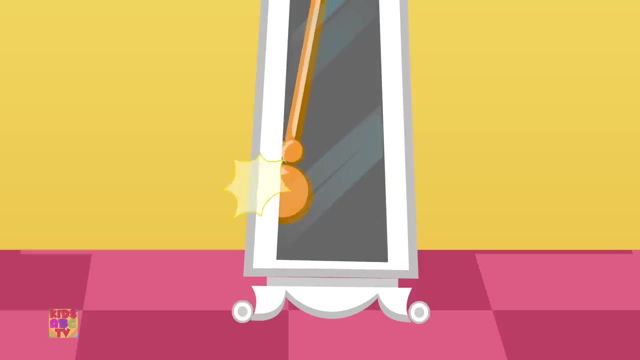 The clock struck two and down. he flew. Hickory dickory dock. Hickory dickory dock, The mouse ran up the clock. The clock struck three, and he did flee. Hickory dickory dock. Tick, tock, tick, Tick, tock, tick. Hickory dickory dock, The mouse ran up the clock. 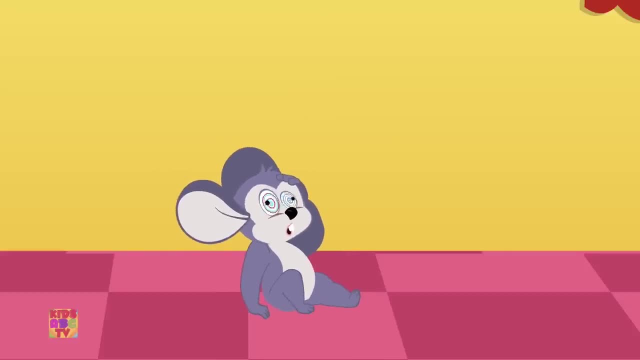 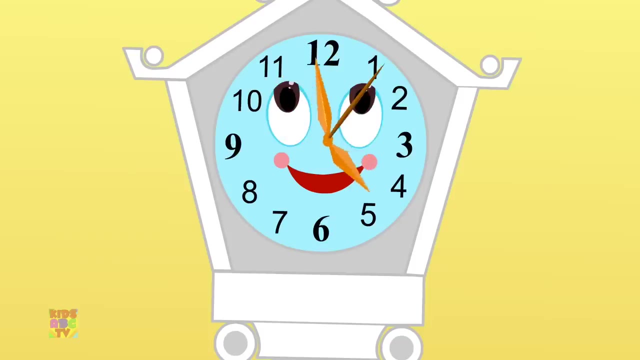 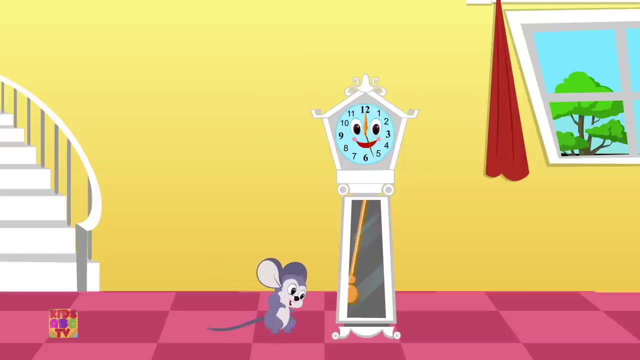 The clock struck four, he hit the floor. Hickory dickory dock. Hickory dickory dock. The mouse ran up the clock. The clock struck five. the mouse took a dive. Hickory dickory dock. Hickory dickory dock. The mouse ran up the clock. The clock struck six. that mouse, he split. 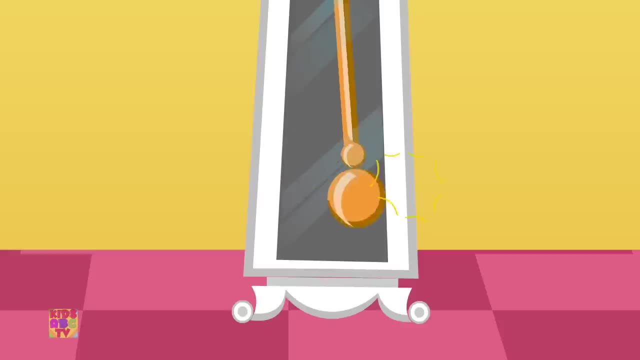 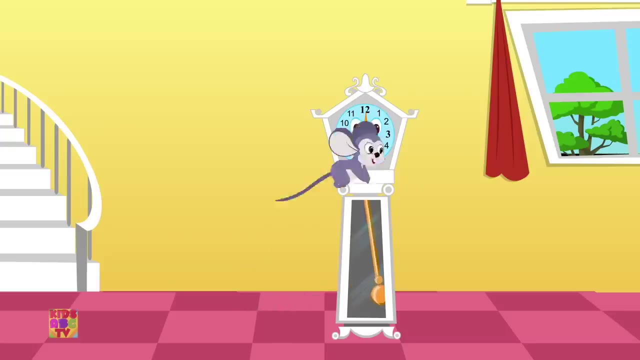 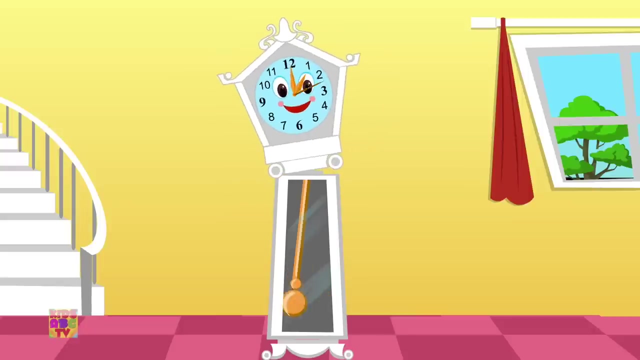 Hickory dickory dock. Tick, tock, tick, Tick, tock, tick. Hickory dickory dock. The mouse ran up the clock. The clock struck four. he hit the floor. The clock struck seven, eight, nine, ten, eleven. Hickory dickory dock. Hickory dickory dock. The mouse ran up the clock. 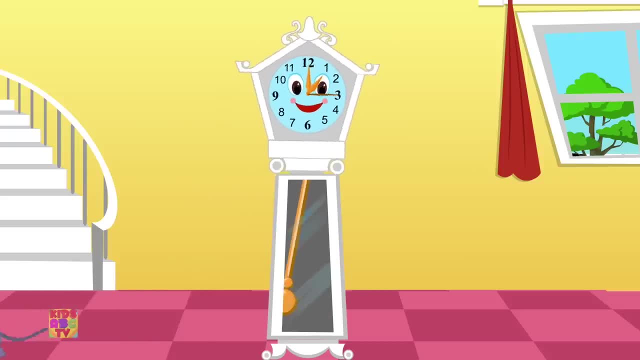 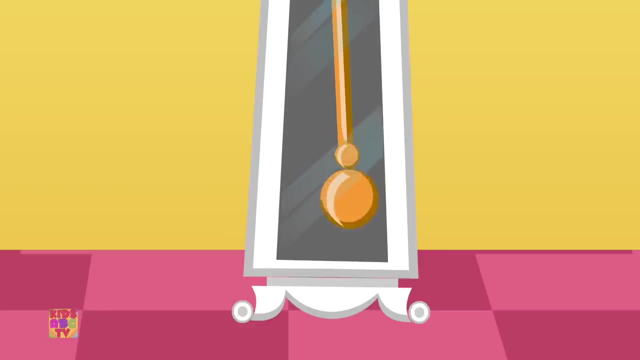 As twelve bells rang the mouse he sprang. Hickory dickory dock. Hickory dickory dock. White scamper asked the clock. You scare me, so I have to go. Hickory dickory dock. Tick, tock, tick, Tick, tock, tick. Hickory dickory dock. 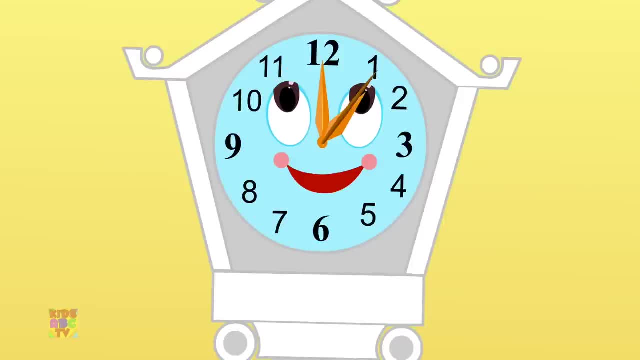 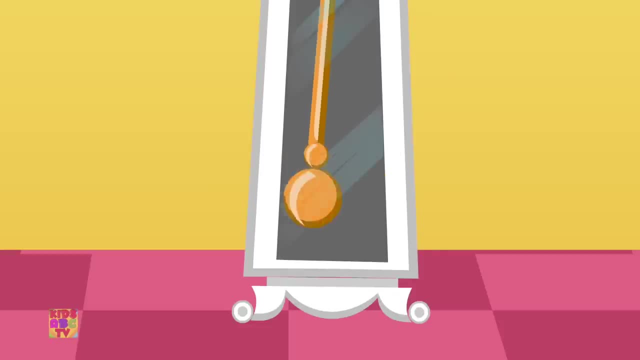 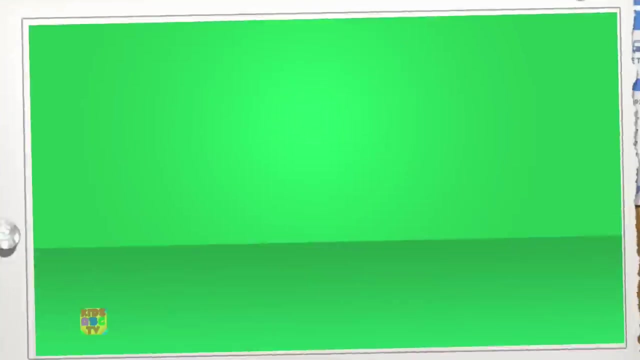 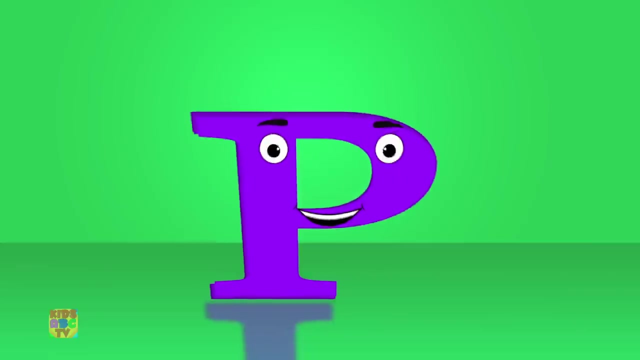 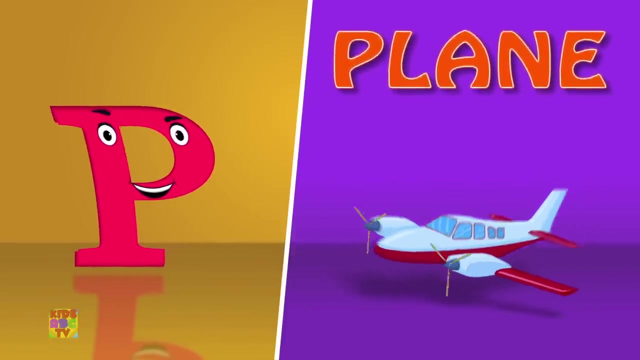 Hickory dickory dock. The mouse ran up the clock. The clock struck one, the mouse ran down. Hickory dickory dock. Here comes the letter P. P is for Plain Puh Puh. Plain. P is for Paint, Puh, Puh, Paint. P is for Paper. 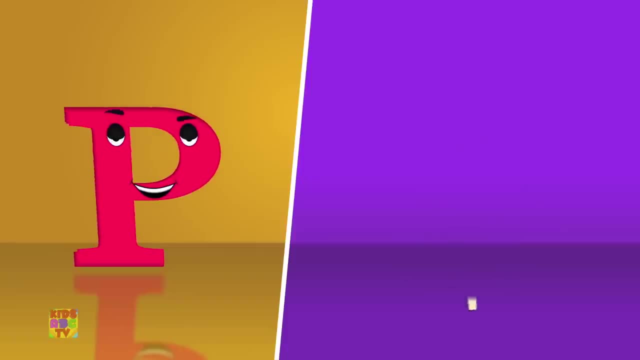 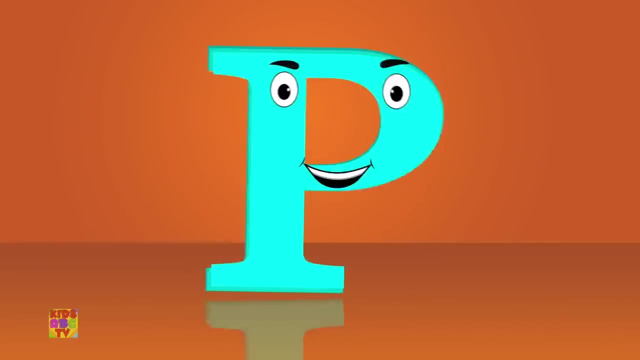 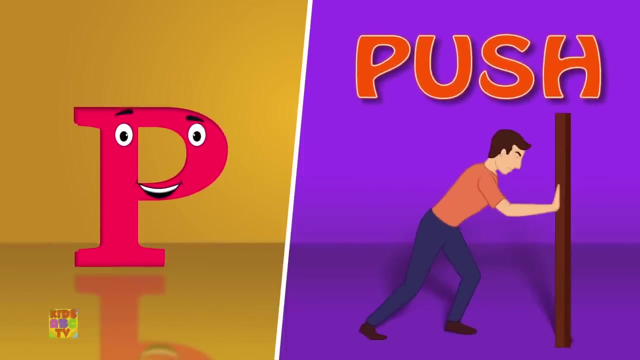 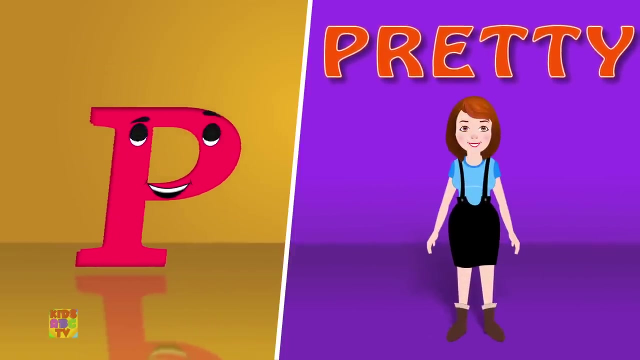 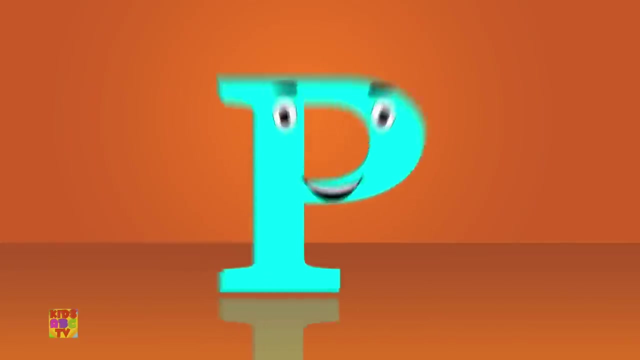 Puh Puh. Paper P is for Picture Puh Puh, Picture Puh Puh. Picture P is for Pull Puh Puh. Pull P is for Push Puh Puh. Push P is for Pretty Puh Puh. Push P is for Please Puh Puh, Please. 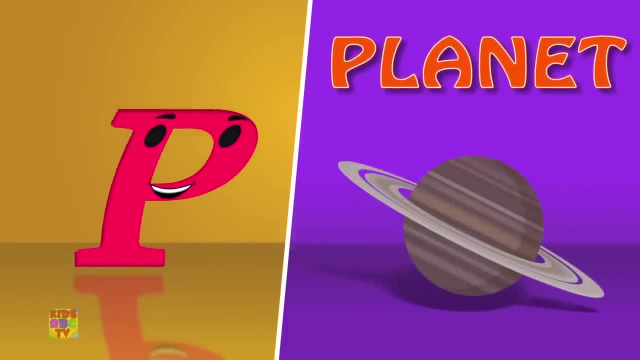 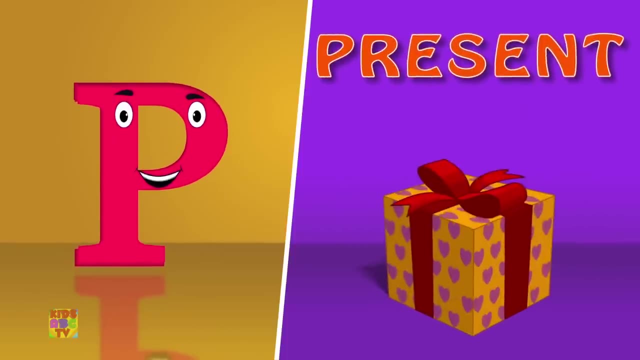 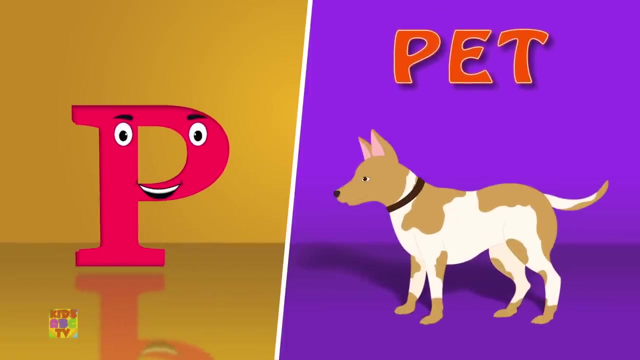 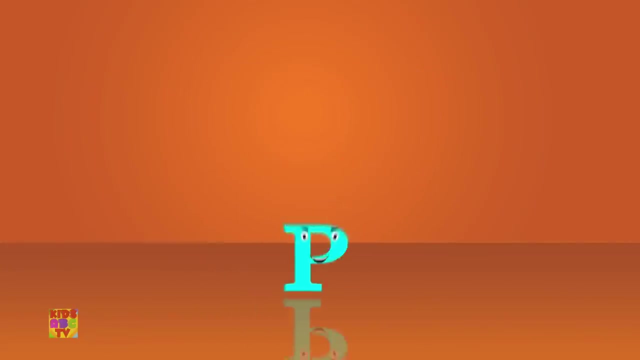 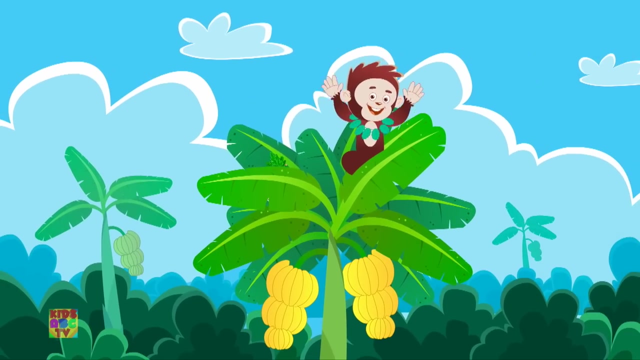 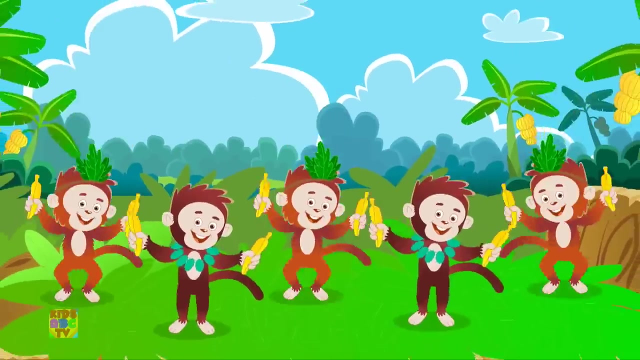 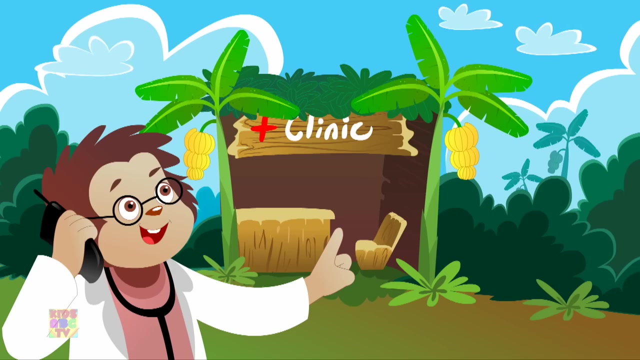 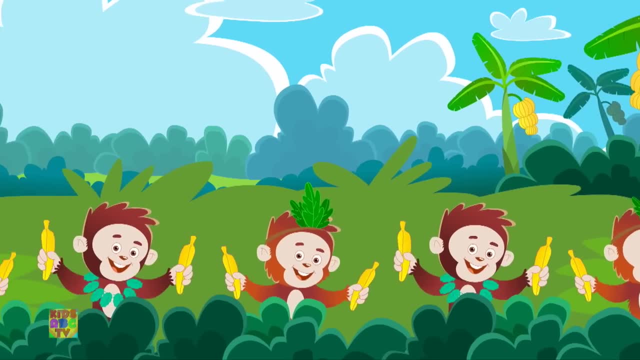 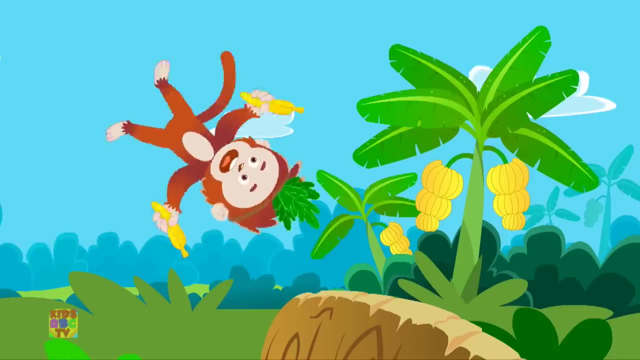 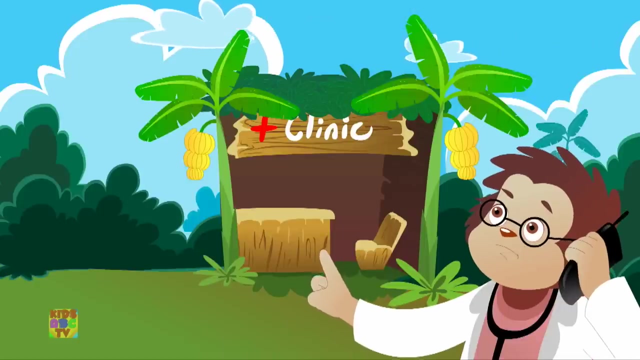 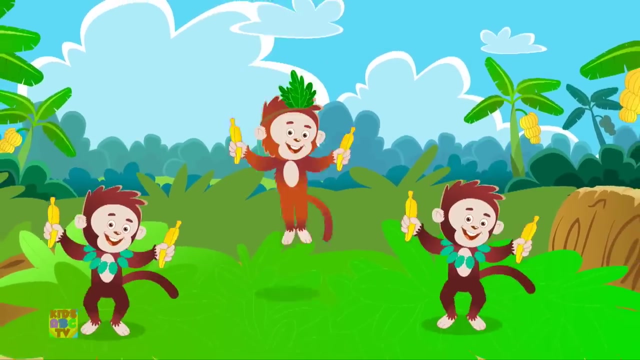 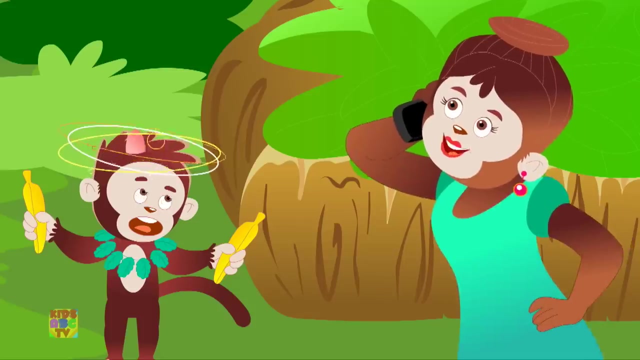 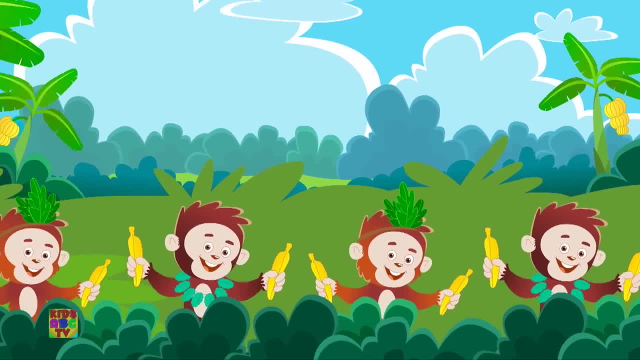 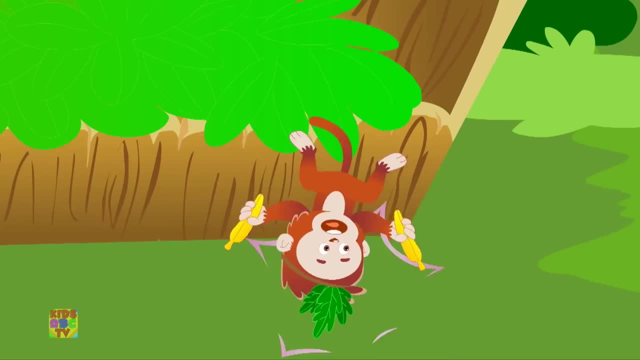 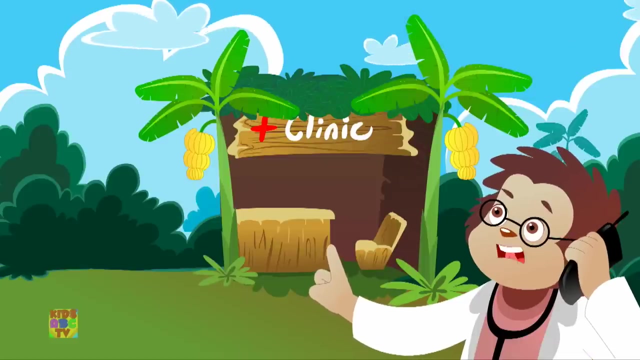 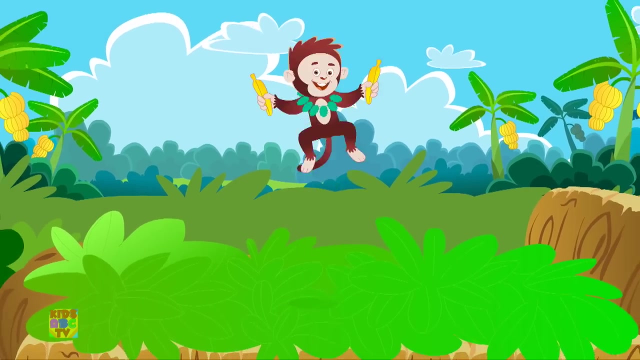 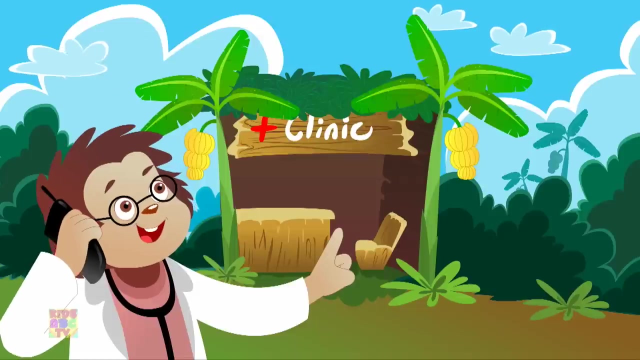 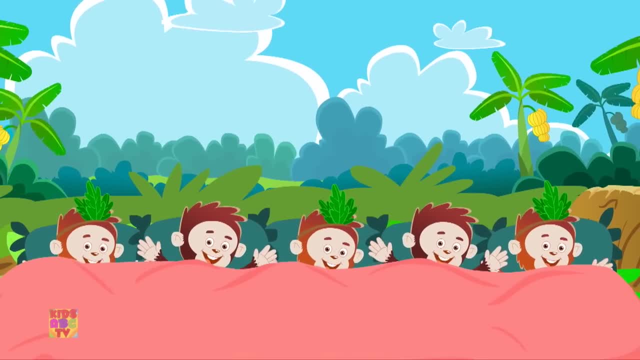 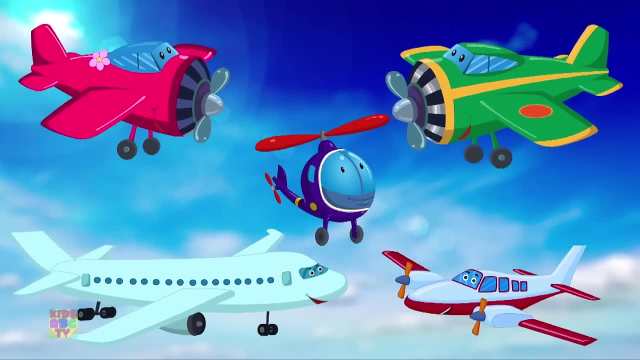 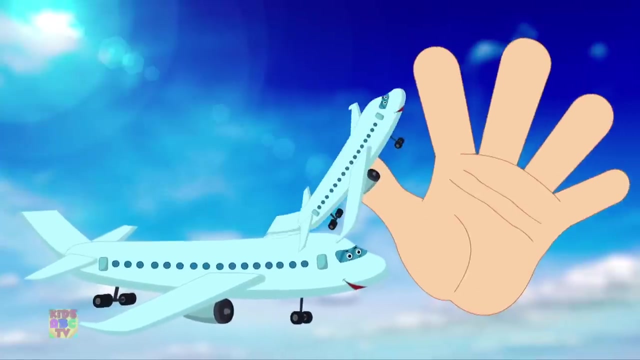 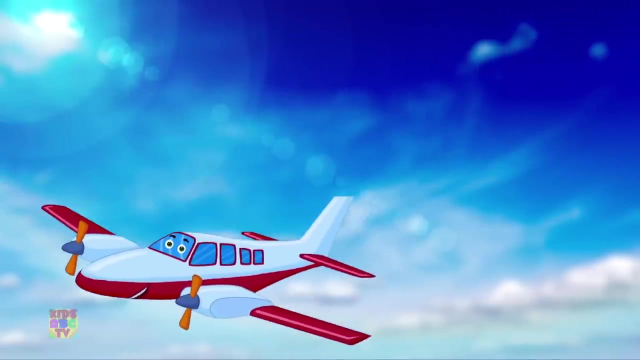 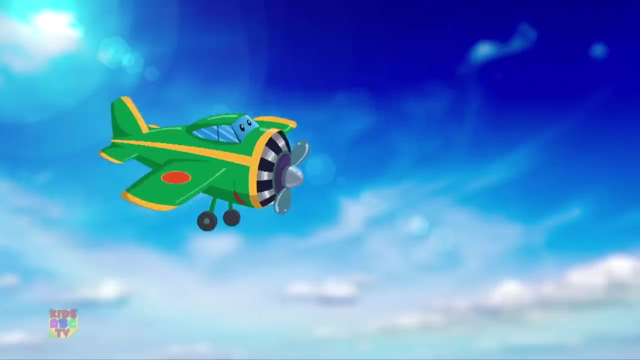 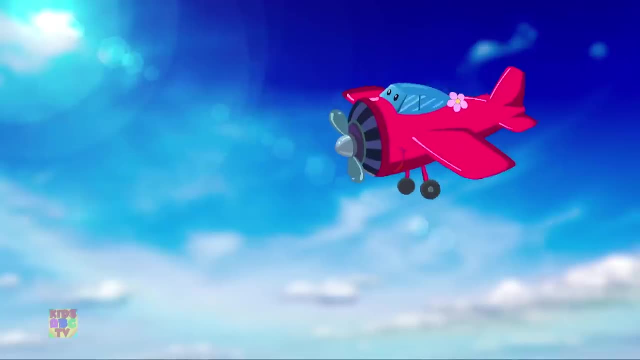 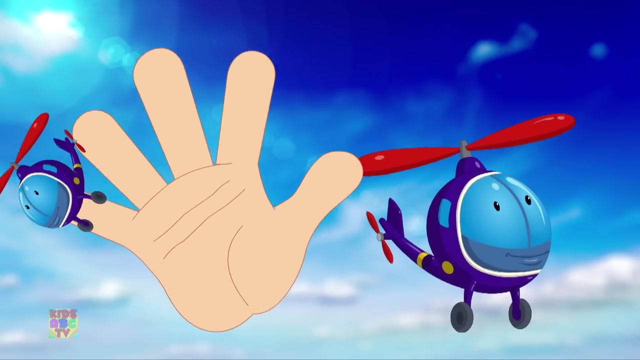 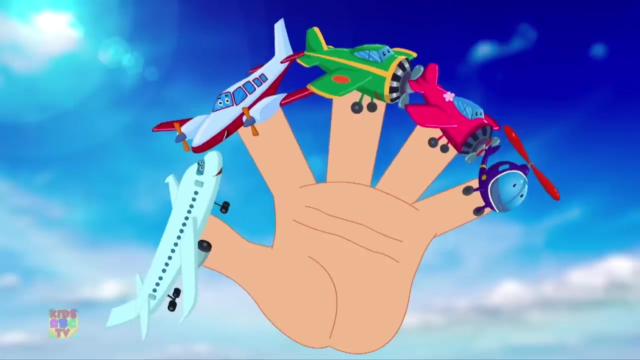 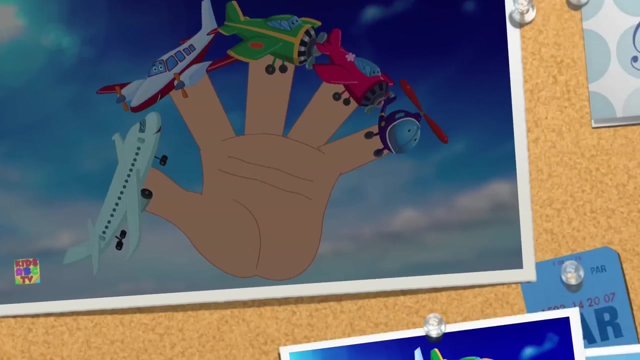 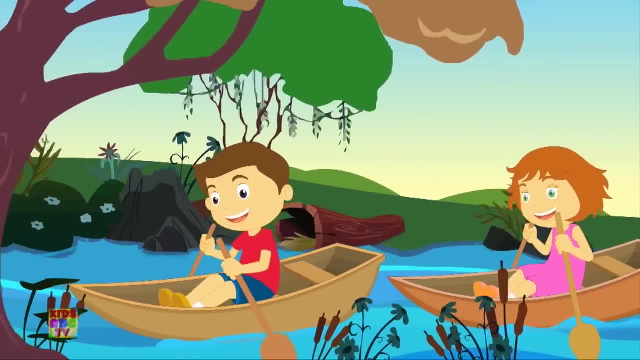 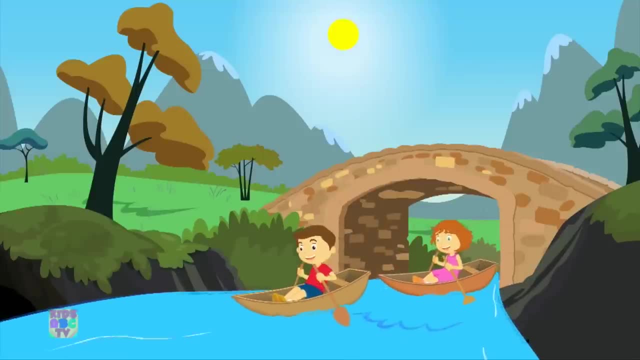 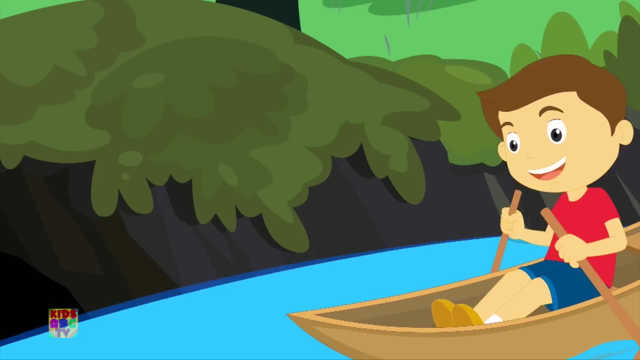 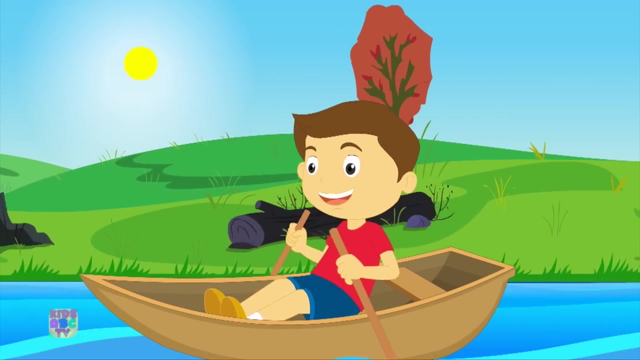 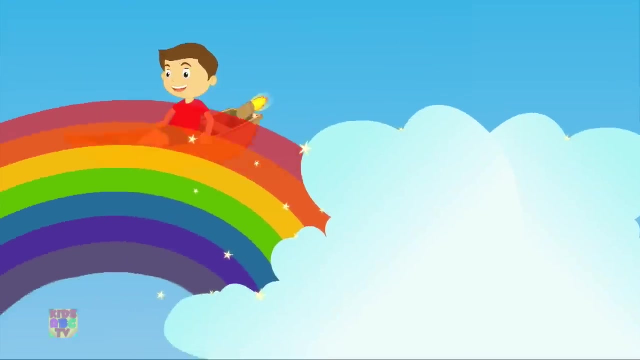 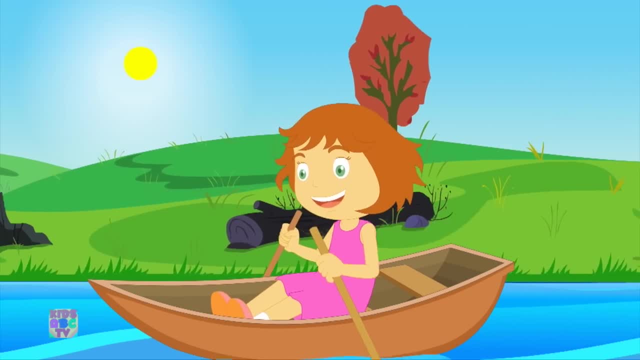 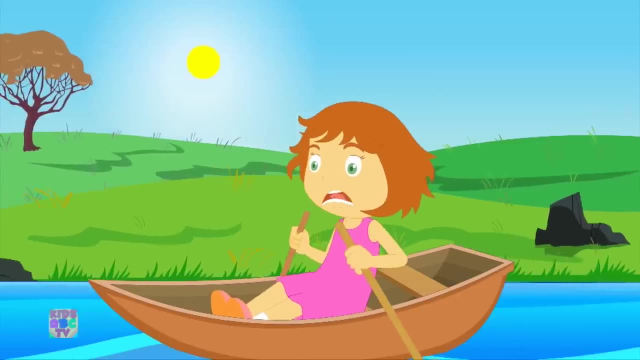 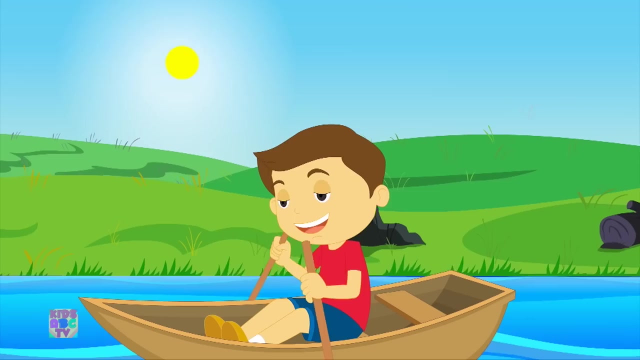 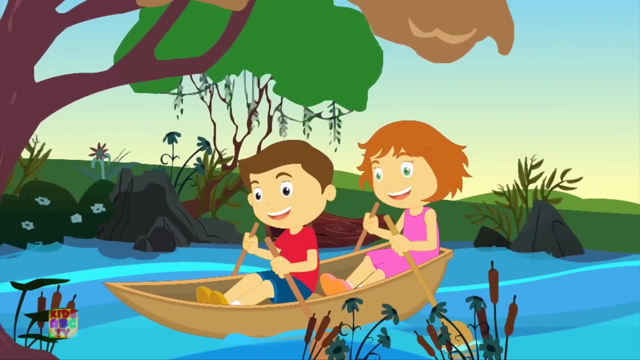 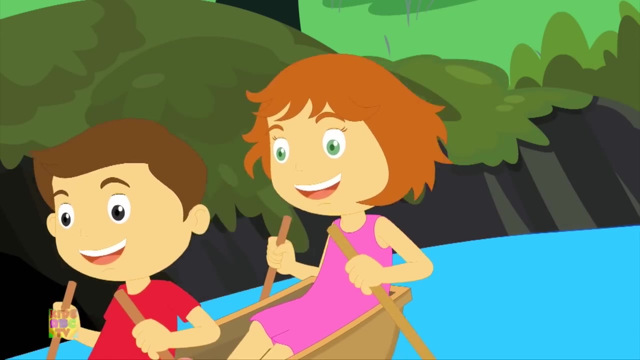 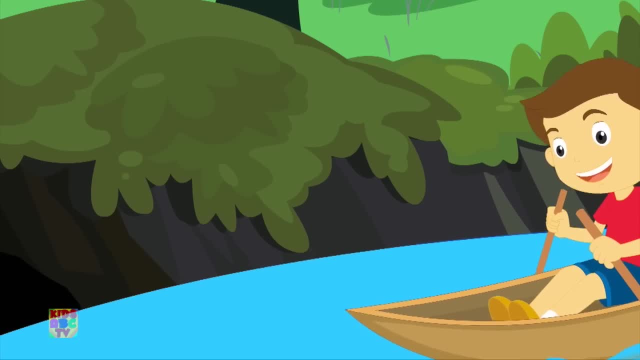 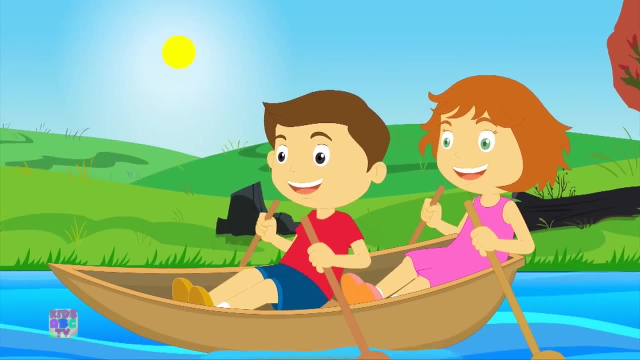 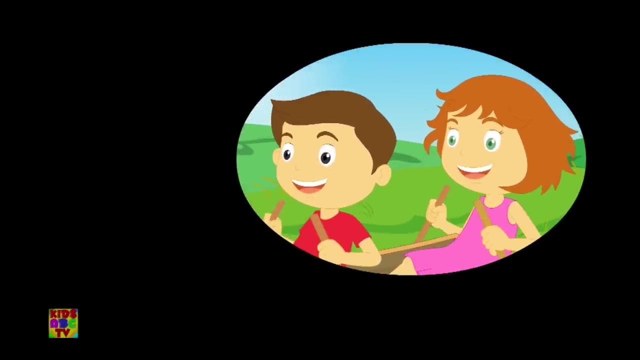 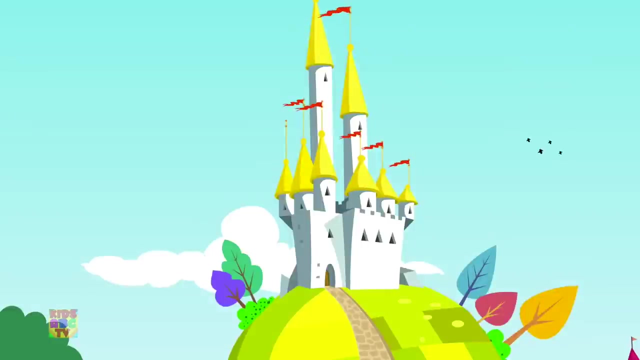 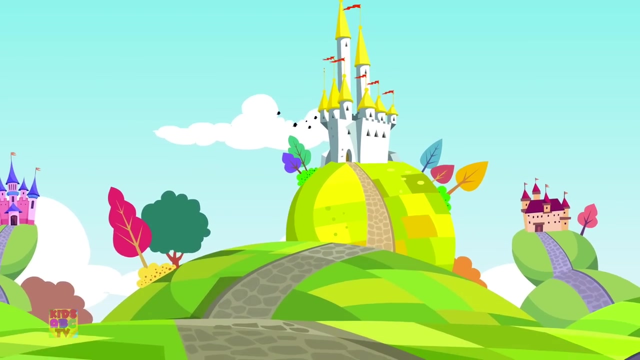 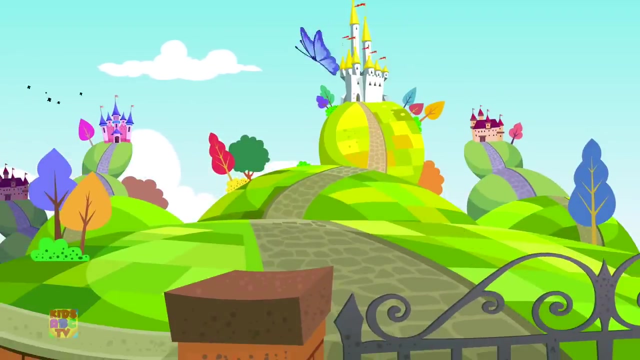 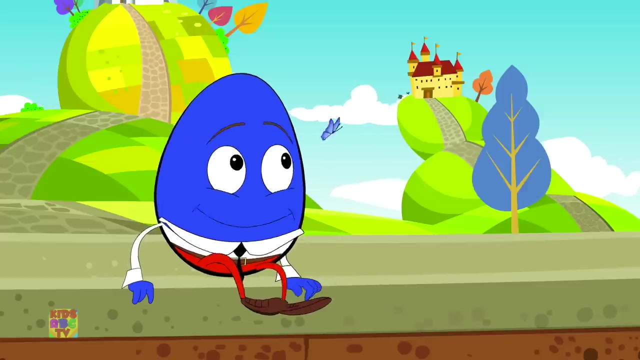 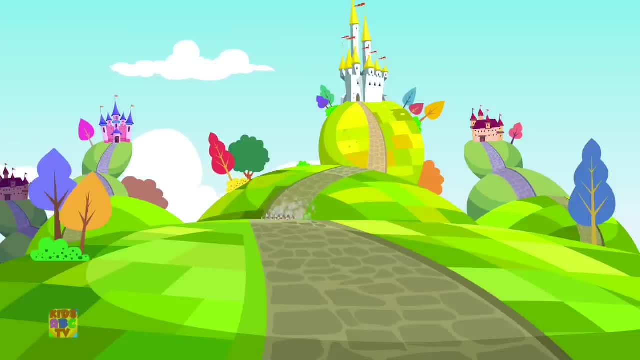 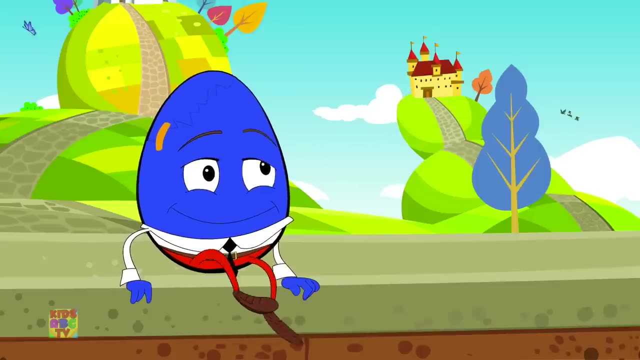 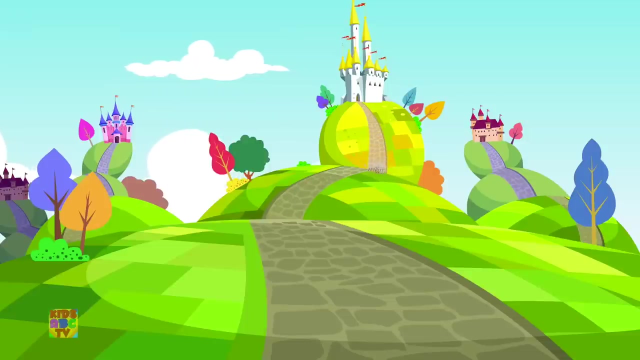 All the king's horses and all the king's men Couldn't put Humpty together again. Humpty Dumpty sat on a wall. Humpty Dumpty had a great fall. All the king's horses and all the king's men Couldn't put Humpty together again. 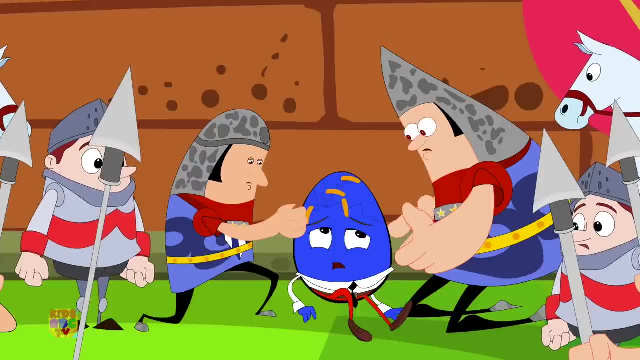 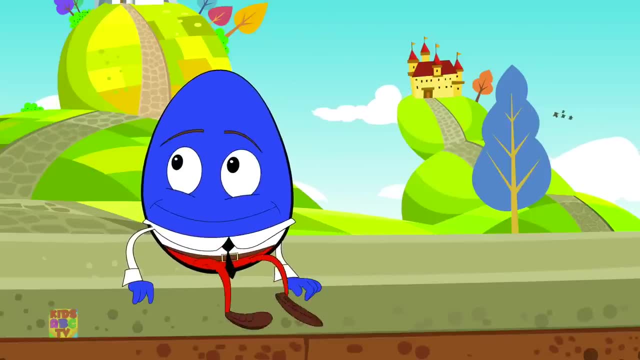 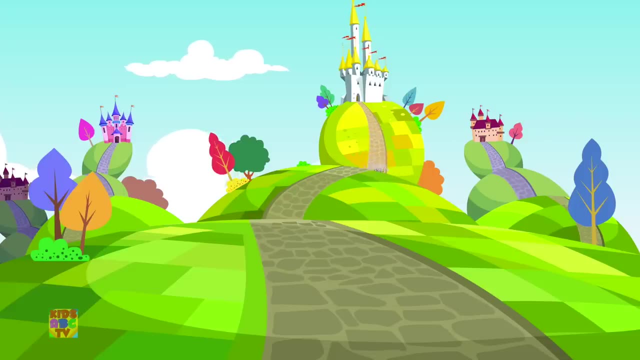 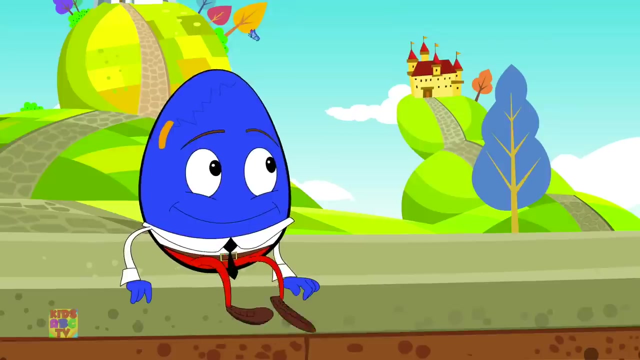 Poor Humpty Dumpty. he's always falling down. Humpty Dumpty sat on a wall. Humpty Dumpty had a great fall. All the king's horses and all the king's men Couldn't put Humpty together again. Humpty Dumpty sat on a wall. 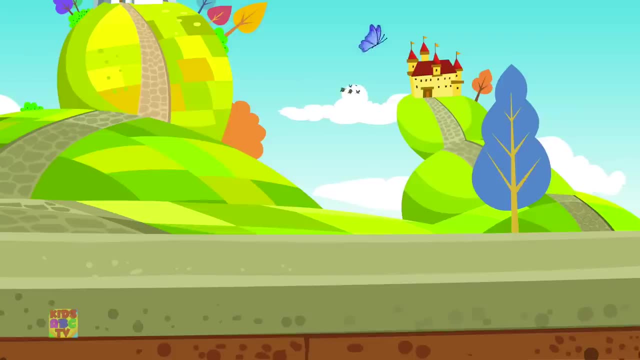 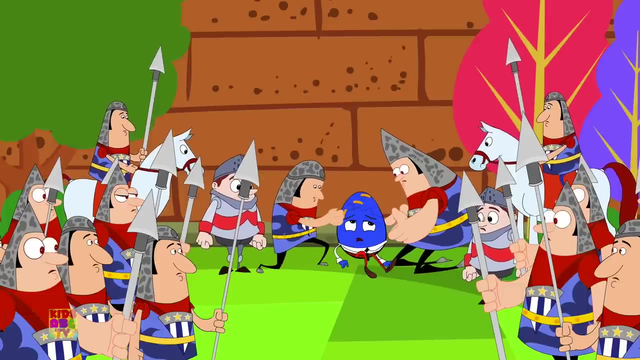 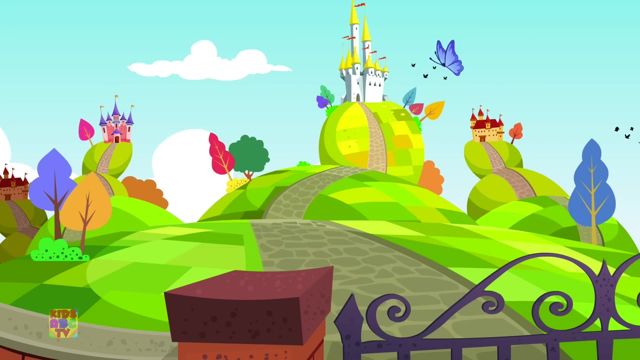 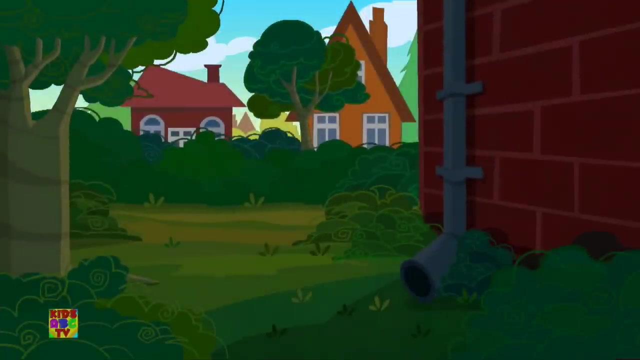 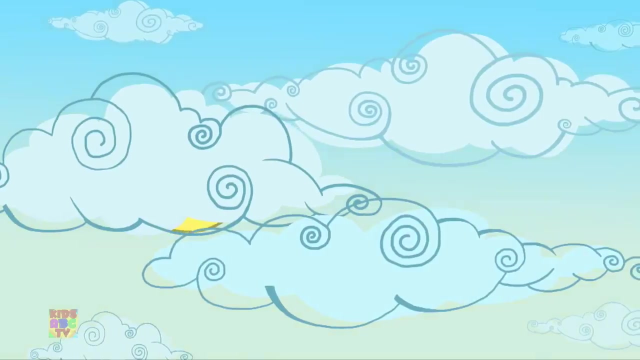 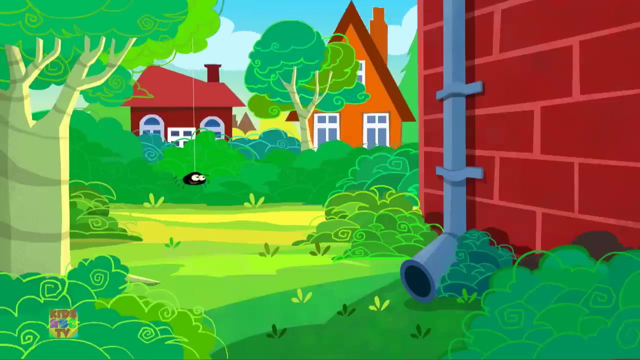 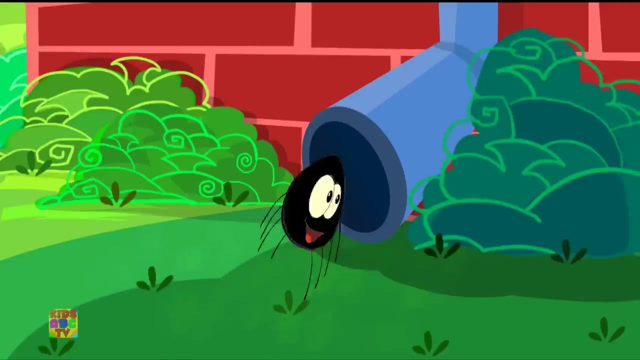 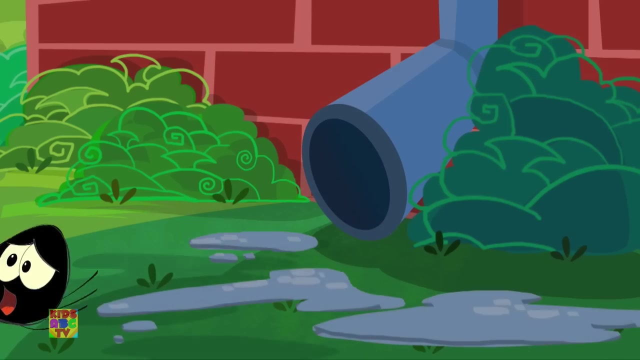 Humpty Dumpty had a great fall. All the king's horses and all the king's men Couldn't put Humpty together again. Oh, Humpty Dumpty, Incy Wincy Spider crawled up the water, spout. Down came the rain and washed the spider out. 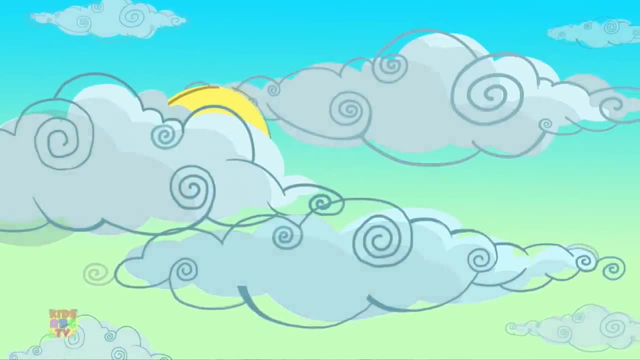 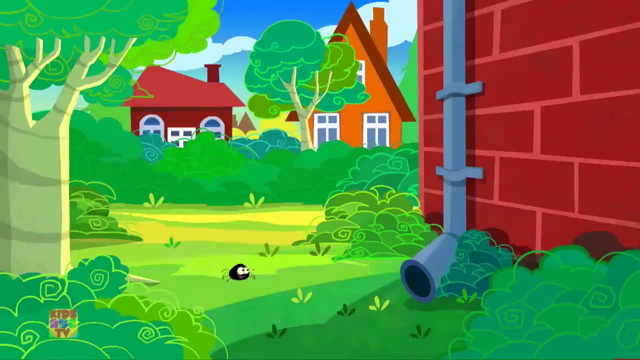 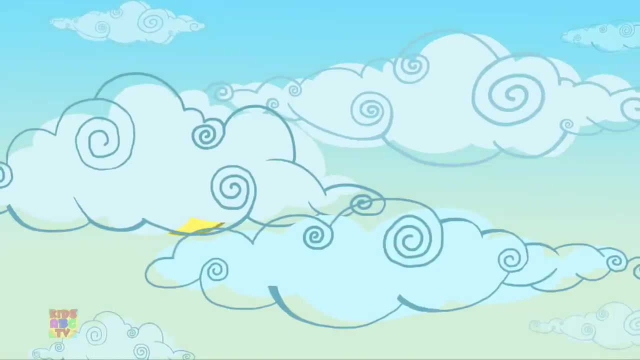 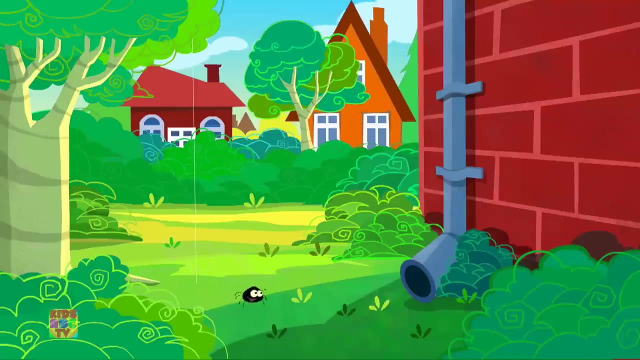 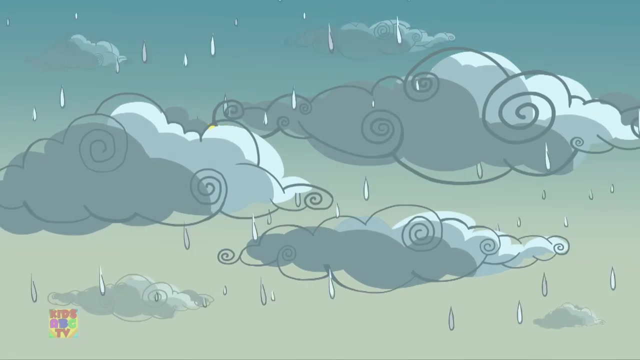 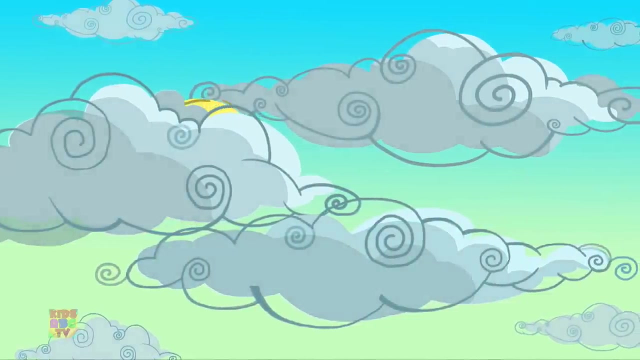 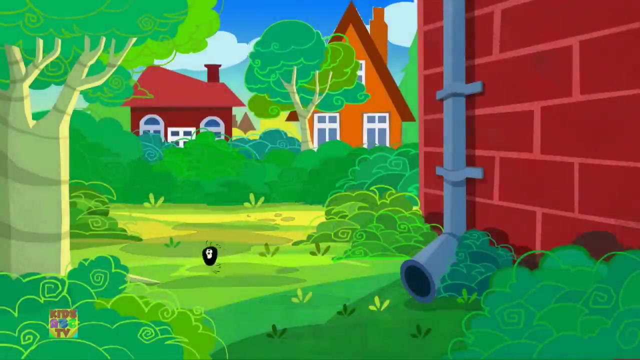 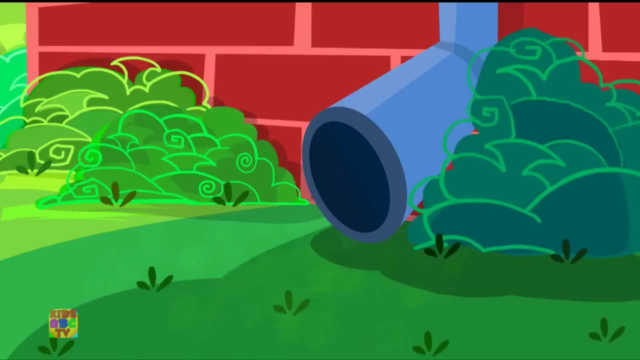 Out came the sun and dried up all the rain. Incy Wincy Spider crawled up the spout. Incy Wincy Spider crawled up the water spout, Down came the rain and washed the spider out. Out came the sun and dried up all the rain. Incy Wincy Spider crawled up the spout again. 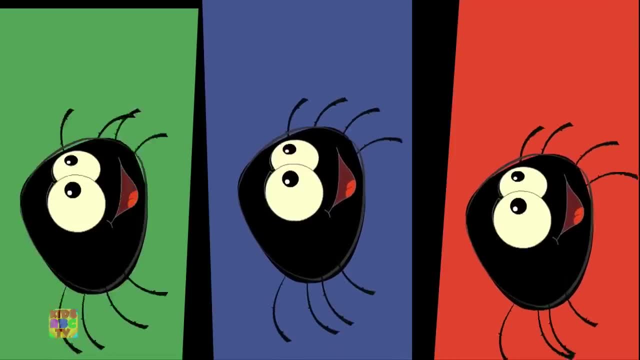 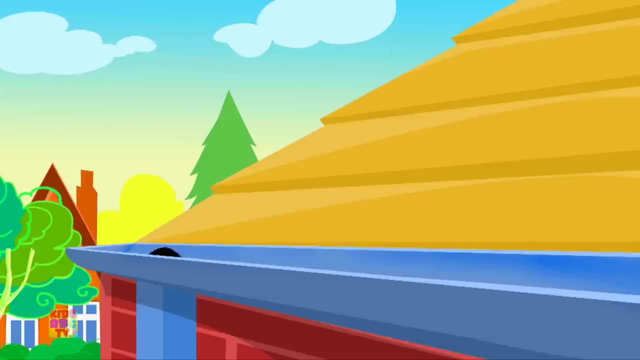 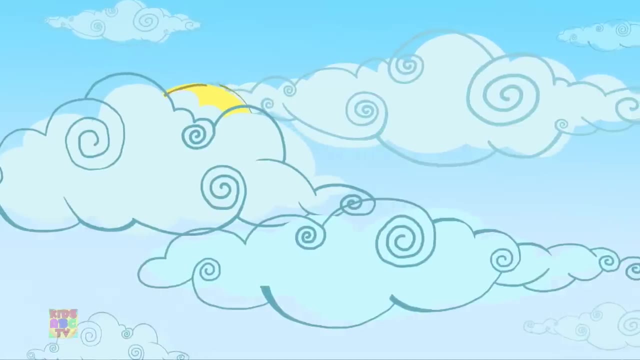 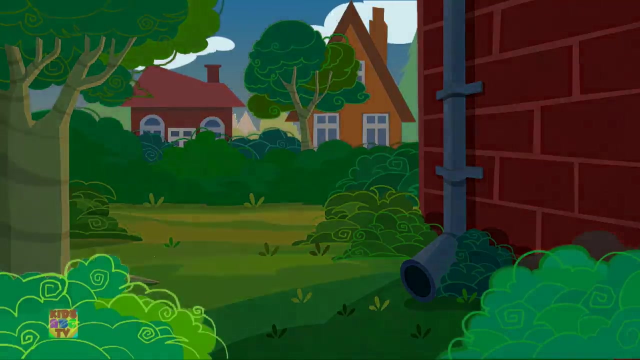 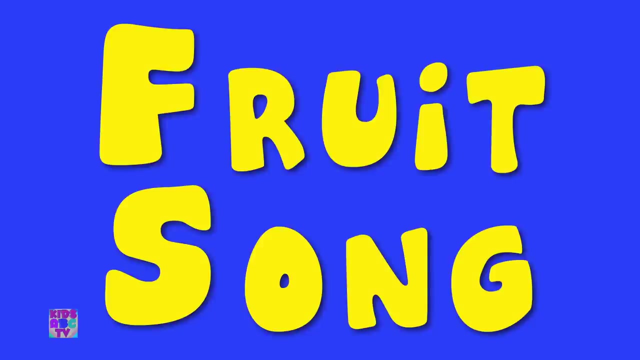 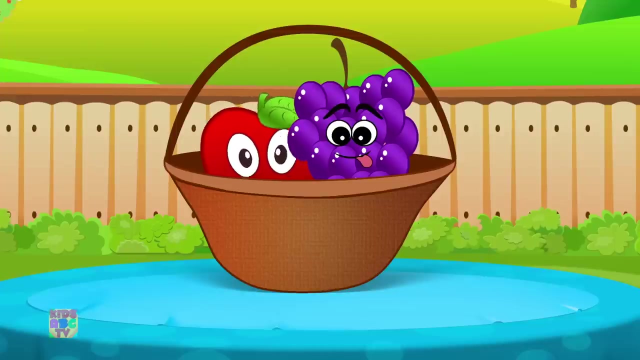 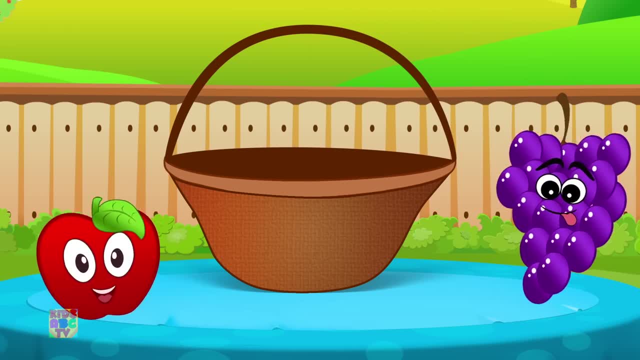 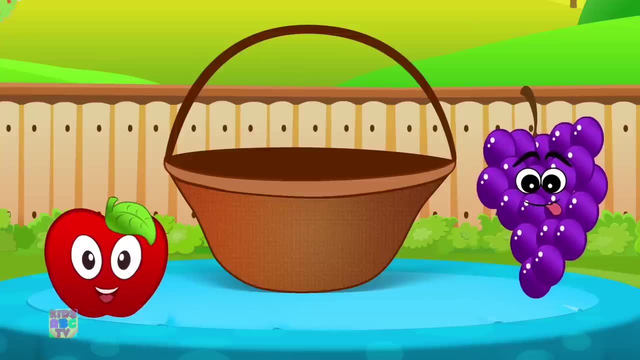 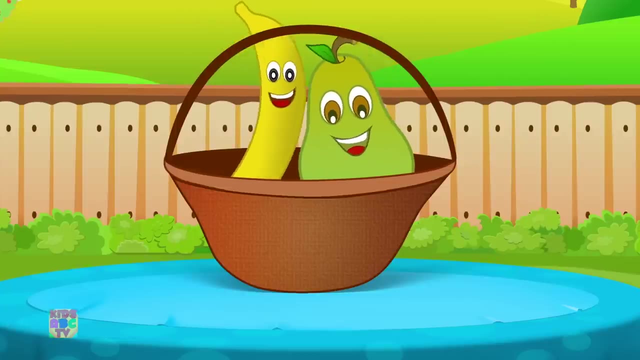 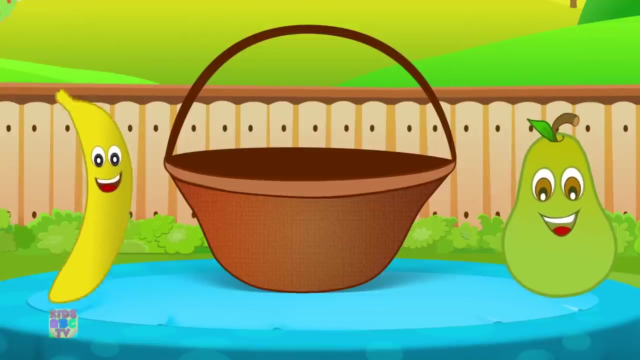 Sometimes I want some grapes. Some days I'm feeling hungry And then I want to eat them. Oh, Look, There's a banana. Sometimes I want a banana, Sometimes I want a pear. Some days I'm feeling hungry And then I want to eat them, Oh. 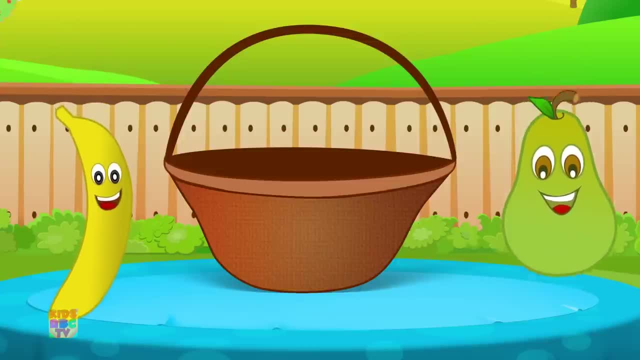 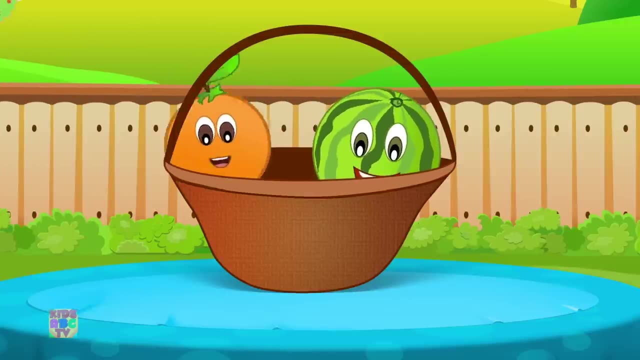 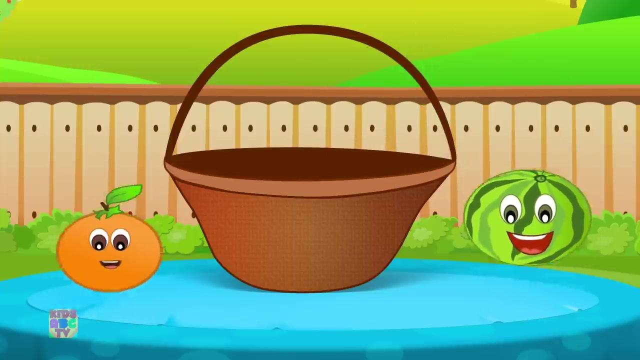 Oh, I really like fruits. Oh, I really like fruits. Oh, I really like fruits. At times I want an orange. At times I want an orange, Sometimes a watermelon. Some days I'm feeling hungry. Some days I'm feeling hungry, And then I want to eat them all. 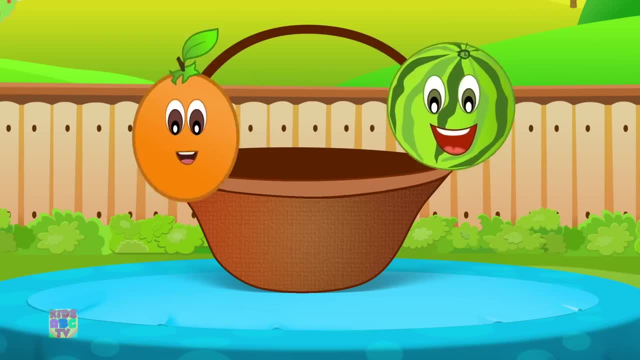 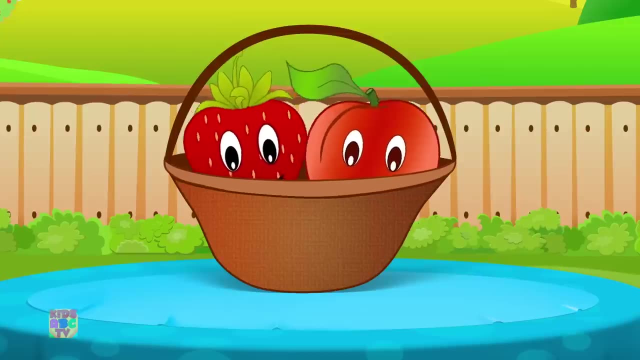 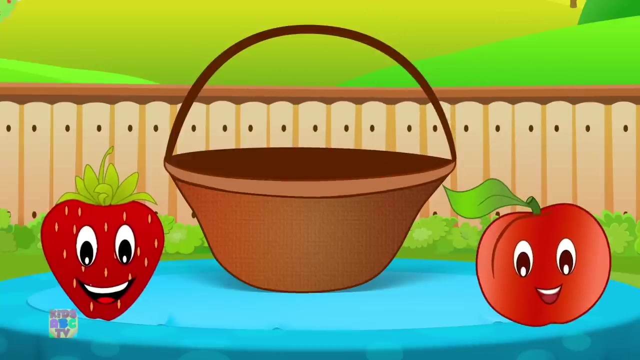 And then I want to eat them all. And then I want to eat them all. Look, there Are those strawberries. Are those strawberries? Sometimes I want strawberries. Sometimes I want a peach. Sometimes I want a peach. Some days I'm feeling hungry. Some days I'm feeling hungry. 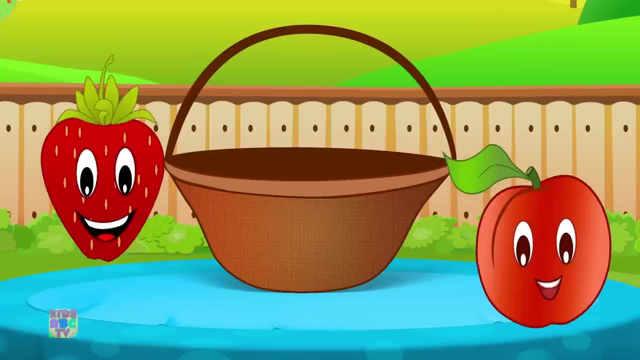 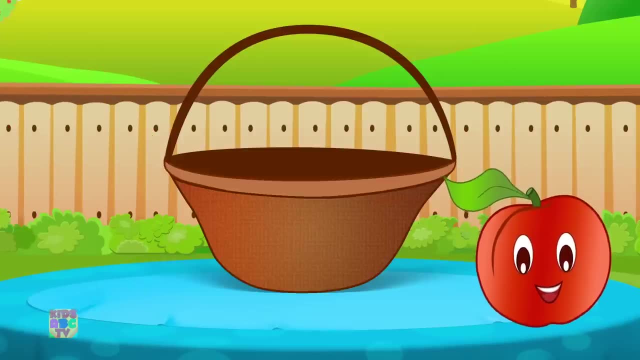 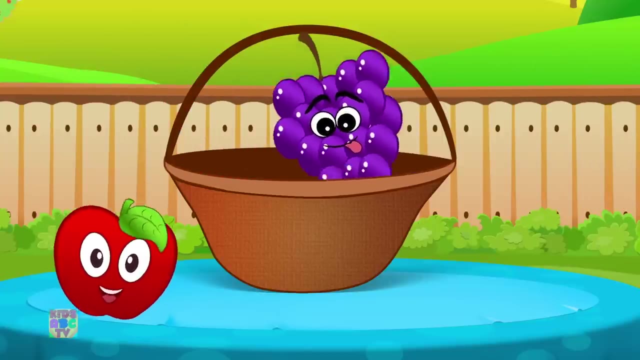 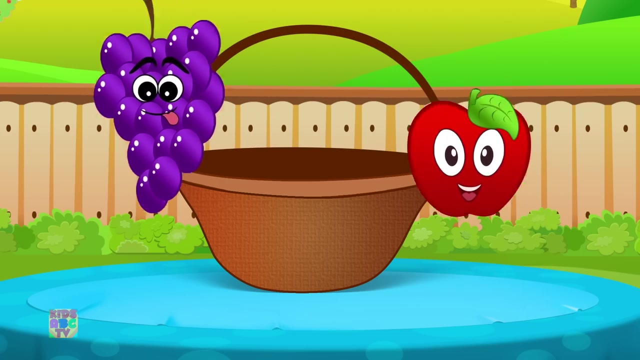 And then I want to eat them all. And then I want to eat them all. I want some more fruits. At times I want an apple. At times I want an apple. Sometimes I want some grapes. Some days I'm feeling hungry, And then I want to eat them all. 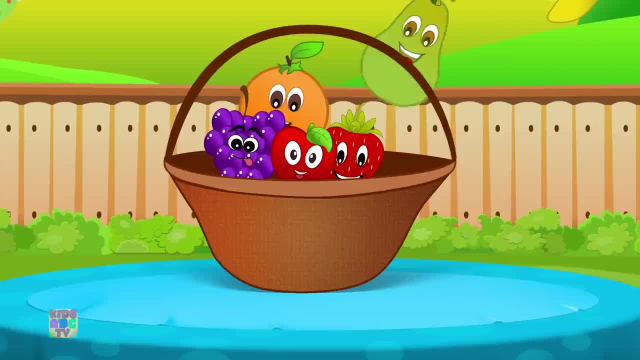 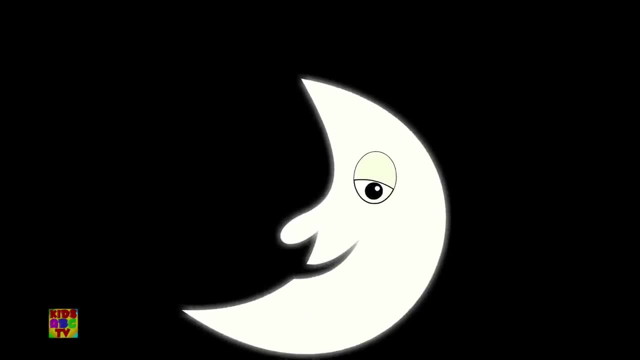 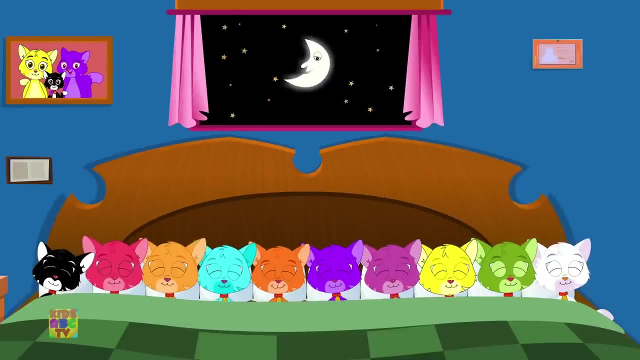 Fruits, Fruits, Fruits And more fruits. There were ten in the bed and the little one said: Roll over, Roll over. So they all rolled over and one fell out. Nine, Nine. There were nine in the bed and the little one said: 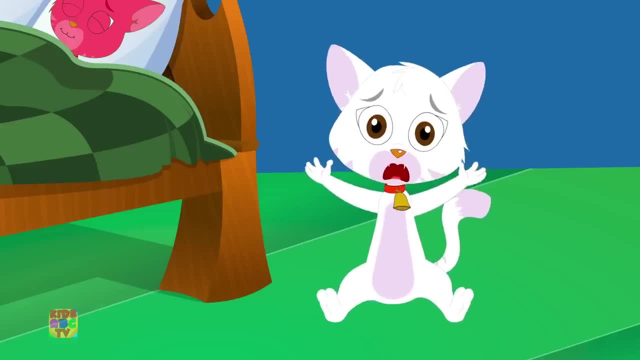 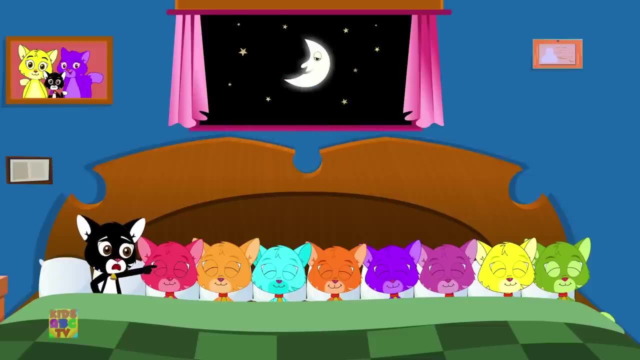 Roll over, Roll over. So they all rolled over and one fell out. Eight, Eight. There were eight in the bed and the little one said: Roll over, Roll over. So they all rolled over and one fell out. Eight, Eight, There were eight in the bed and the little one said: 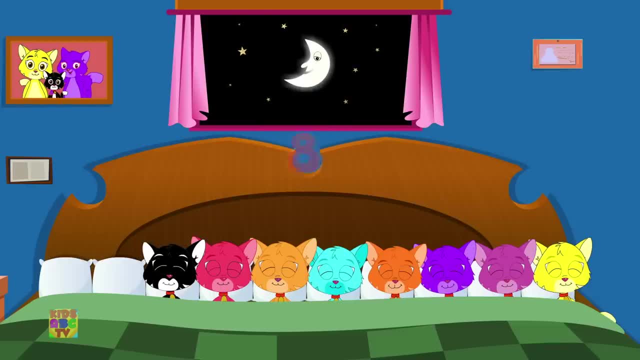 Roll over, Roll over. So they all rolled over and one fell out Seven, Seven. There were seven in the bed and the little one said: Roll over, Roll over. So they all rolled over and one fell out Seven, Seven. There were seven in the bed and the little one said: 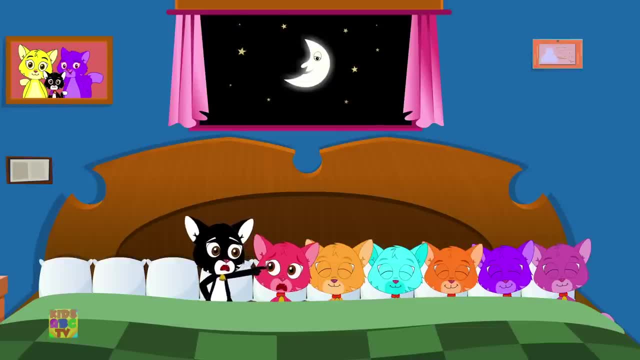 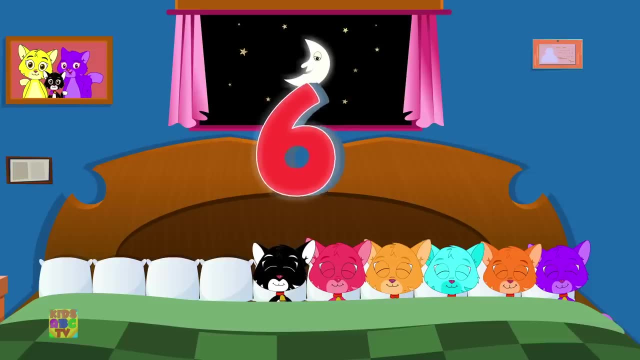 Roll over, Roll over. So they all rolled over and one fell out Six, Six. There were six in the bed and the little one said: Roll over, Roll over. So they all rolled over and one fell out Six, Six. There were six in the bed and the little one said: 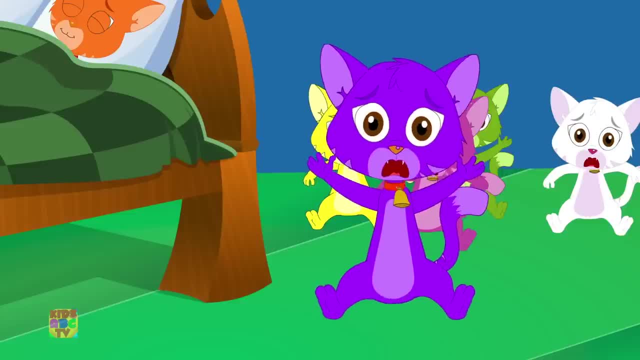 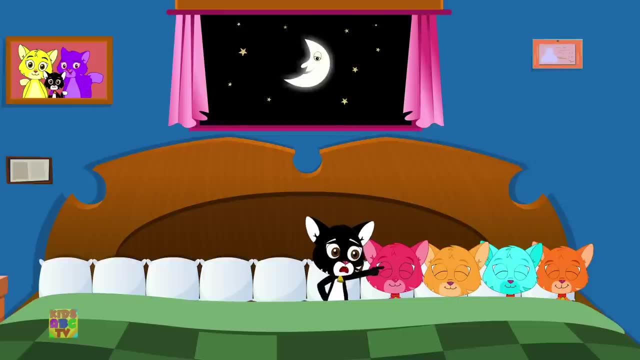 Roll over, Roll over. So they all rolled over and one fell out Five, Five. There were five in the bed and the little one said: Roll over, Roll over. So they all rolled over and one fell out Four, Four. There were four in the bed and the little one said: 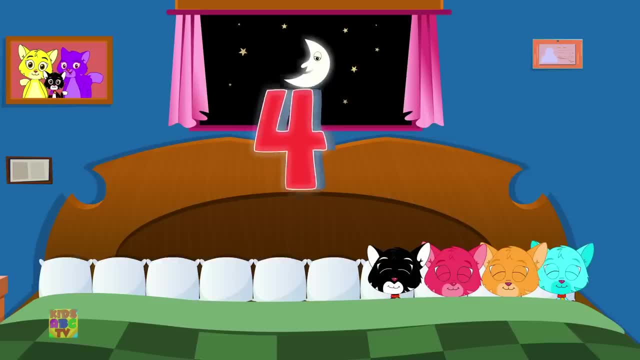 Roll over, Roll over. So they all rolled over and one fell out Three, Three. There were three in the bed and the little one said: Roll over, Roll over. So they all rolled over and one fell out Three, Three. There were three in the bed and the little one said: 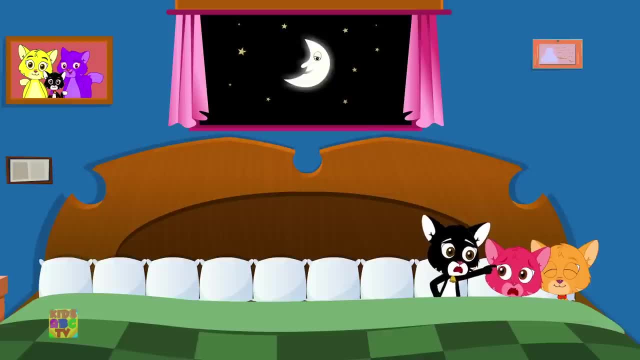 Roll over, Roll over. So they all rolled over and one fell out. Two, Two. There were two in the bed and the little one said: Roll over, Roll over. So they all rolled over and one fell out. One, One. There was one in the bed and the little one said: 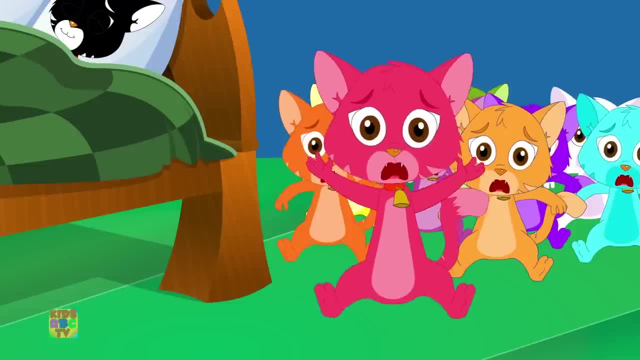 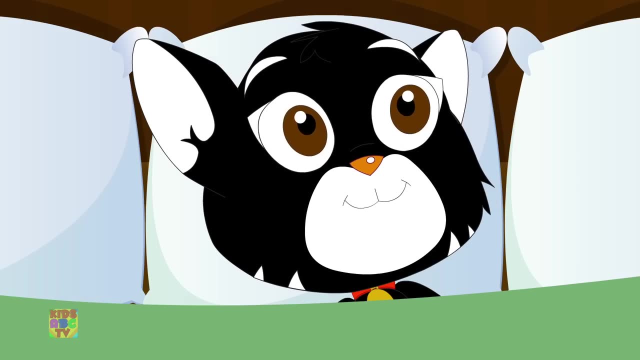 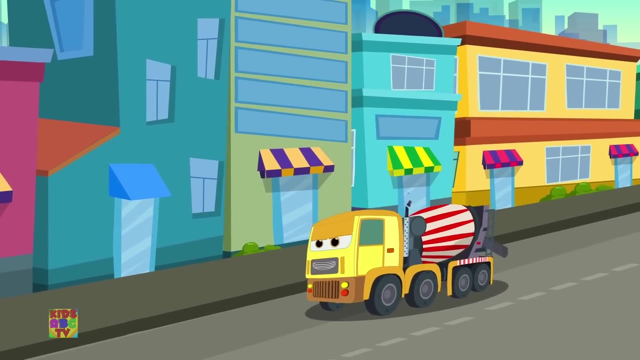 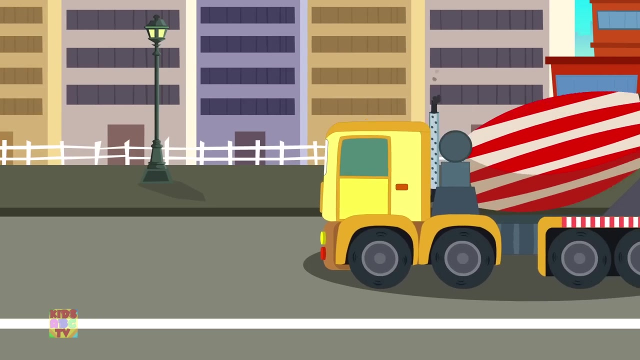 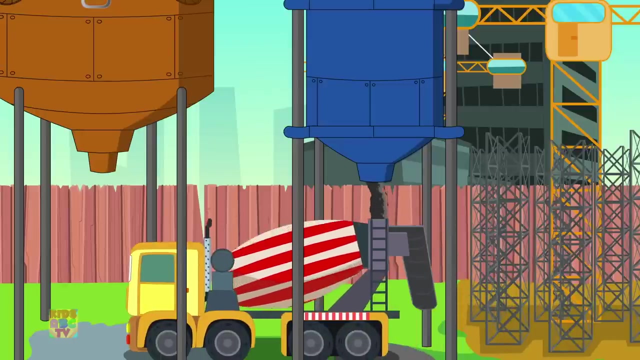 Good night. Look, It's the cement mixer truck. Why does it go round and round? I go round and round To keep the concrete all unstuck. I go round and round The day long. I'm the cement mixer truck. I go round and round. 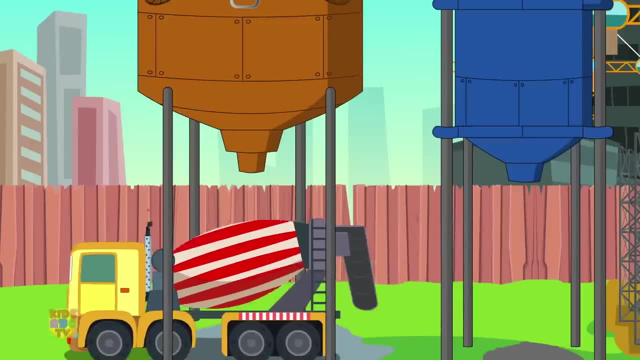 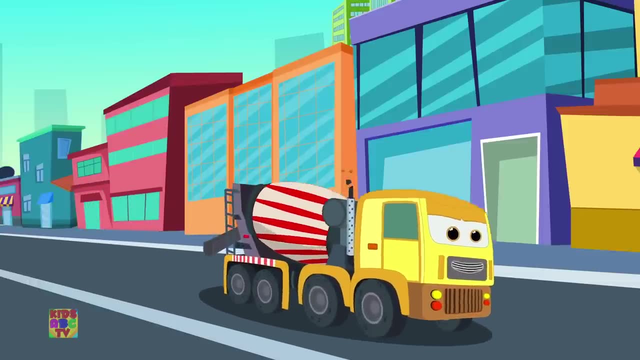 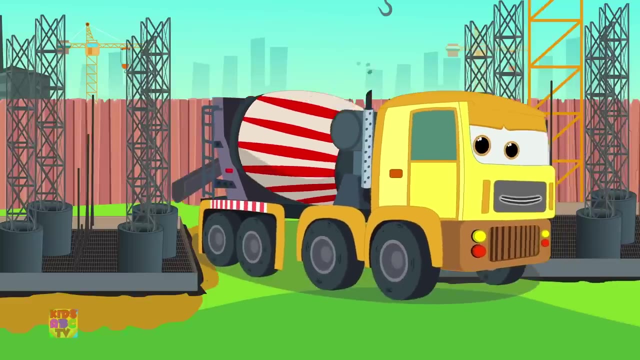 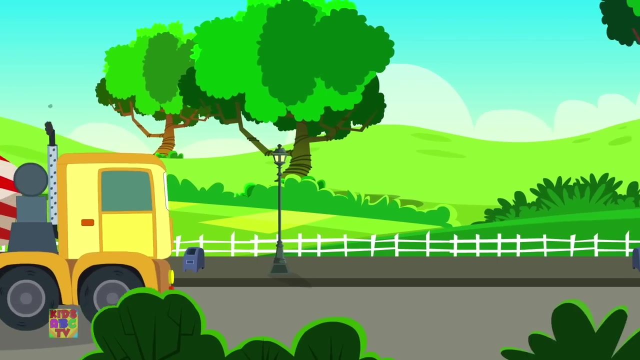 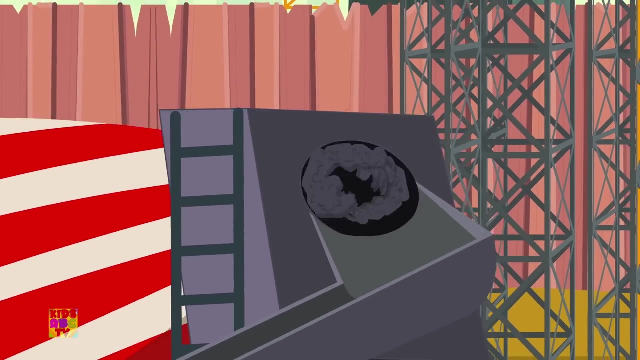 To keep the concrete all unstuck. I go round and round The day long. I'm the cement mixer truck. I take the concrete to the construction site And it must not set Until I reach there. I go round and round To keep the concrete all unstuck. I go round and round. 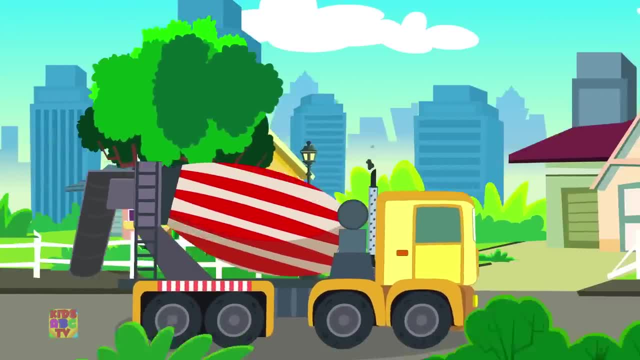 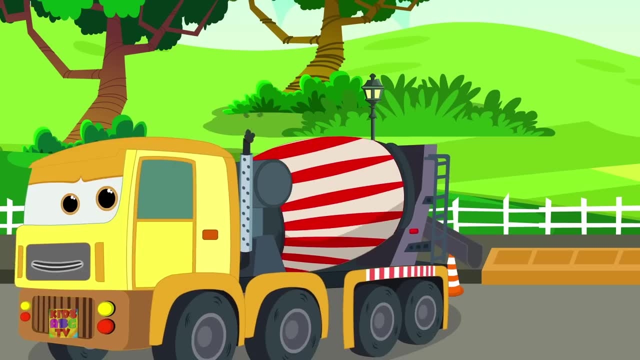 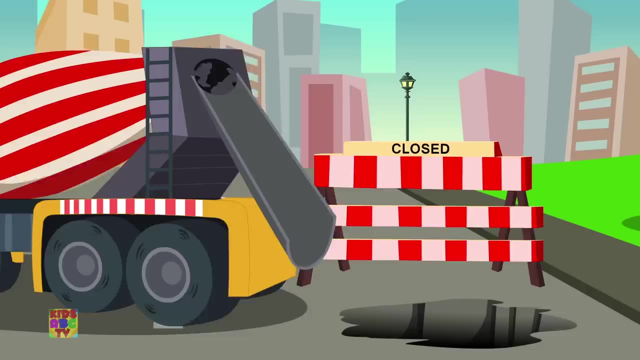 The day long. I'm the cement mixer truck. I go round and round To keep the concrete all unstuck. I go round and round The day long. I'm the cement mixer truck. My drum keeps turning all the way. This way, the concrete doesn't set Till I pour it out. 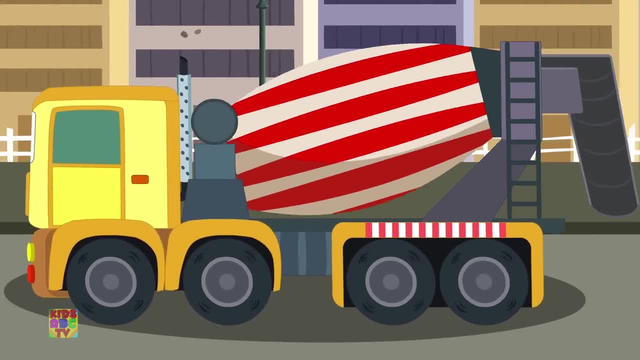 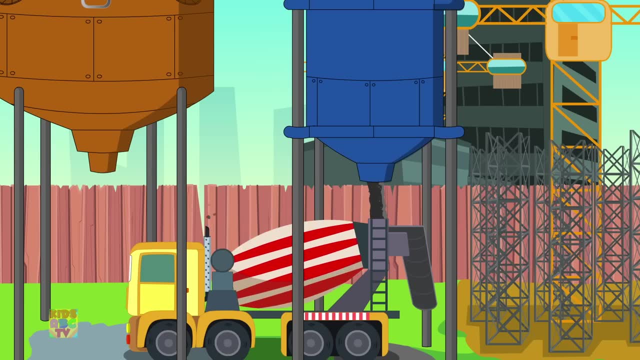 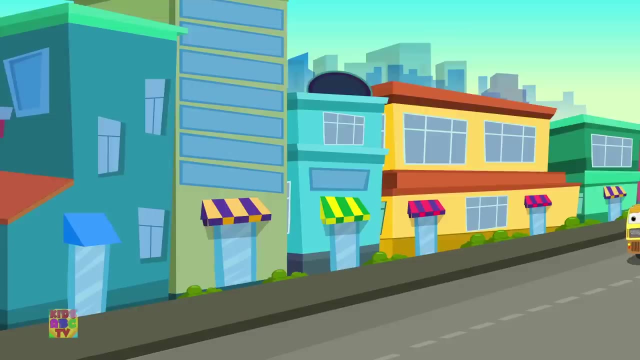 I go round and round To keep the concrete all unstuck. I go round and round The day long. I'm the cement mixer truck. I go round and round To keep the concrete all unstuck. I go round and round The day long. I'm the cement mixer truck. 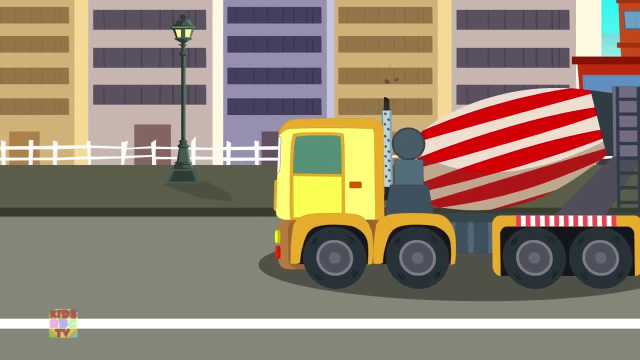 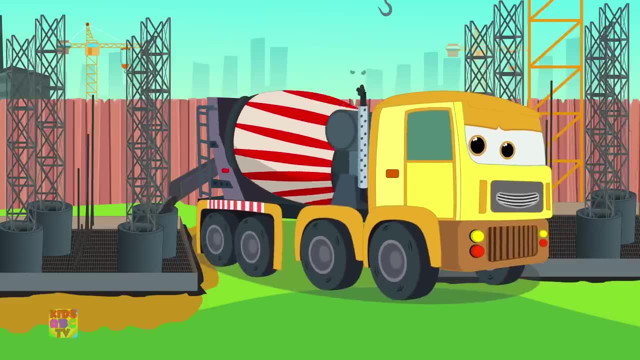 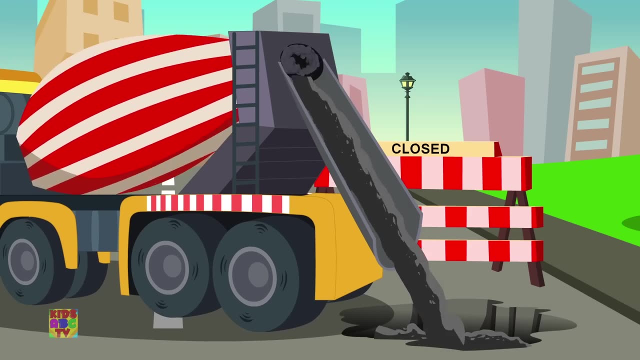 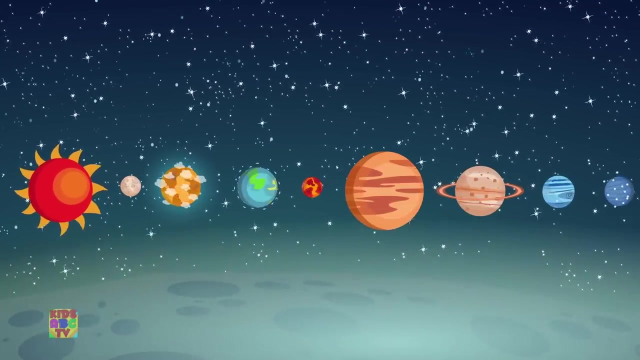 I go round and round To keep the concrete all unstuck. I go round and round The day long. I go round and round The day long. I go round and round To keep the concrete all unstuck. I go round and round. Spread your hands, Go round and round. 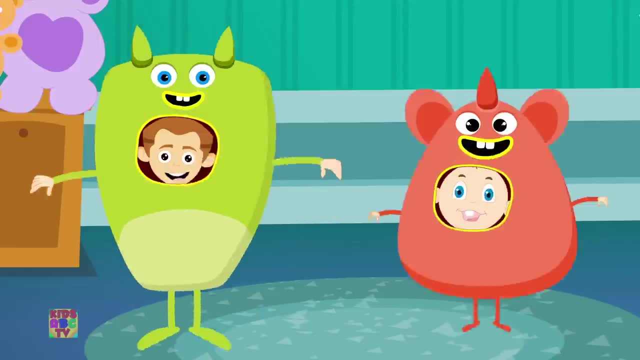 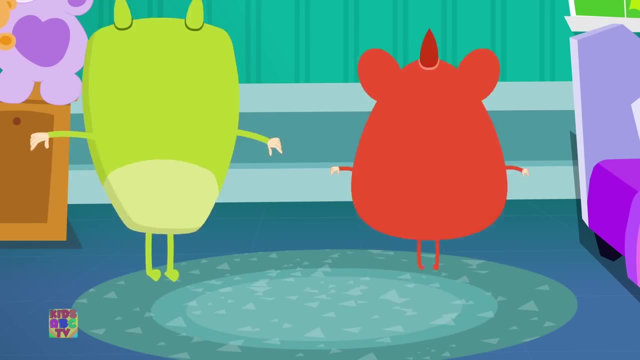 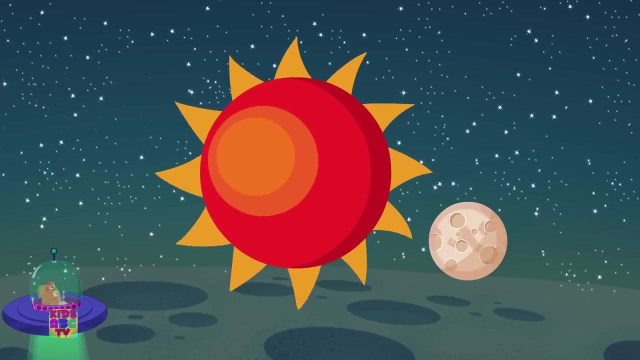 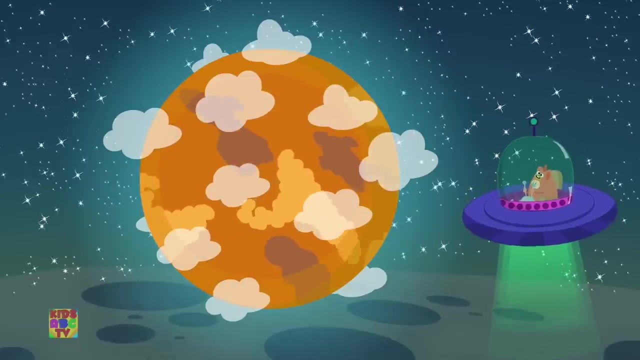 Now tap your feet And sing the planet song. Spread your hands, Go round and round. Now tap your feet and sing this planet song. Can you see Mercury? It's so close to the Sun. There's Venus, so precious Bright and all covered in clouds. Round and round, round and round. 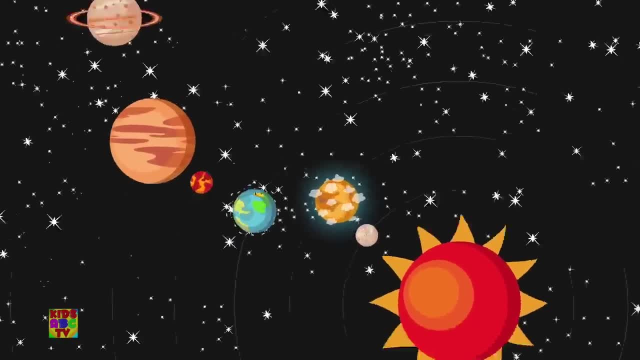 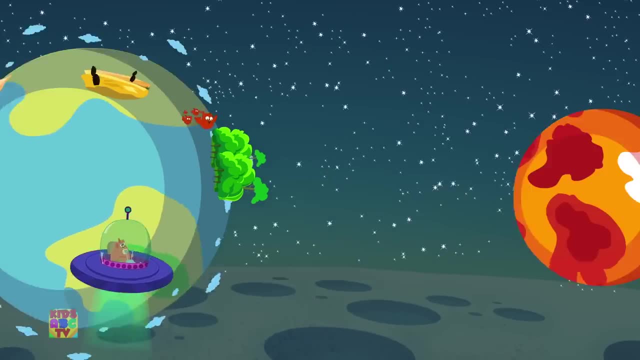 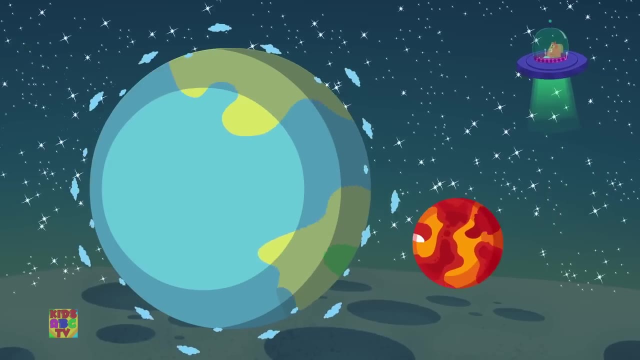 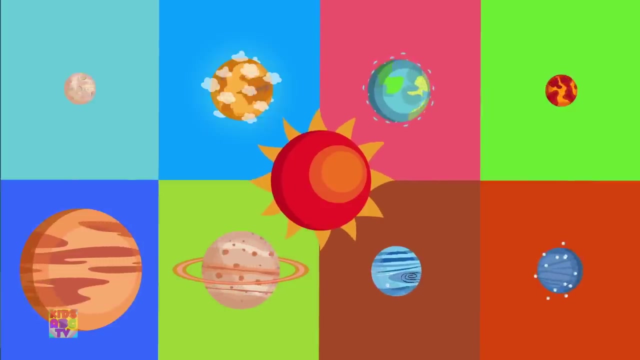 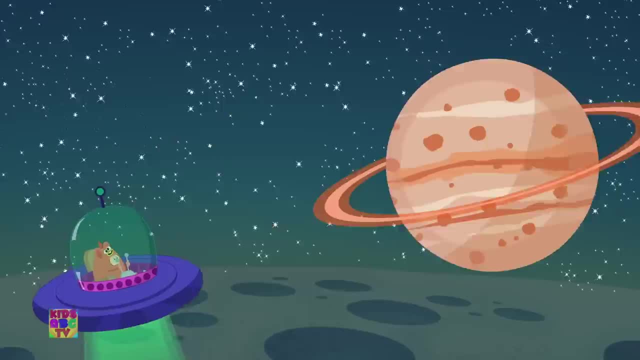 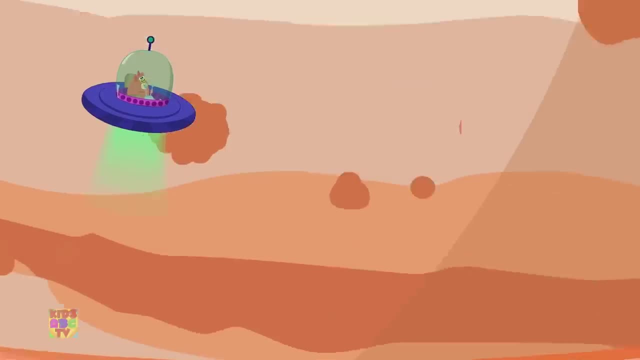 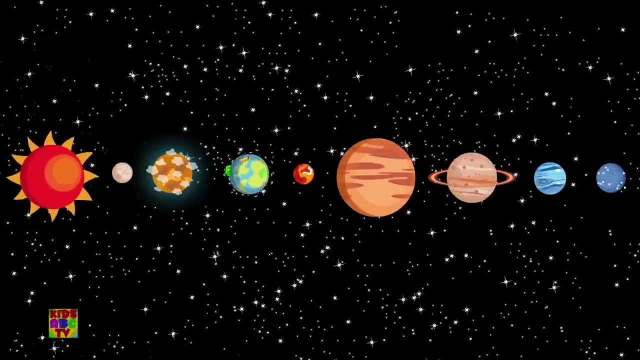 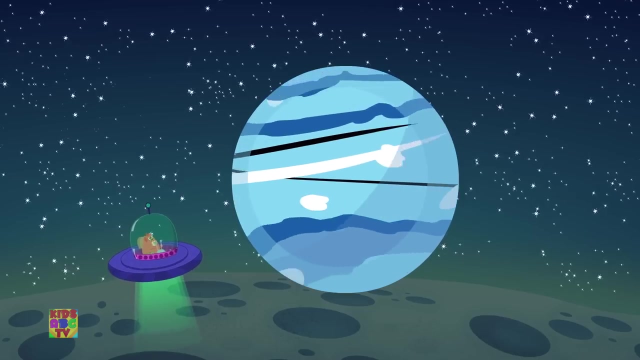 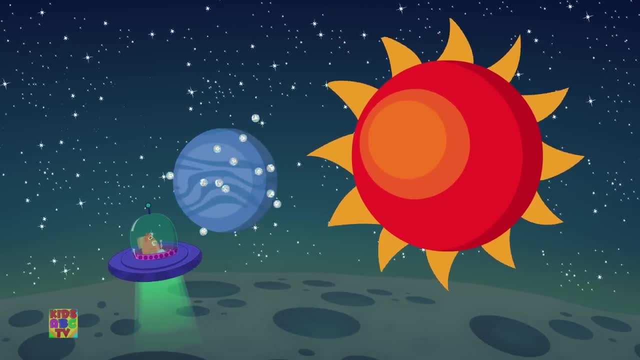 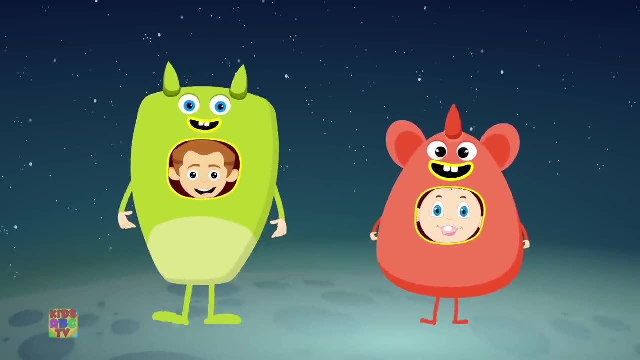 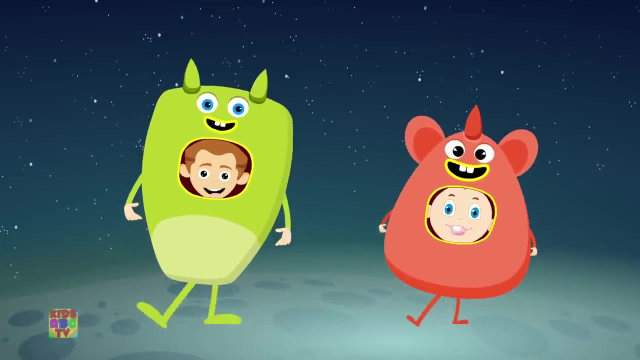 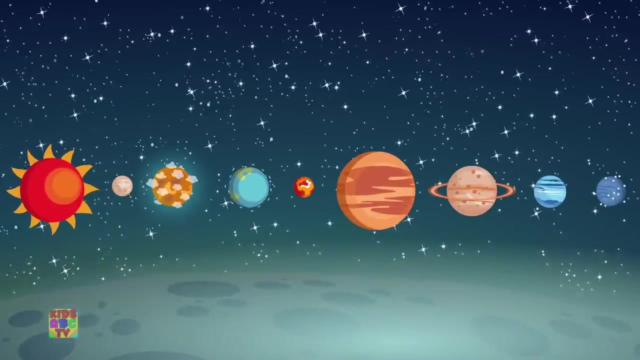 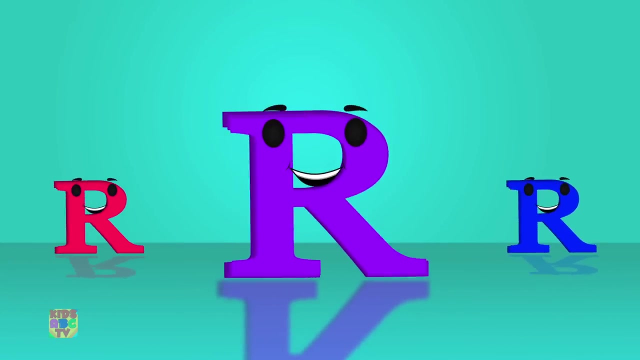 A planet so far from the Sun. It's so close to the Sun. Spread your hands, go round and round Now tap your feet and sing the planet song. Spread your hands, go round and round Now tap your feet and sing the planet song. Here comes the letter R. 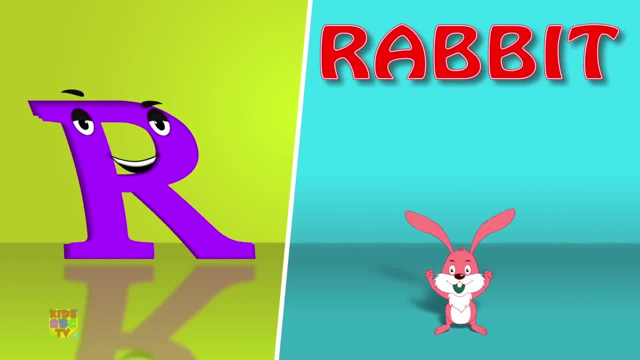 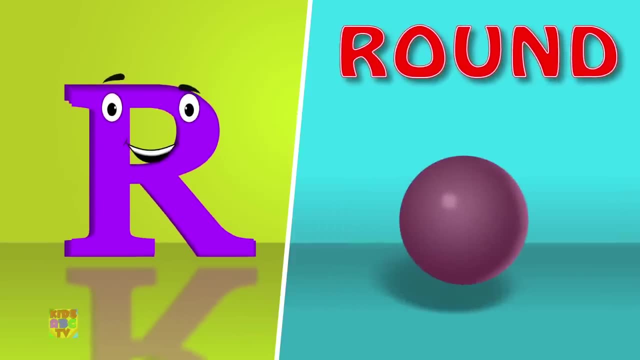 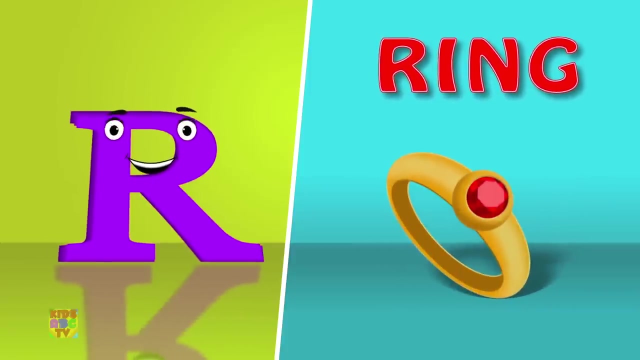 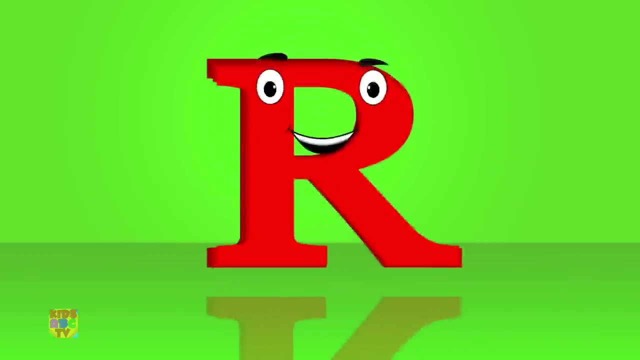 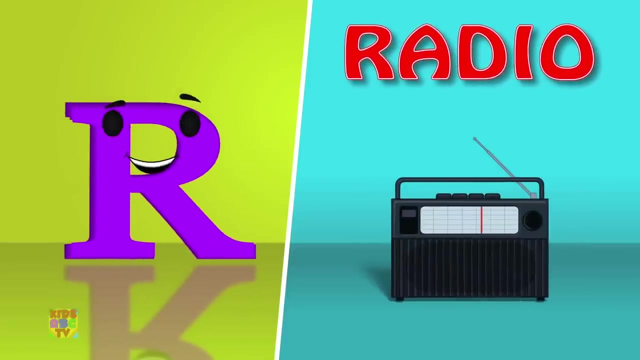 R is for Rabbit R R. Rabbit R is for Rain R R. Rain R is for Round R R. Round R is for Ring R R. Ring R is for Radio R R. Radio R is for Road R R, Road. 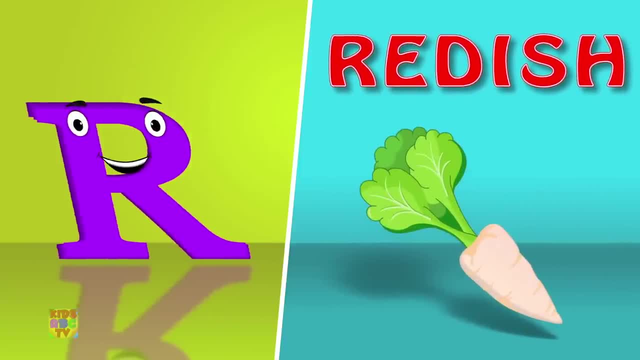 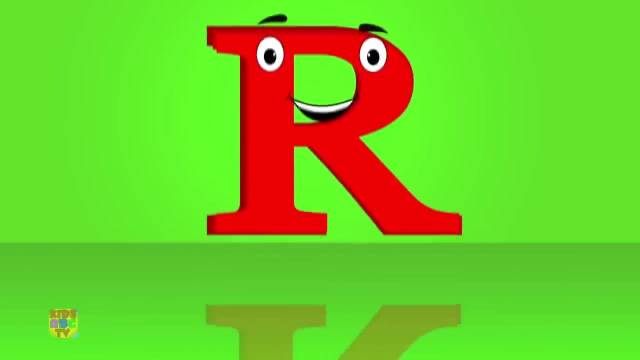 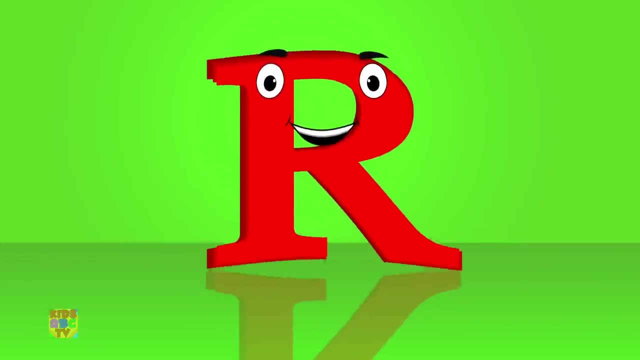 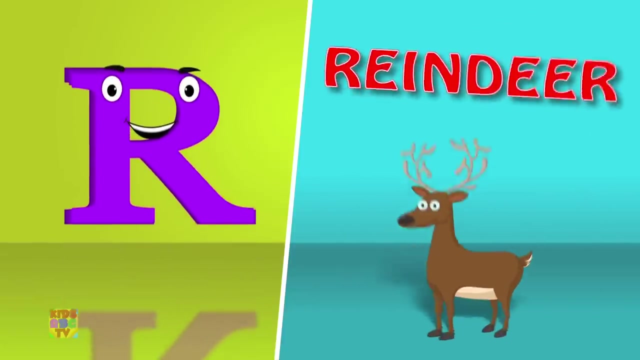 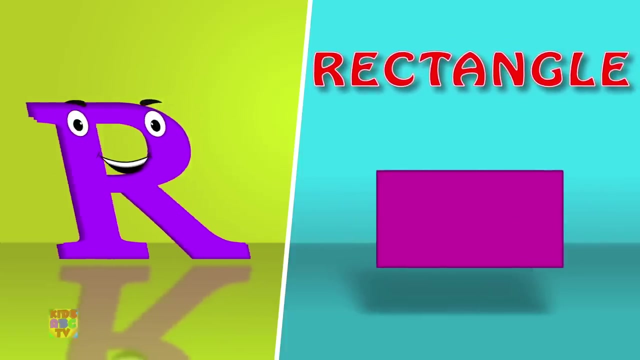 R is for Radish R R. Radish R is for Red R R. Red R is for Raincoat R R. Raincoat R is for Reindeer R R. Reindeer R is for Rectangle R R- Rectangle. 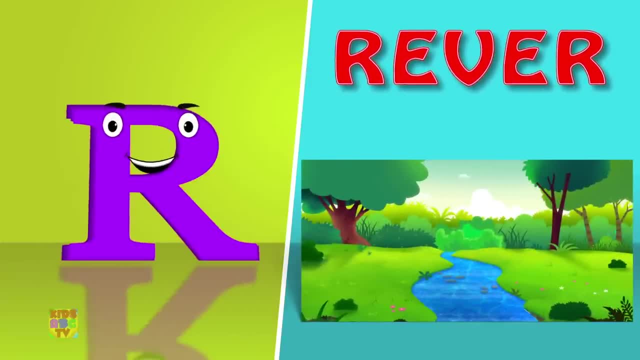 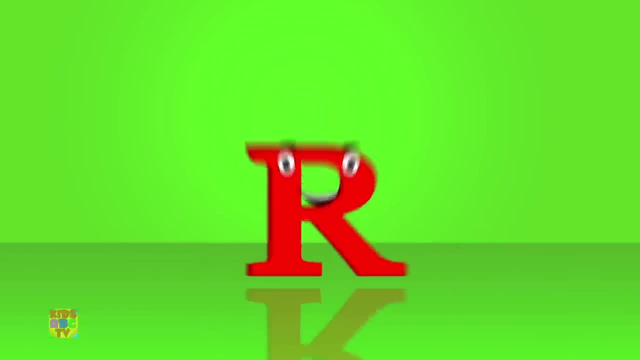 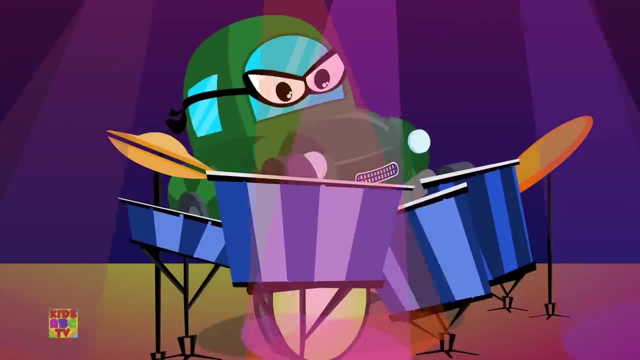 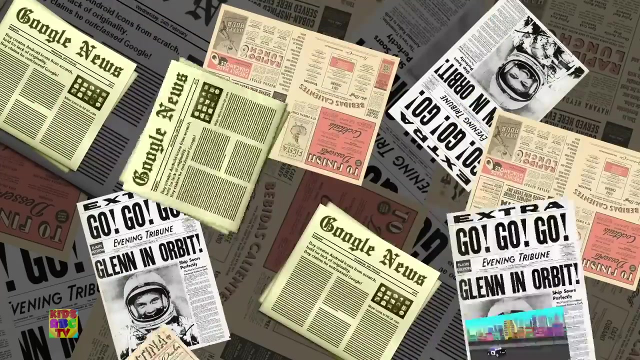 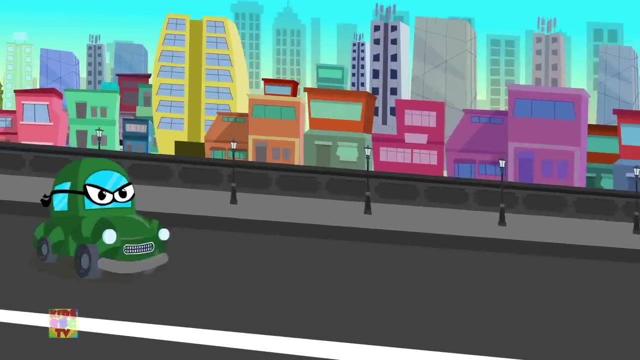 R is for River R R River. Hello, I am a police car. Come take a look at me now. I'm a police car. If I start to give chase, you bet The bad guys don't go very far. Come take a look at me now. 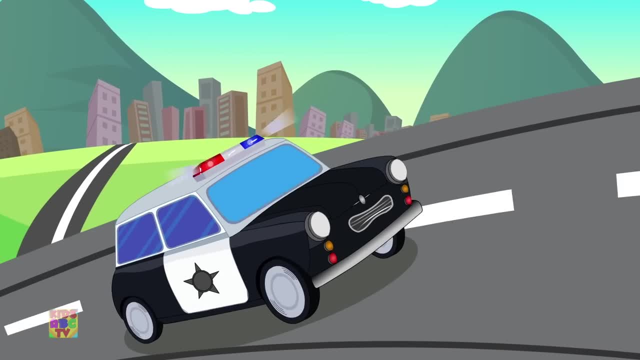 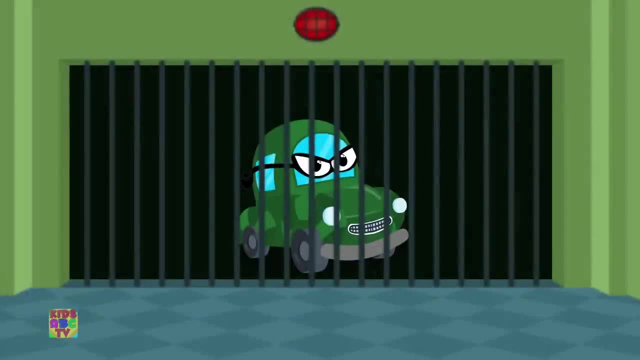 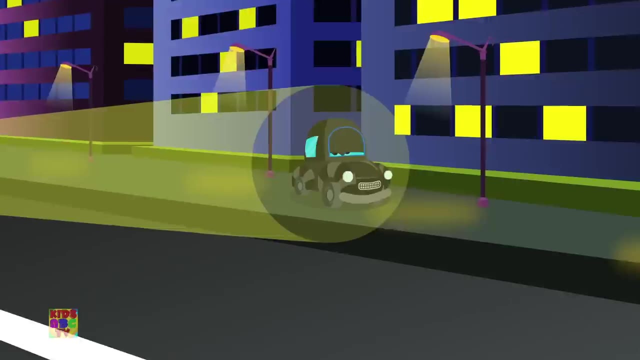 I'm a police car. If I start to give chase, you bet The bad guys don't go very far. The bad guys don't go very far. I go on patrols, Keep a lookout for criminals, And if I spot something suspicious I make sure to investigate, Cause that's my job. 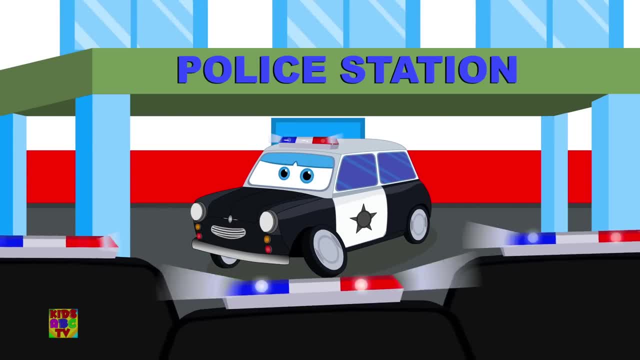 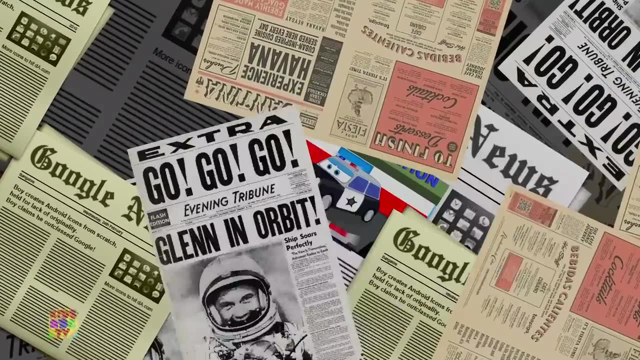 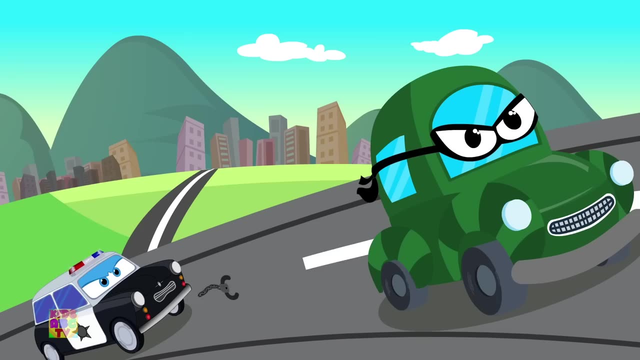 To keep people safe And keep the streets safe. I am a police car. Come take a look at me now. I'm a police car. If I start to give chase, you bet The bad guys don't go very far. Come take a look at me now. I'm a police car. 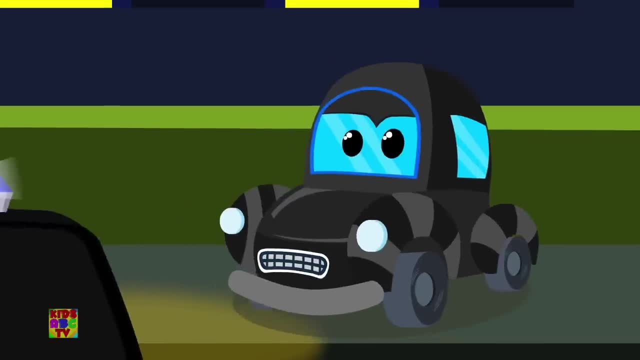 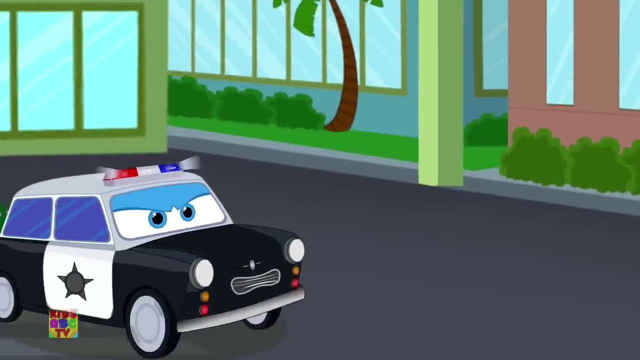 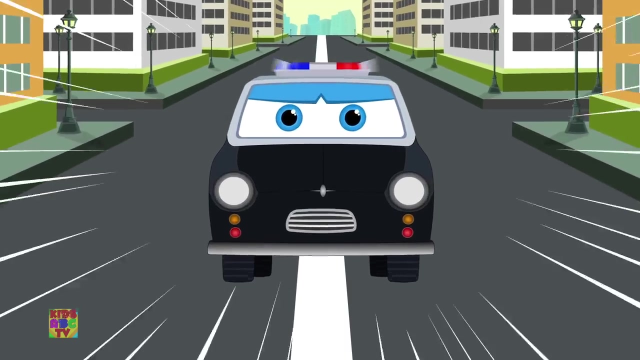 If I start to give chase, you bet The bad guys don't go very far. When there's an escape from prison- Ooh, that's so exciting. I need to track the runaway car And follow them at high speed. Of course there's my friends assisting me. 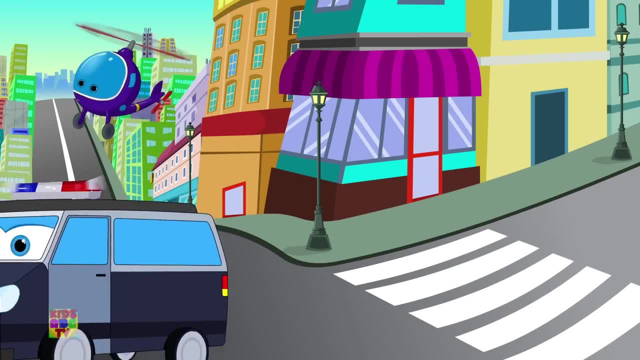 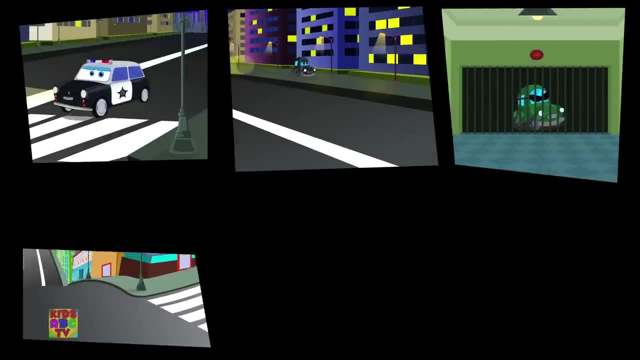 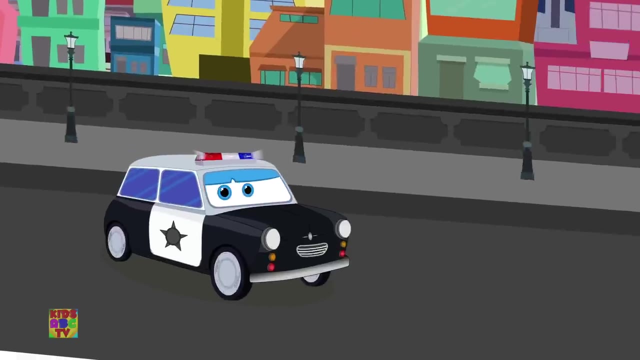 Like Mr Helicopter and the policeman, They do a real good job With their roadblocks and other cool gadgets. Come take a look at me now. I'm a police car. If I start to give chase, you bet The bad guys don't go very far. Come take a look at me now.